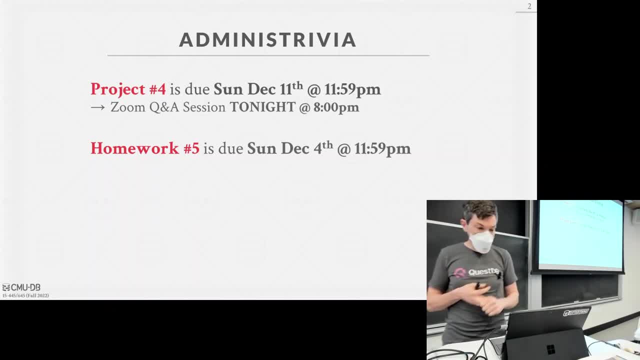 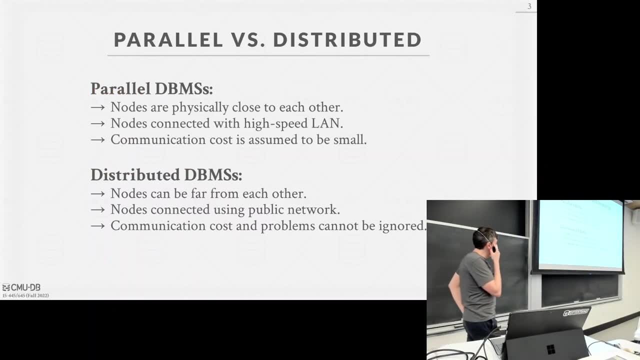 no one has gotten started yet. Okay, All right. So this part of the lecture opens up the new chapter of now talking about distributed databases And, as I said at the end of last class, we spent the entire semester so far just talking about how do you build a single node. 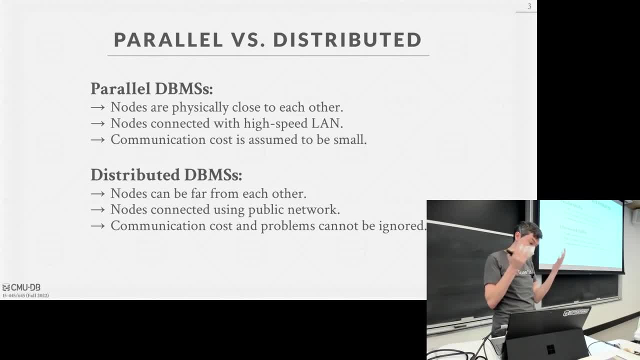 database And I didn't want to bring any. you know you don't want to bring in the distributed execution in because that opens up a whole other can of worms that complicates things. So now that we understand how does a single node database work, we can then extend the architecture. 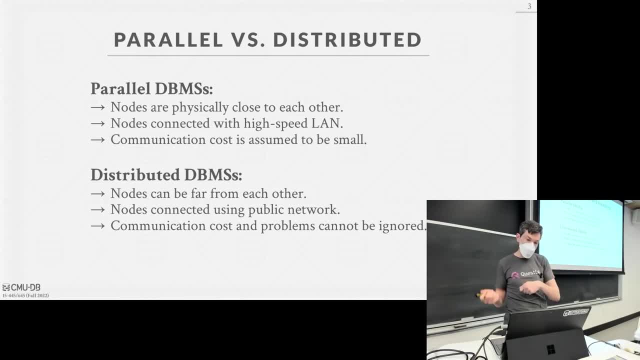 to now support a multi-node environment. So that's what this class and the next two classes will be about, And hopefully the main takeaway will be just from all this is that not only are single node databases hard, but they're even also harder if you make them distributed. 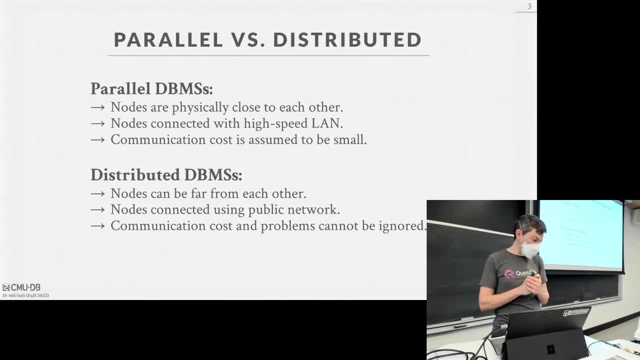 And so I would just say, oftentimes, people, oftentimes, you're better off trying to make your single node database scale vertically, meaning like getting better hardware and getting faster and faster as far as you can, before going distributed. Now replication complicates things and we'll cover that next class. So, if you recall, before the midterm we talked 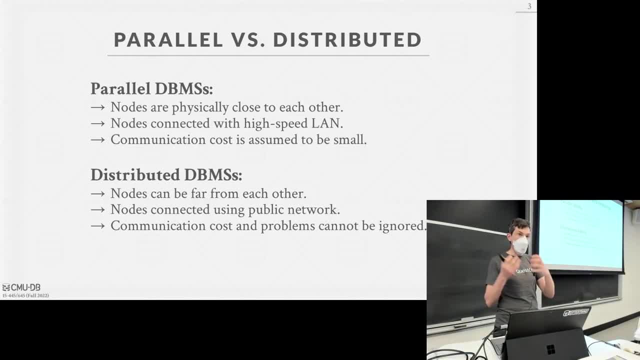 about parallel query execution, And that was about again on a single node. how do I take a single query and run it in? you break it up into smaller fragments and run that in parallel. Well, on multiple threads and multiple CPUs. And so we said this: we had this distinction. 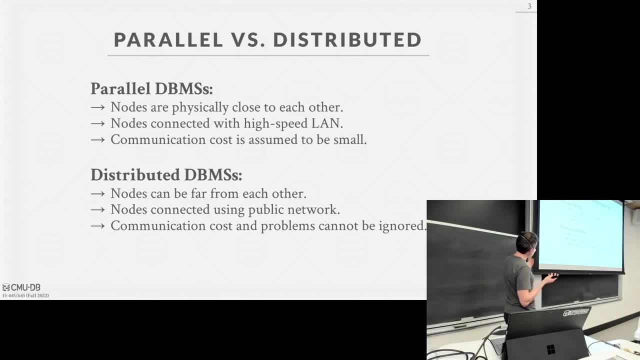 between the parallel database and distributed database, And my definition was: the parallel database is when the execution nodes are physically close to each other, could just be different CPUs on the same motherboard And we didn't worry about the communication costs or the communication being unreliable. But now, in a distributed system, all of that we can't. 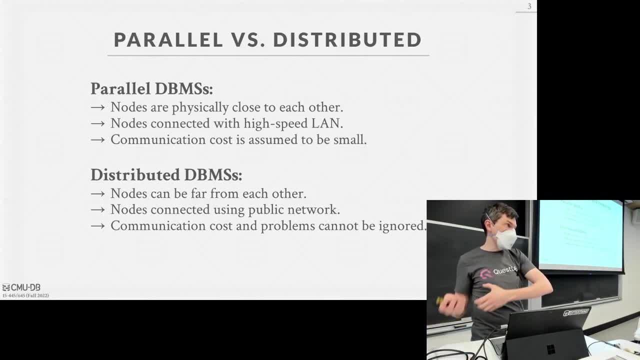 make that assumption anymore. Now the nodes could be physically far away from each other, Like if I send a message or I send a request from one node to another. it might be in the same rack. it might be in the same availability zone. 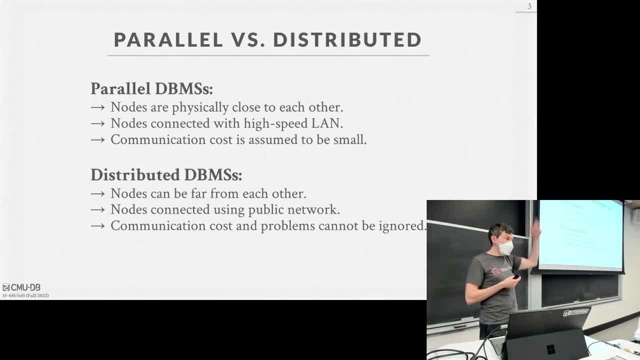 might be the same data center, or it could be in a data center on the other side of the planet, So we have to take that into consideration in how we design our algorithms and execute queries. So it also may be the case, too, that the messages 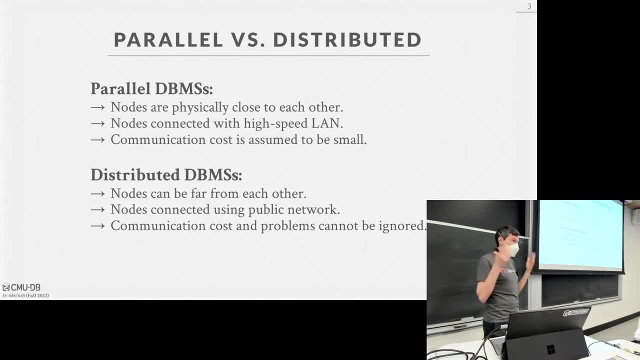 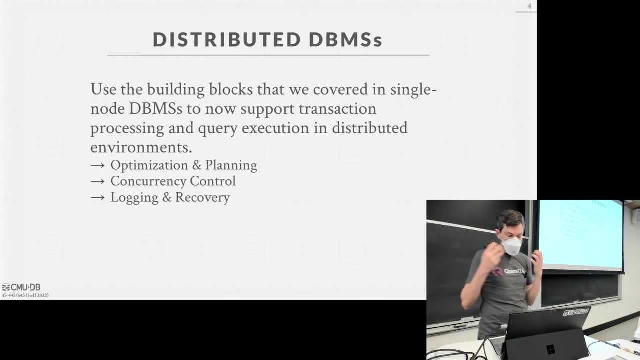 we're sending between the nodes may never show up. So we have to be aware of that and design for that That problem. So, as I said again for this point in the lecture, we're going to use the single node databases. we've covered so far as the building blocks to now support larger. 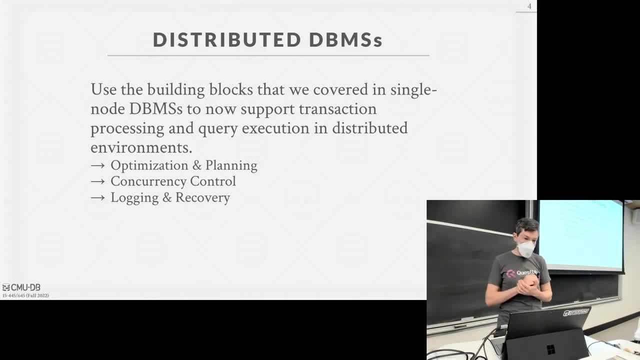 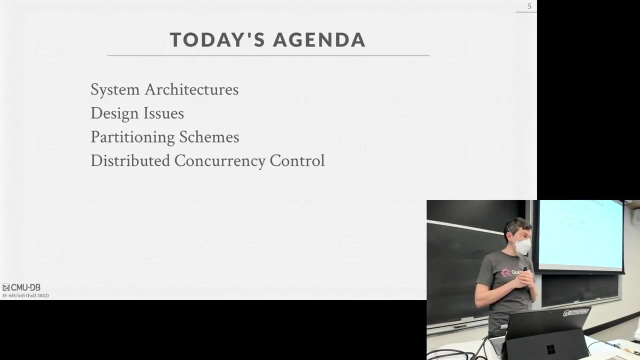 and larger systems And everything again just becomes more complicated, especially query optimization. That was hard. It's harder- Slightly harder, But concurrency is definitely harder and logging recovery is harder as well. So today we'll talk about beginning the different type of system architectures you could have. 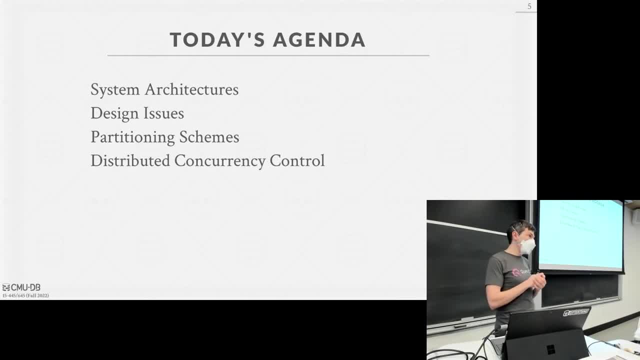 for a distributed database system At a high level. Then we'll talk about what are the things you have to consider when we actually build a distributed database. Then we'll talk about how we split things up, partition the data across multiple nodes, multiple resources, And then I'll give a teaser at the end of 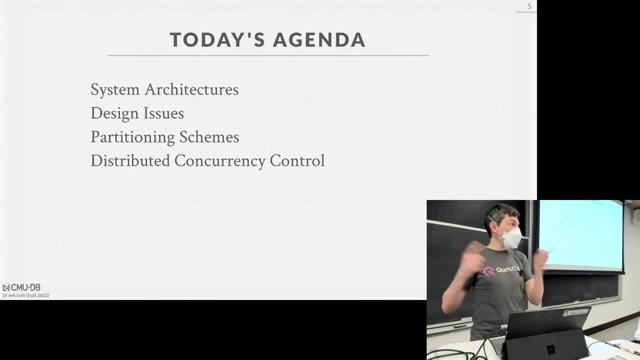 what the challenges are will be in distributed concurrency control, And that will be what we will focus on in next class. How do we take all that two-phase locking stuff that you guys can implement in project four OCC? how do we make that run across multiple nodes? 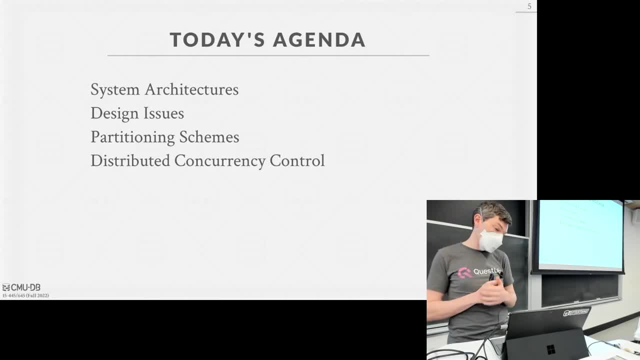 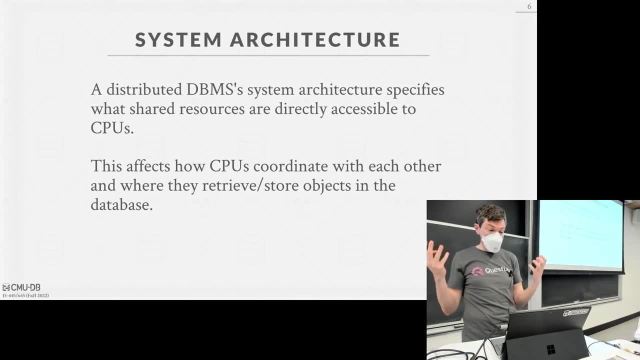 Again, and the spoiler is: it does, But it's slow and it's hard. All right, So the first thing we're going to figure out is: what does actually the system architecture look like? Meaning, how are we designing the database system in terms of? 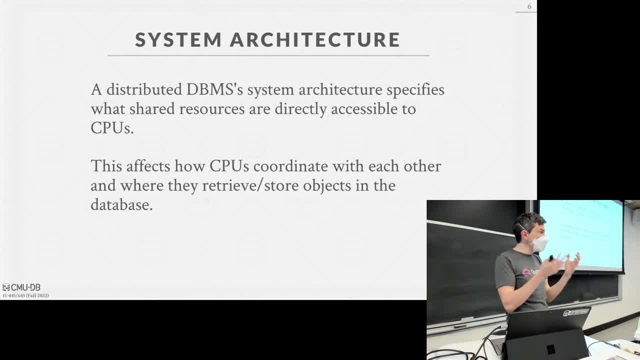 storage, memory and compute. Where are these resources actually physically located? And that's going to determine what kind of protocols or algorithms we can use when you run queries and run transactions. And it's also going to have an interesting side effect of that. It's going to have a 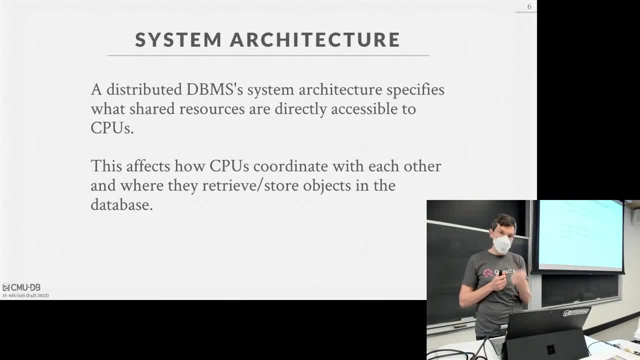 lot of different features. It's going to have a lot of different features. It's going to have a lot of different ways of determining how we're going to be able to scale our system elastically, meaning add more resources, add more nodes, If we were running on a single. 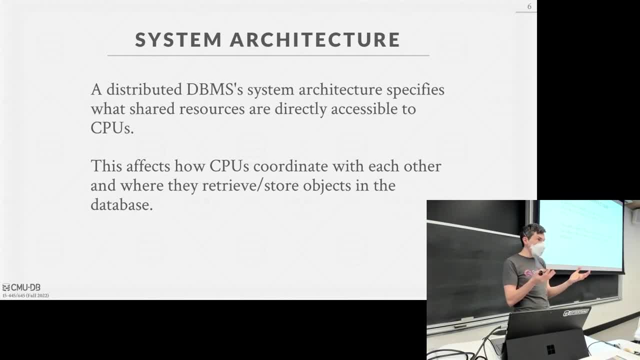 box, a single node system. if you want to add more CPUs, we literally have to turn the machine off and either migrate the database to another machine that has more CPUs or physically go put more CPUs into the motherboard. Disk is usually swappable. I don't think RAM is swappable. But now in a distributed environment, 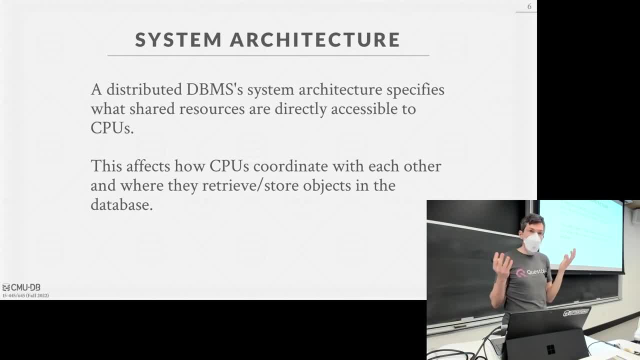 especially in the cloud. we're able to do that, And we're able to do that, And we're able to do that in the cloud in theory, that we can just add more nodes and scale it horizontally, And we want to be able to do this without having to take the database system down entirely. 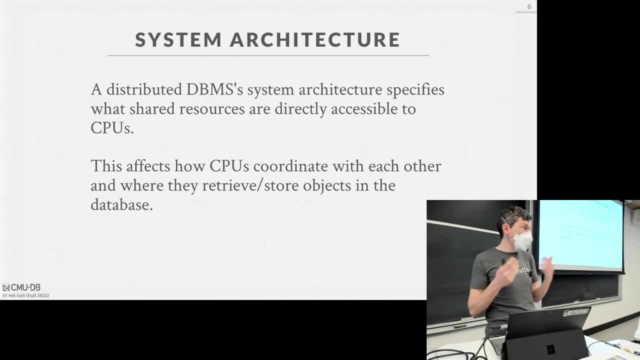 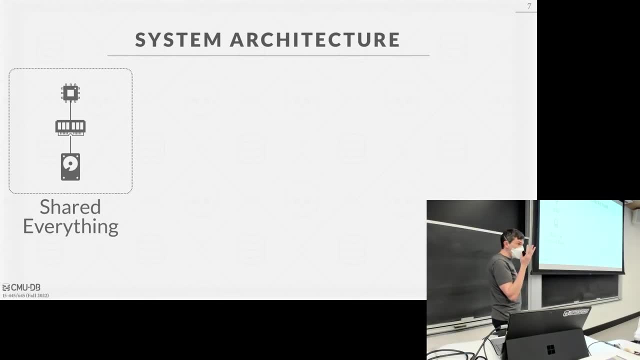 So what the system architecture is will determine what are the capabilities and how we actually would want to do this. So there's basically four types of database systems. We can import embedded databases. as I said before, Those are like a library you would link in, like SQLite, into your. 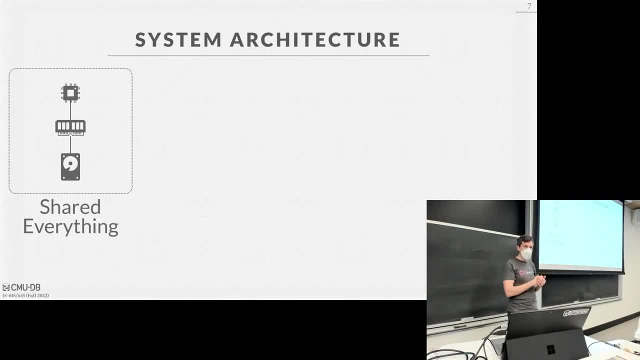 application And they're running in the same address space in the same process, So you're able to do this in the same process as your application And you could argue that those are basically shared everything. But for now we can ignore them, We don't care. 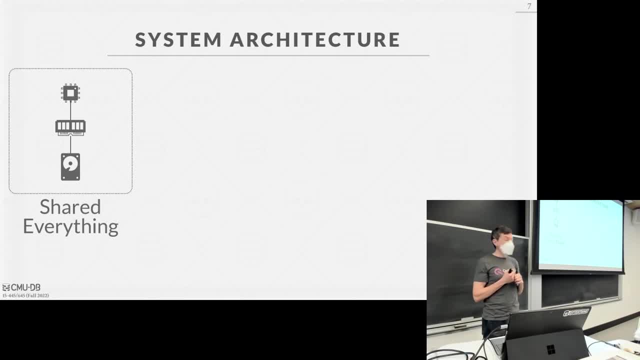 So everything we've talked about so far in this course are what are known as shared everything systems, meaning like the disk and the memory and the CPU are all local to each other, And if I want to have, say, two threads running or two queries running at the same time in 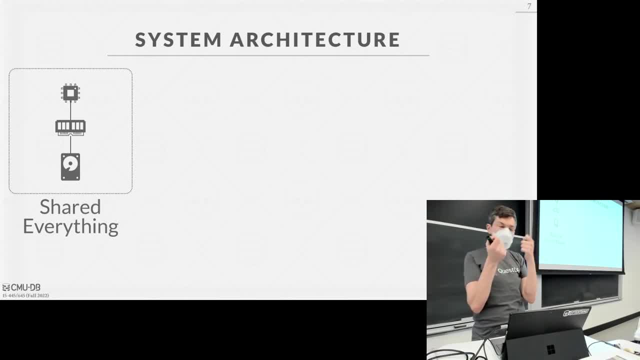 my shared everything system, then I can just pass memory- you know- messages to each other. And if I want to have, say, two threads running or two queries running at the same time in my shared everything system, then I can just pass memory- you know messages over memory. 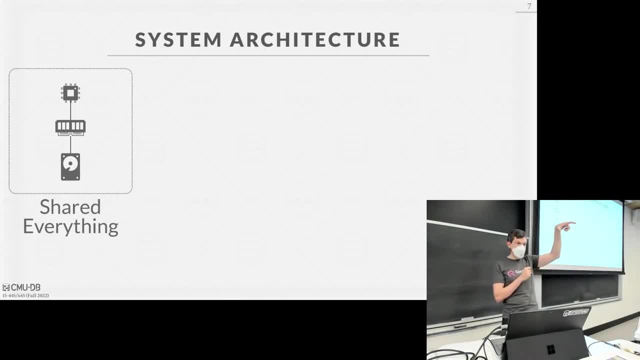 to each other And if I write any, if one transaction writes something to the local disk for the shared everything system, the other transaction can just read that right. The next type of architecture you have now, if you want to have it distributed, is called: 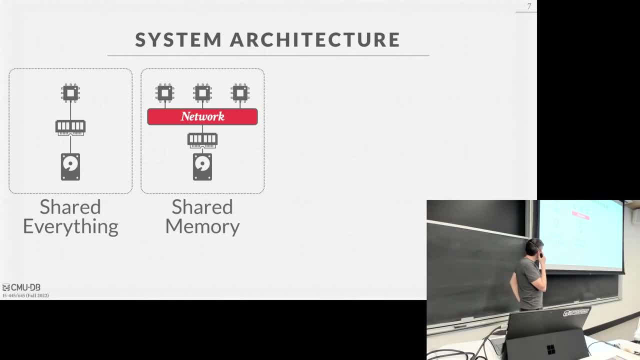 shared memory. The idea here is that the CPUs are not co-located, but there's some messaging fabric that allows the Some amount of memory to be shared amongst all of them, And then the disk, likewise, is also shared amongst all of them as well. So now I could have like think of this as 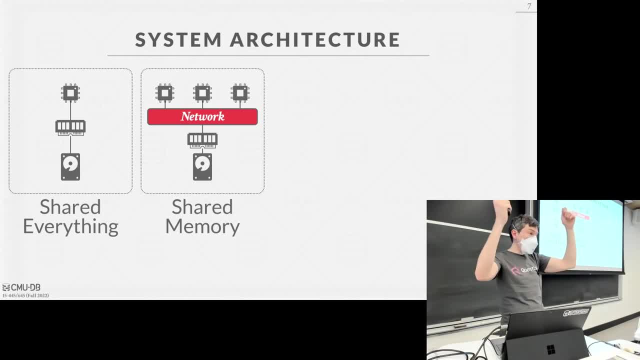 two boxes, and any time I want to have one thread running on one machine communicating with another machine. they could write to this memory address and then there's some hardware mechanism that's sending that message over the wire to the other node. RDMA is sort. 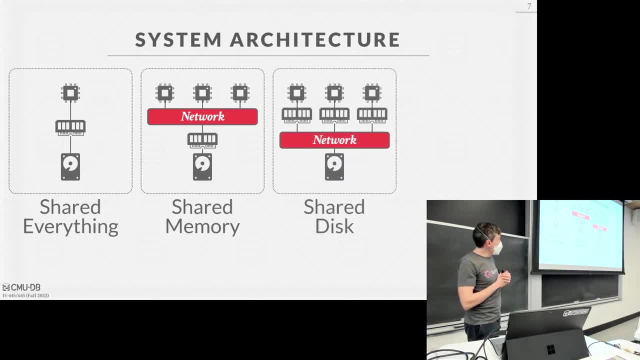 of something like this. What is more common in databases or the last two shared disk is when you have separate nodes that are going to have their own local CPUs and their own local memory, but then the disk will be shared amongst all of them. And again some messaging fabric, something. 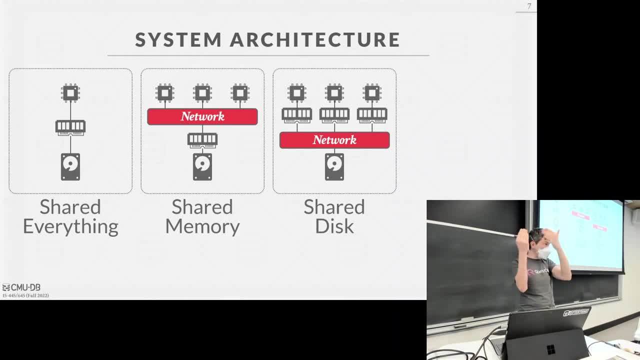 over the network that can take the request to from each of the different nodes and send them down to the disk. So again, if one CPU writes something to the disk, the other CPU could be able to see it when it goes and doesn't read. 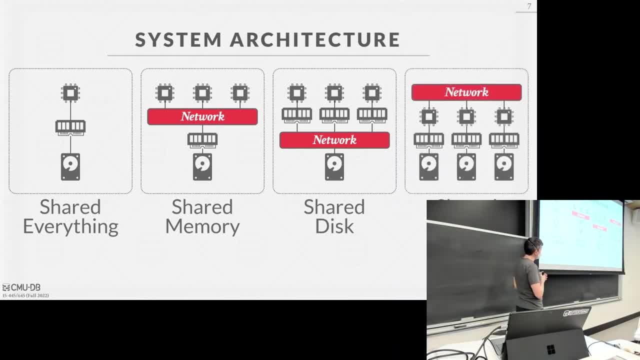 and then, when you think of distributed systems, this is oftentimes what most people think of what are known as a shared nothing system, where every single node is its own. it has its own local disk, local memory and local CPU and the only way to communicate between the different threads or different queries. 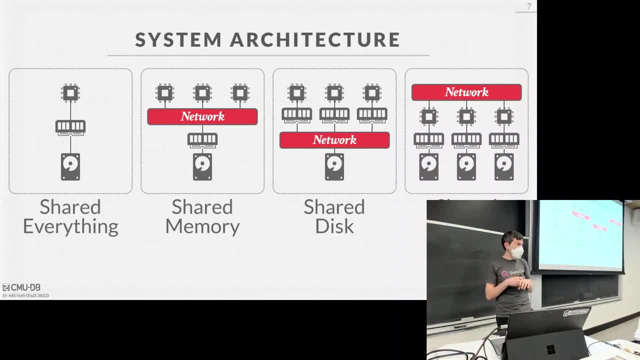 running on different nodes is to send a network message over TCP IP to pass it along to the different nodes, right? so think of like: I buy a whole machine, has, you know, disk memory and CPU, and I have multiple ones and each one is its own sort of kingdom. but they can communicate if they go over the network, right so you? 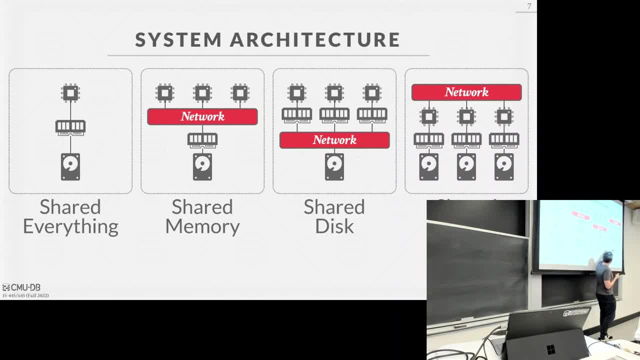 can sort of think of like I should have drawn borders, but like this is like its own node, this is zone node. this is no node. wherever the CPU is, that's, it has to be its own node, right? yes, this question is: do we assume that the network is reliable in the second and 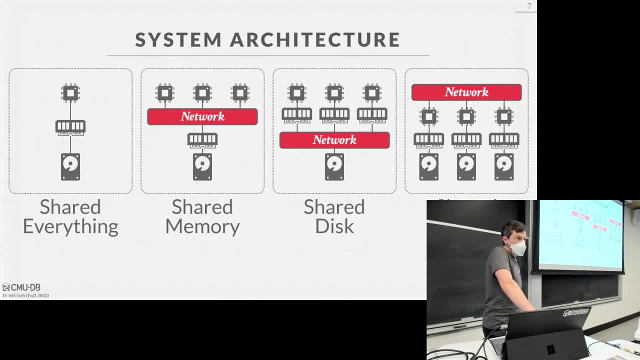 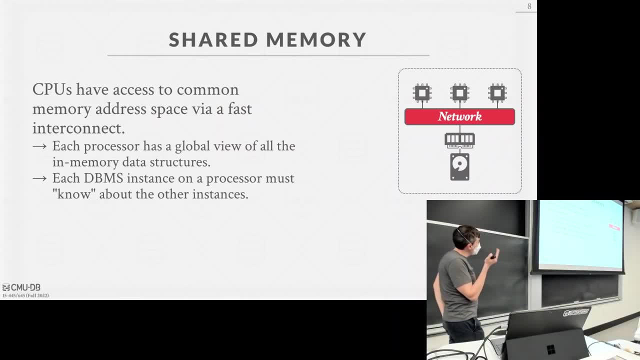 third case: no, okay, so do them, each one may want so. again in shared memory. again, CPUs are running on separate boxes but they have access to a common, common address space and it's soon to be a fast interconnect. does it not? guaranteed to be reliable, like is the other, the other node that you're writing the reading. 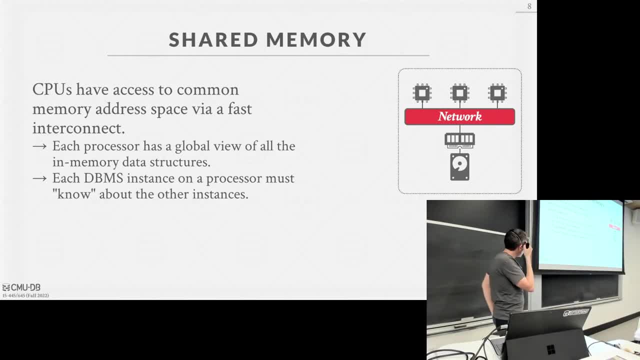 writing memory from could just go down and you have to deal with that. you right, but like. the idea is that, like, even though the CPU is maybe running on a separate boxes, they think or they believe that they have a global memory address space that they can all read and write to and so when they boot up, they 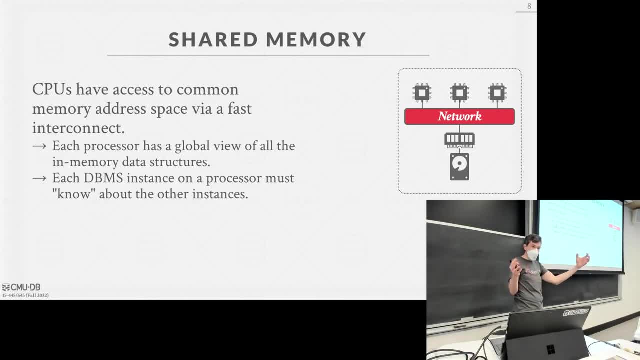 have to be told: hey, here's the other instances, there's something to tell me, here's what the giant memory pool is, and then hard work could keep track of how to pass messages around. so, as far as I know, there is no distributed a system that actually implements this. this architecture appears mostly in the HPC. 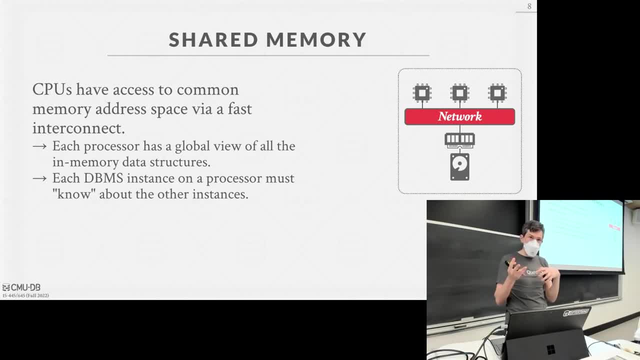 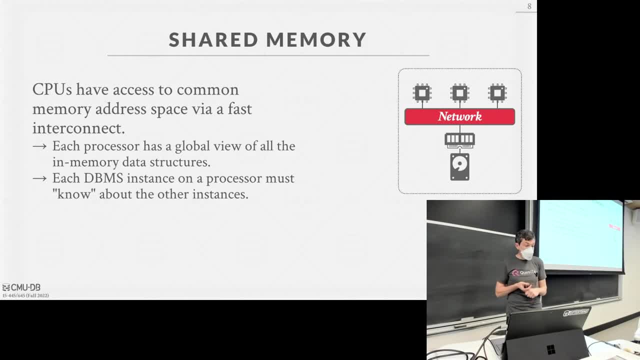 looks like this is Oracle Rack. the way that works is the buffer pool. you'd have sort of multiple nodes and the buffer pool has been modified so that the, when you read and write pages to it, it knows how to do send that requested to the different memory locations of the buffer pools on other nodes. so that's why I'm trying to get to that point. I'll see you guys in the next session. 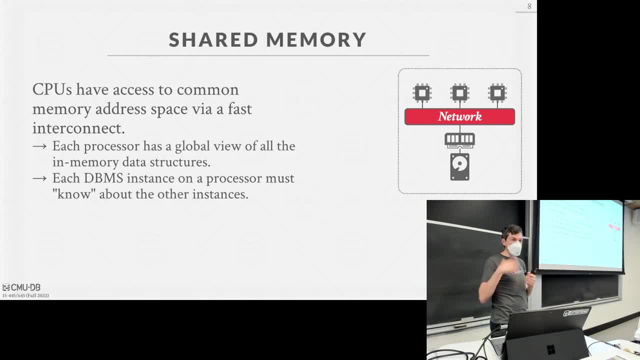 It's not exactly shared memory, because if I allocate memory for, like, a query to fill up a hash table when I'm doing a join, that's local memory and nobody else can see that It's only for whatever is backed by the buffer pool will be shared across multiple nodes. 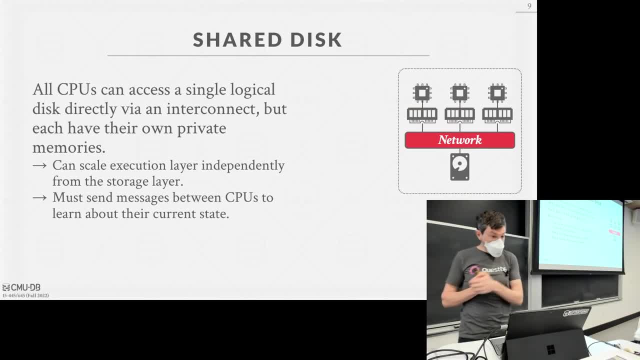 What is a lot more common is shared disk, especially in a modern cloud setting, And again, the idea here is that we have different nodes that each have their own CPU and local memory, But any time they need to read and write to disk, they're going to go to some central location. 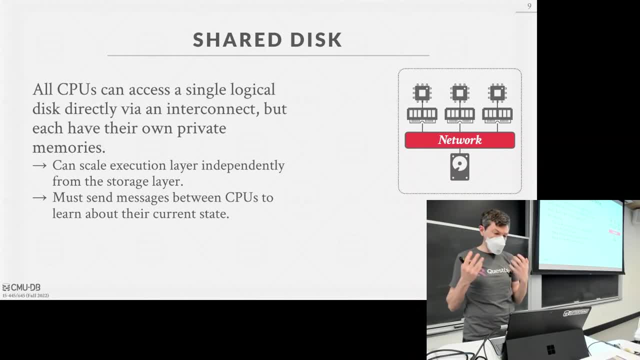 And if you're running on-prem, it could be like a NAS, like a network tax storage device. If you're running in the cloud, think of something like S3, right, And so if they need to get the state of the one CPU, needs to get the state of another CPU, like what query they're running, what transaction they're running. 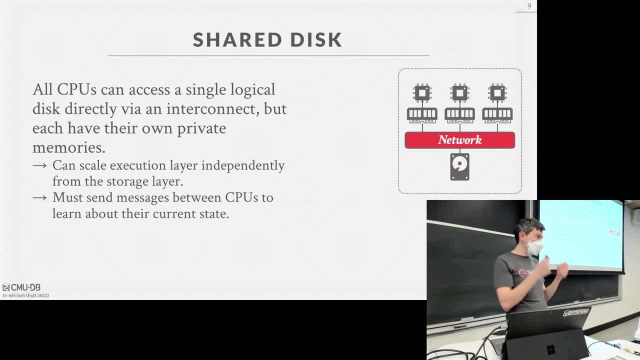 then they have to send messages over the network to like TCP IP between them. But again, if one query updates some record, that gets written out the disk. the other CPUs could be able to see that because they're always going to read and write from the same disk. 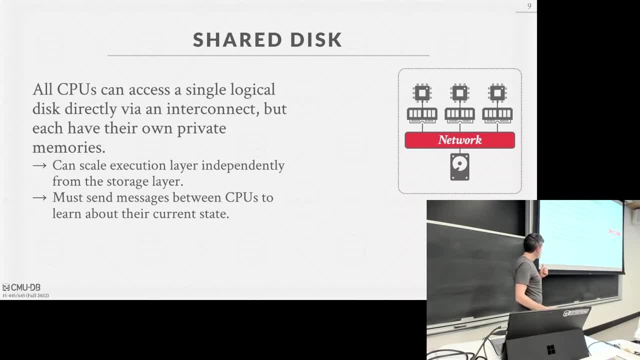 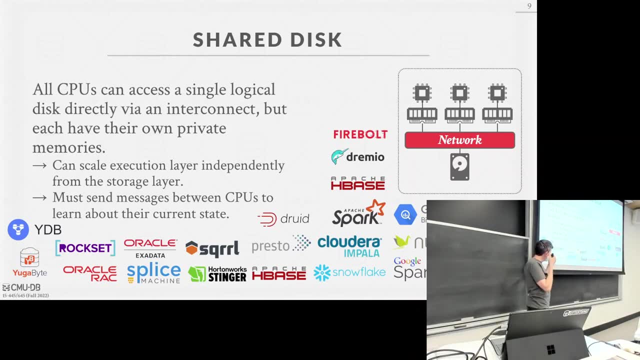 So this is super common now, especially in the cloud. So pretty much any modern OLAP system you think of today is going to be using this. Think of this again as like S3. There's a bunch of buckets. I could have a bunch of computers. 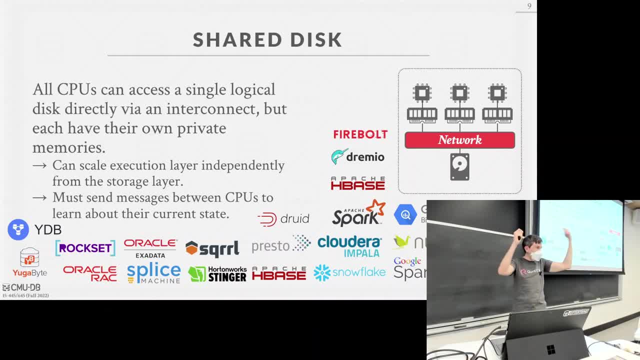 There's a bunch of compute nodes that are going to run queries and they're pulling data out of the S3 buckets into their local memory and then processing them to produce the query results. Yes, Would each page be stored as an object in S3, or would you store the entire? 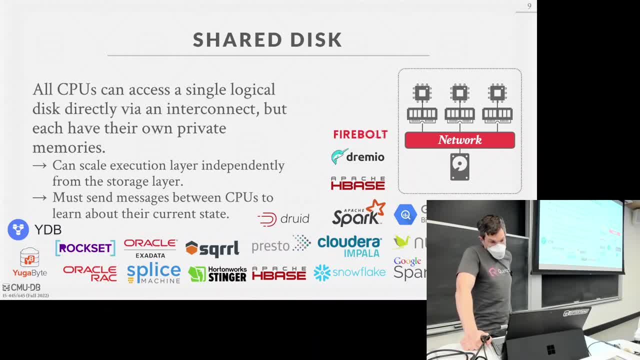 Because then if the entire database is just one blob, you kind of like just access the initial cases. So his question is: in case of S3, is each page its own blob or is the entire database? is the blob? Well, at this level you wouldn't necessarily call them pages. 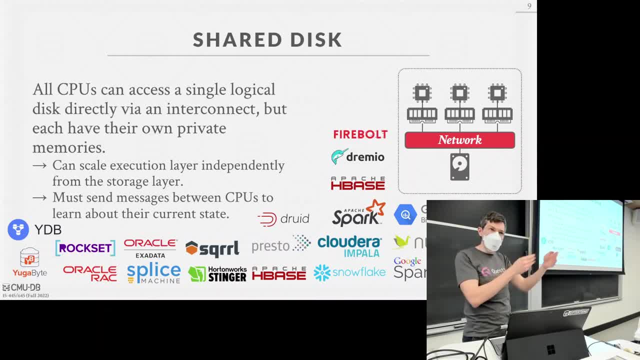 They might call them a higher-level segment that might be comprised of multiple pages. But the idea is that you'd go fetch that 10 megabyte chunk of data comprised of multiple pages and then run your query on that. Yep, The lines get kind of blurry because there are systems. 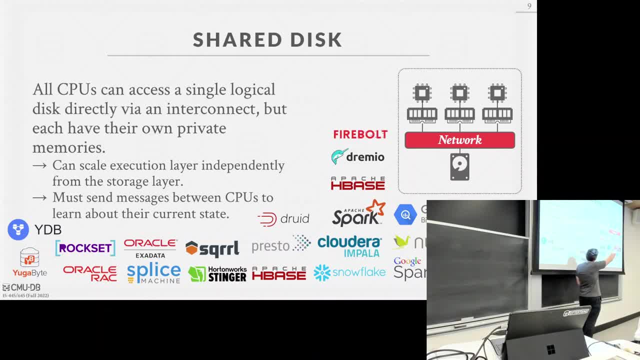 So yeah, the lines get blurry because again, this is like think of this thing, It's like it's its own EC2 instance, right, So you could have locally attached storage. But that locally attached storage could be used as a cache like a fast NVMe drive. 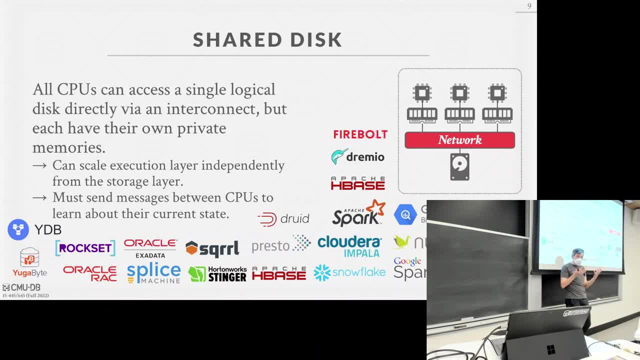 But the state of the database, like the final resting place of the database, has to be down on this shared disk storage here. So, as I said, this is pretty much every cloud system that exists now. today, for the most part, is using something like this. 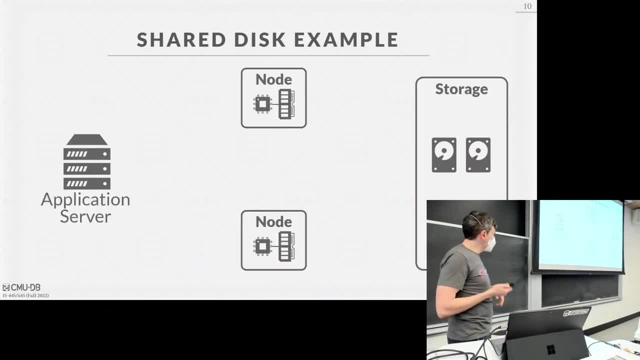 Yeah. So for example, how would it actually work? So you have your application server And so we have two nodes And then we have our storage, And then storage layer is like this own independent thing where again different nodes can read and write from it as needed. 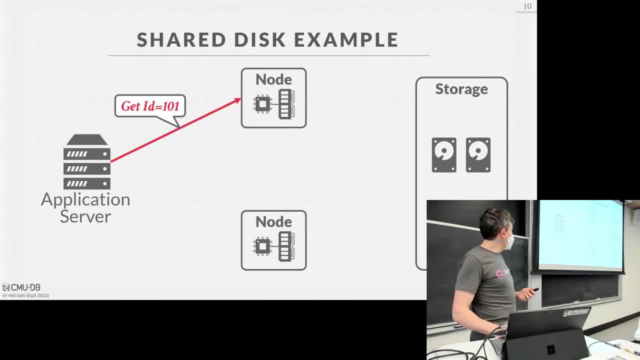 So my query starts. It says I want to get ID some object ID 101, like some record. So then it has to go down. I'm sorry It goes down here. It gets page ABC Again it's a single object or it could be a larger object. 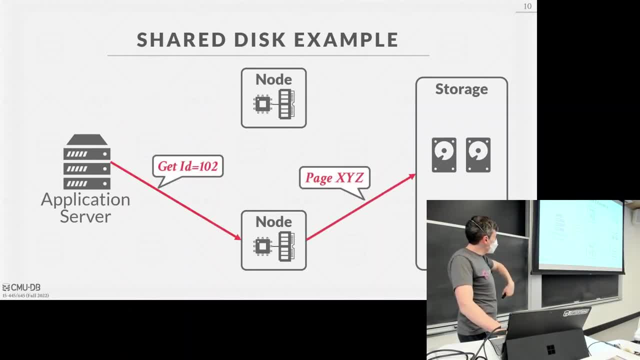 And I have to pull the page out of that. That gets shipped back over to the node and answers the result. This other query shows as long as I want ID 102. So it has to go to this node. How exactly do we find what node has the data we want? 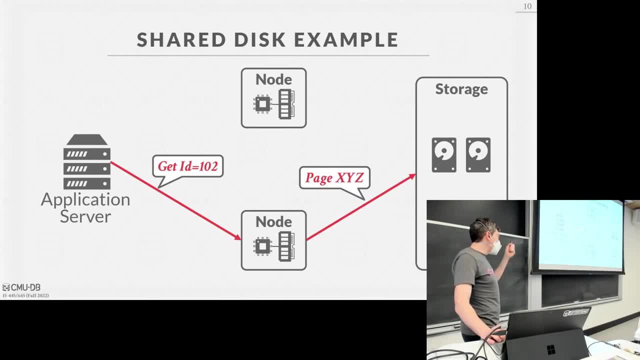 We'll talk about that in a second, But the idea is, again it goes back to the shared storage device and gets this All right. So now, the advantage of a shared disk architecture over a shared nothing architecture is that it makes it really easy to scale up with the compute layer and the storage layer independently of each other. 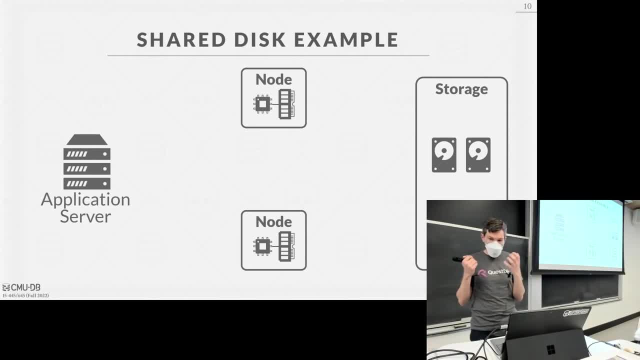 Because the final state of the database, like the state of the database that we want to persist forever after a crash and after stopping, is always out on the storage layer. So in theory, I could kill off these front-end nodes and I don't lose my database. 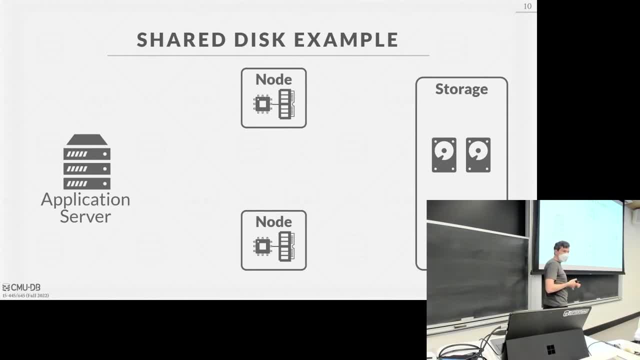 If you ever hear, like, when they talk about serverless architectures, that's sort of what they mean by this. So, like I can, Since this thing doesn't have Again disk, that's It's not storing anything on disk, that is the database that we have to persist forever. 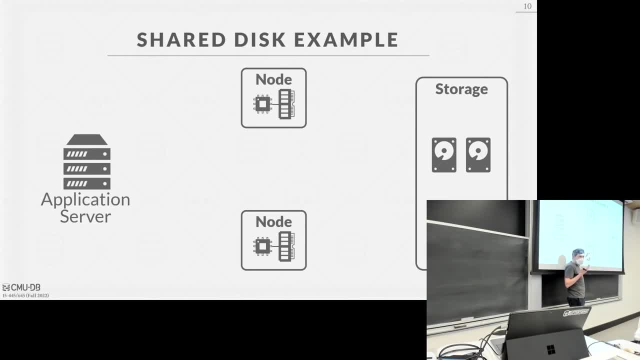 We can kill this node no big deal and then shut everything off. Amazon keeps maintaining my S3 storage And then if I want to run out of the query then I can spin this node back up and it can pull pages from the storage layer easily. 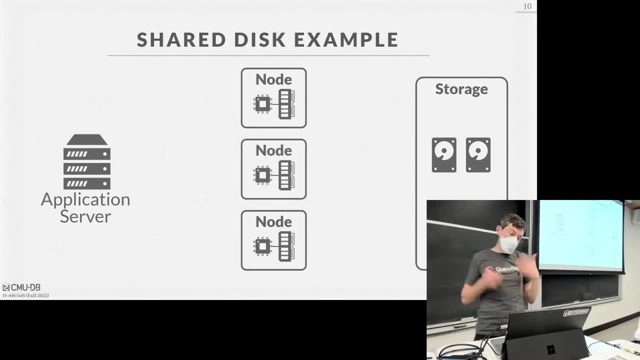 Or if I want to add more nodes without taking out the other ones. so I just pop this node up here And then now the query is going to. I can go to that and run the same kind of request and get results back. Likewise, in addition to scaling up the compute nodes, I can also scale up the storage nodes. 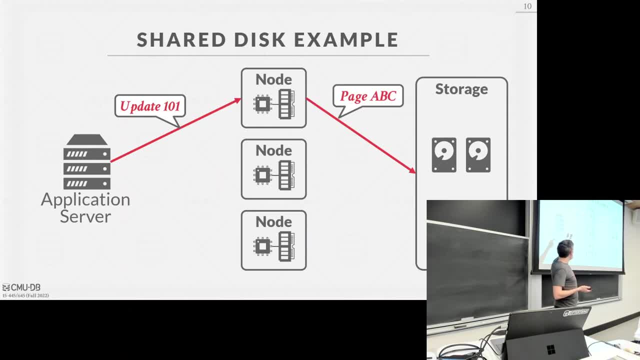 I will ignore this. Sorry, sorry, sorry. Yeah, so here I want to update. I want to update here Somehow- I know that this node up here at the top is responsible for the- For updating this record 101.. How we get there, how it knows to do that. we'll get there in a second. 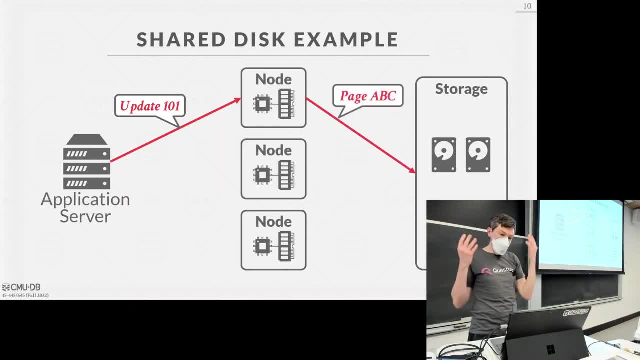 So in this case here I would go out to disk Update page ABC on S3.. That's fine, But let's say now that I also know that these other nodes have a cache copy of this record 101.. To make sure that they have the latest update, I can just send them a request over TCPIP. 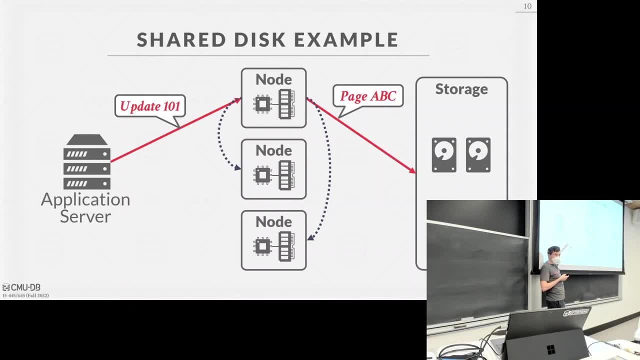 Say hey. by the way, I know you know something about record 101.. I just updated it. Here's the new value, Or you tell me to invalidate it, so then they'll go fetch it again from the storage device. Yes, 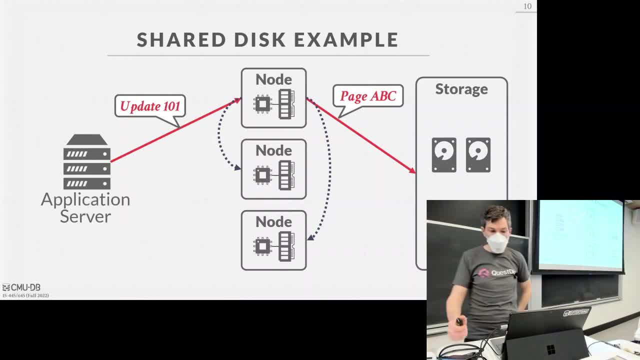 Like if you just direct this traffic always like, say, 101 always goes to node 1, 102 always goes to node 2.. Yes, You don't have to do this like thing, right? Yeah, so his statement is, and he's correct if I always make it so that 101 always goes to this node. 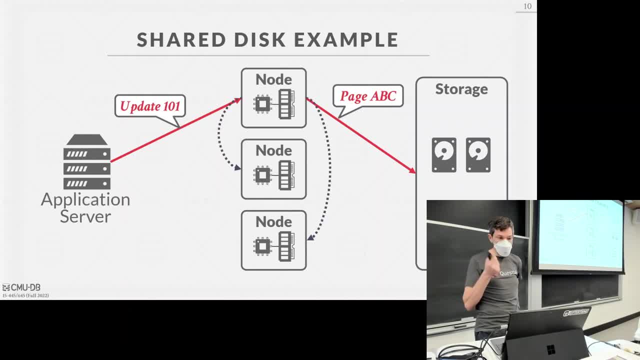 then I don't have to do this extra step of telling everybody to invalidate- Correct- Some systems do that. Other systems sometimes cache, Oh Yeah, Like a read-only copy, Because then otherwise you would have to do distributed transactions, which makes things harder. 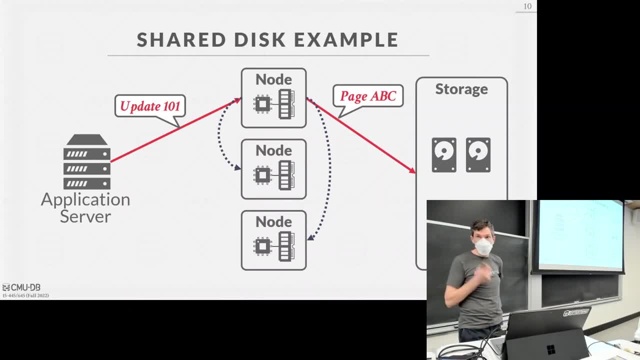 We'll get there in a second, But you're right, If you don't have another copy somewhere else, you don't have this problem, All right. So the thing I was going to say also too, in addition to being able to scale up the compute node independently of the storage layer. 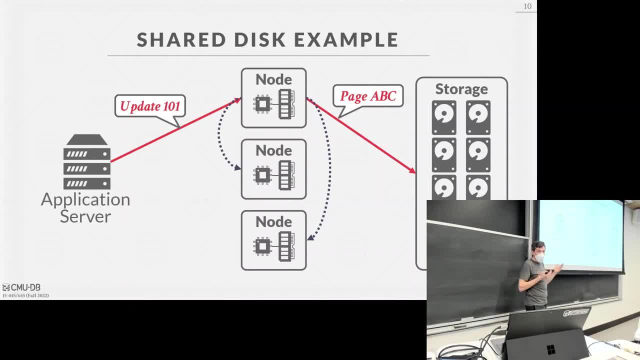 I can scale up the storage layer as well. Right, I can add more disks. I mean, Amazon will do this, They're going to do the covers for you. It's not something you tell S3 to do, But it can make multiple redundant copies. 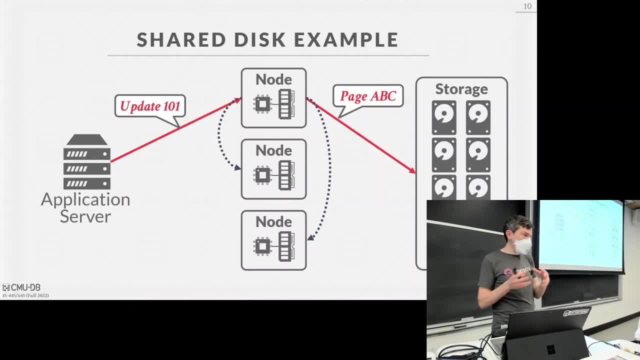 You can increase your provision. IOPs get better bandwidth. You can Make the storage layer be faster without again changing anything at the compute layer. Right, I'm using S3 as an example. Azure has their own thing, GCP has their own version S3.. 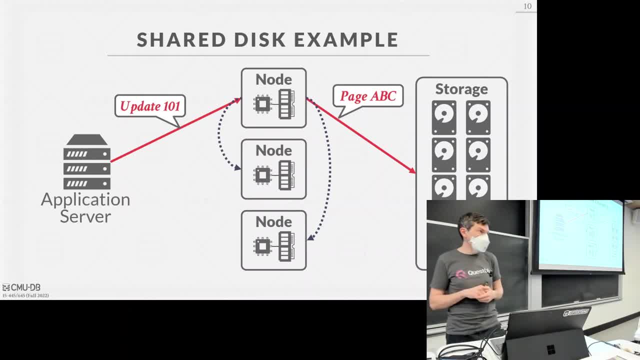 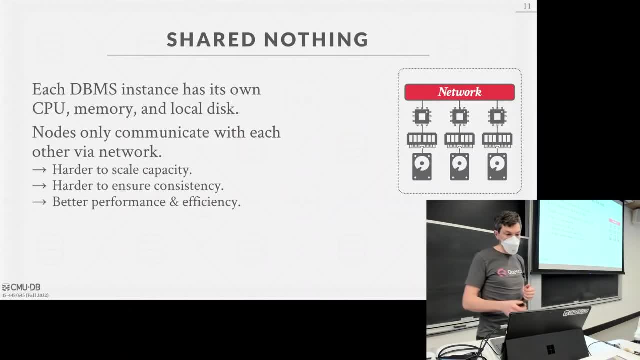 I forget what it's called All right, But the basic idea is the same. Right, It's like an object store I can do: reads and writes or puts and gets from and deletes- All right, So share nothing is as I was saying. it's where all the nodes are independent and have their own local disk and local memory. 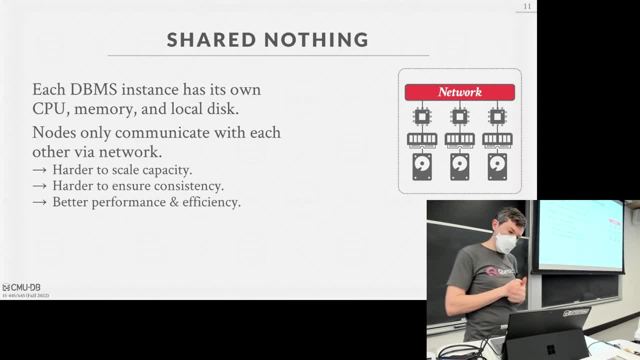 And historically, up until probably the last ten years, this has been the preferred or conventional wisdom, the right way to build a distributed database system. Right. There's a bunch of actually shared disk systems even before the cloud, going back to like the 1980s. 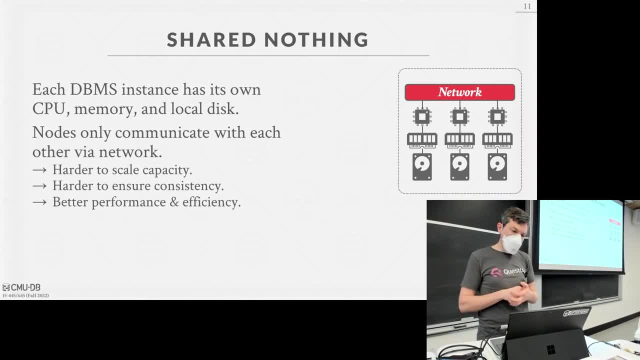 But these things are always sort of seen as problematic And a bunch of them, like the products, didn't go anywhere, And so everyone sort of said, okay, if you're going to build a distributed database, you would build a share nothing system. 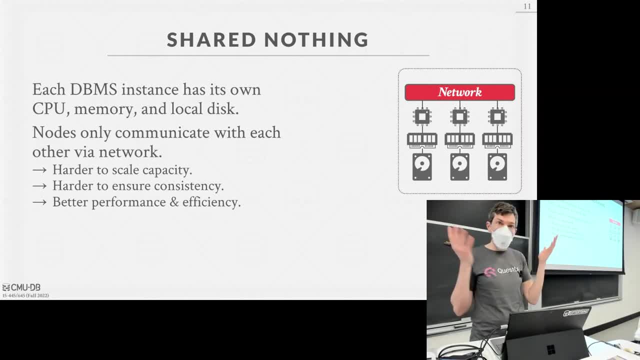 But now because of the cloud- You know Amazon Or whoever- the cloud takes care of the storage layer- It's just easier to build, better, to build a shared disk system, Again, because you can scale them independently. All right, 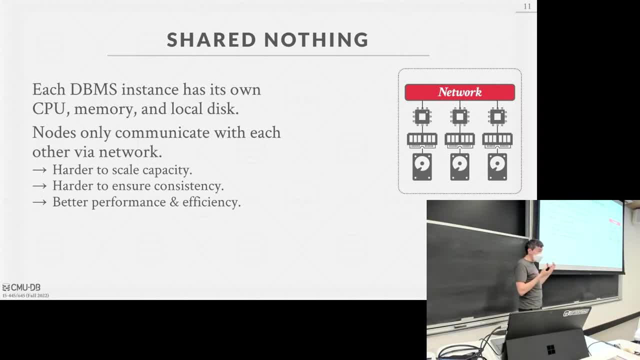 The basic idea is again with the share nothing system is that every node has their own locally attached disk and storage and memory And if I need to communicate between different nodes I just send messages over TCP IP. Yes, But isn't it like if you're using Amazon for a shared disk system? aren't you assuming- because, like I'm pretty sure, I'm behind the scenes? 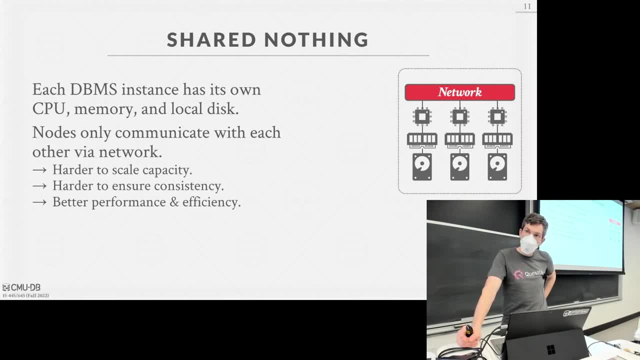 Amazon is doing their own like, own way of like doing a distributed like storage. Yes, So you're just kind of assuming that like they are going to manage it better than you do in that situation. Yes, 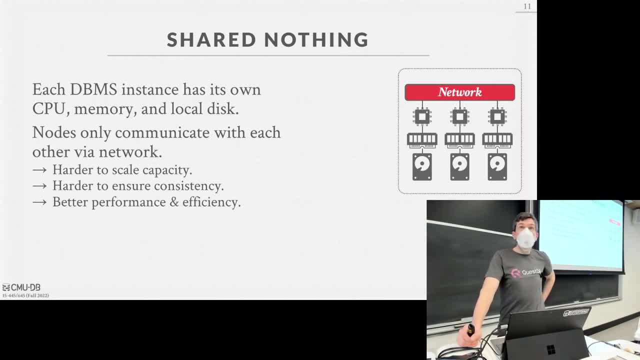 So the statement is: if you're using something S3, isn't Amazon managing the disk underneath the covers for you? Right Where I thought you were going to say it's also like replicating and all that stuff. Yes, And they're going to do a better job than you could. 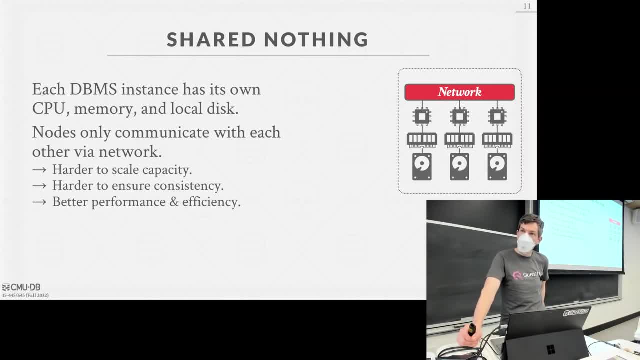 But like isn't. but don't we know that, Don't we know better about what kind of data we're storing, And then we can manage that better? It's kind of like: I see where you're going, Okay. 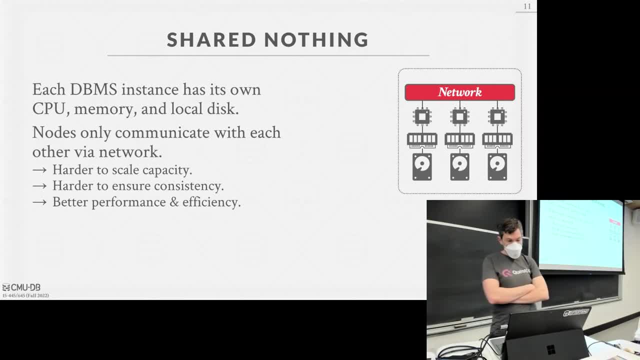 So your statement is that, like I made a big deal about how the OS doesn't know anything about your database and therefore don't let the OS manage things in your database. But now I'm saying, hey, if you use Amazon, you can use S3 and let them manage your things about. you know the storage, about your database. 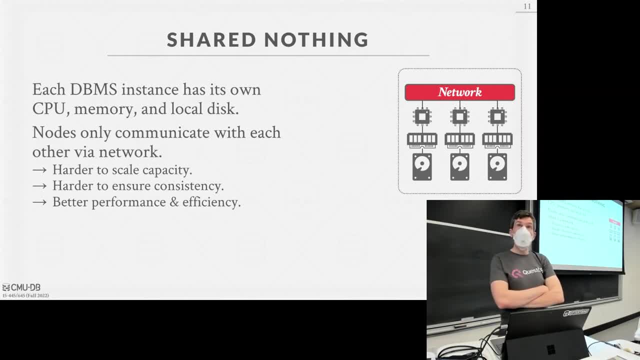 Right, Yes, You're right, And there would be optimizations we're not going to be able to do if we use S3, like predicate pushdown, Like we can't, Like we got to go fetch the entire blob of you know if we need a page. 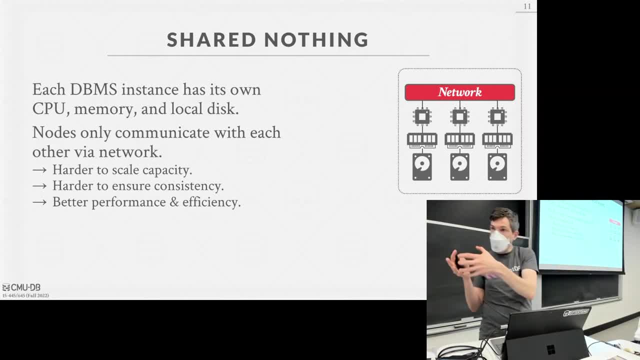 We can't do any like filtering where the data resides. We'll cover that topic in a second. Yes, The difference, I think, is, though, like: at that scale, Amazon is going to do much better, much cheaper, than you could yourself. 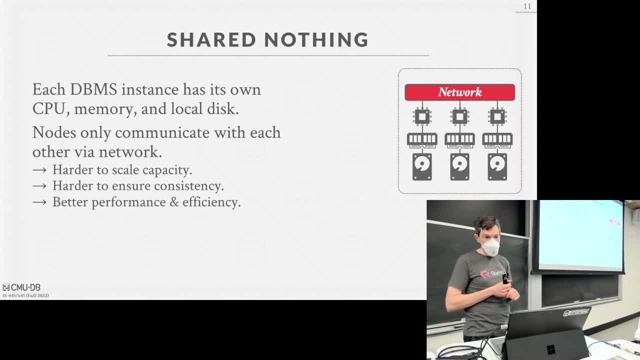 Right, It's just again like: S3 is pretty good, Right, It's slow. It's like 100 milliseconds, 100, 200 milliseconds per fetch- Right, That's a long time, And so you wouldn't want to use that for transactional workloads. 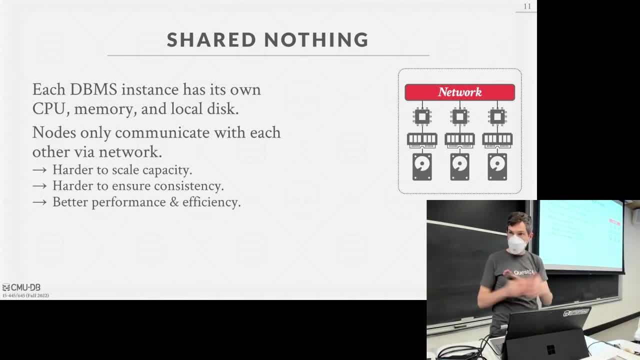 You could maintain that local cache on the node, as I mentioned. the local disk, Right, But if you want to be able to shut things down, you got to flush it out. the EBS or S3. OLAP systems will make more use of S3 because it's very, very cheap and affordable. 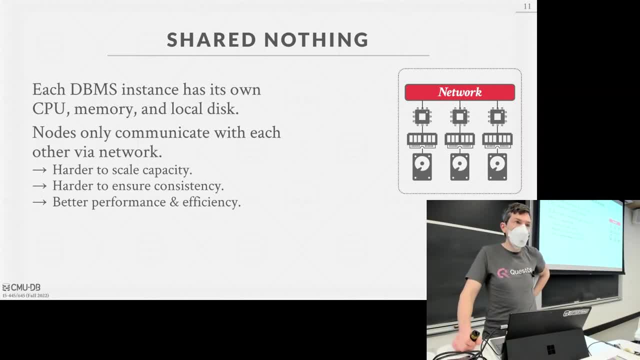 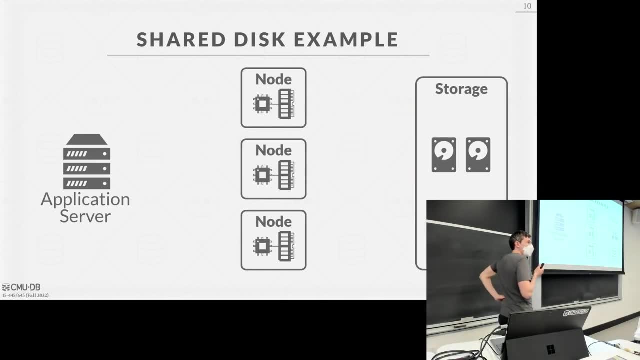 The other systems will use EBS. Yes, Yeah, I think it's interesting that like Aurora is also in the slide of like database and I guess they're using EBSes on S3? Yeah, So go back here. 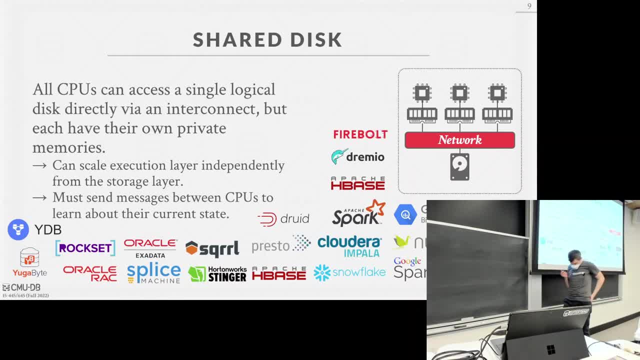 Yeah, Amazon Aurora is a very interesting one, So we can cover this at the end of the semester. But they- Amazon Aurora is basically- they took MySQL, they took Postgres, ripped up the bottom half of the storage layer, took the storage layer off and then rewrote them to be shared disk systems. 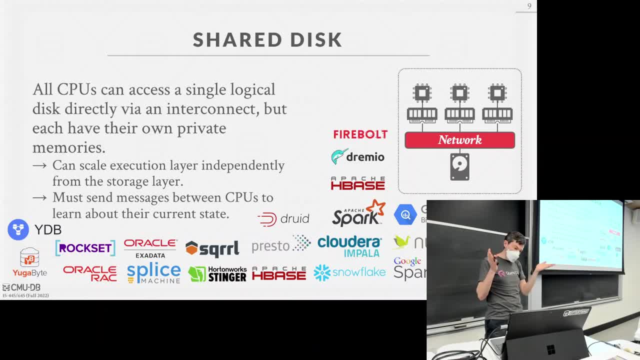 But instead of just storing things on S3 or using EBS, instead of just storing things on EBS like every other database vendor would normally do, since they control the whole stack, they actually put a little bit of database magic up above a layer, above EBS that knows about replication and transactions and durability. 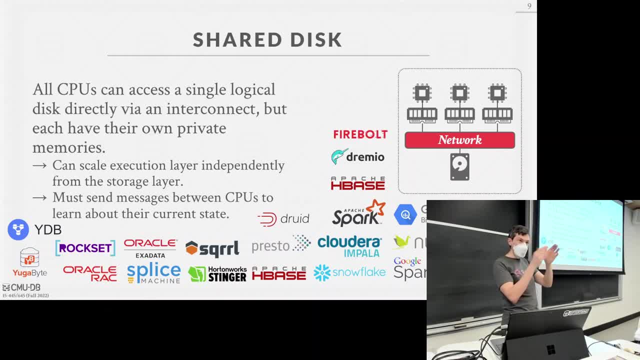 And so they can actually send messages at the storage layer between different nodes in a way that you and I can't, because we don't control EBS. Yeah, So Aurora is a special case where they- again, it's a shared disk system, but to his point, the disk layer isn't dumb just like getting set. 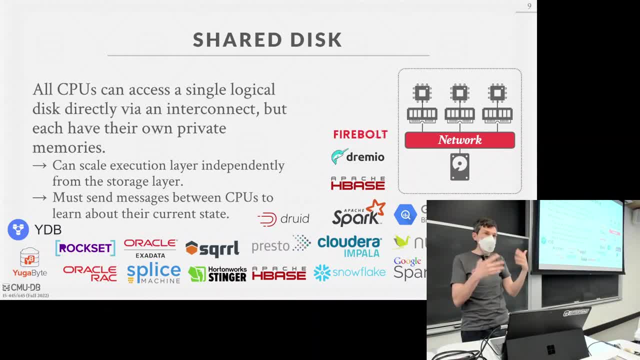 It's doing a bit more because it understands what transactions are and what the database is actually trying to do, And that's more efficient. when you can run like OOTB on top of it, That's more efficient for OOTB. yes. 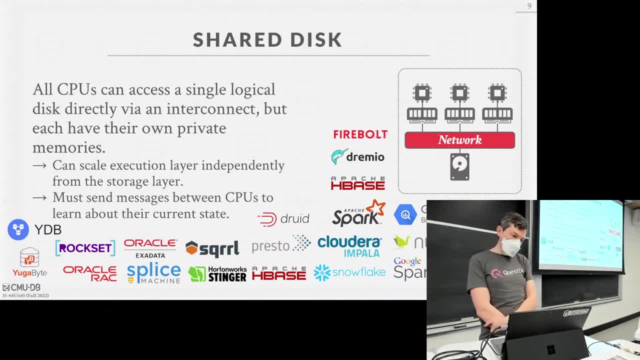 Yes, And there's other complications with shared disk as well, Like There's examples where people start off with a shared nothing system and they want to say, oh, I want to run it in the cloud, And so they want to run it in, like you know, a Kubernetes cluster. 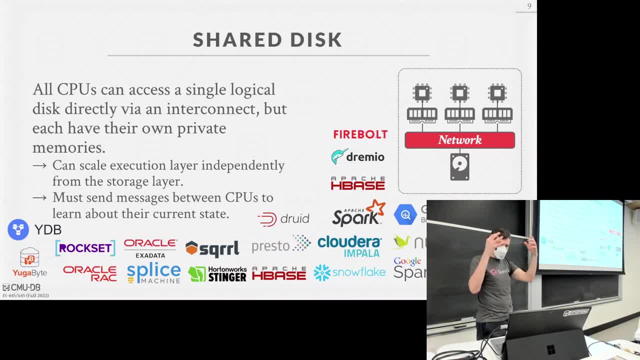 But like S3 is already replicating And then the system itself, the database system, is also replicating. So, like in Cassandra it used to be, if I do one update into Cassandra it would replicate that three times in the system. 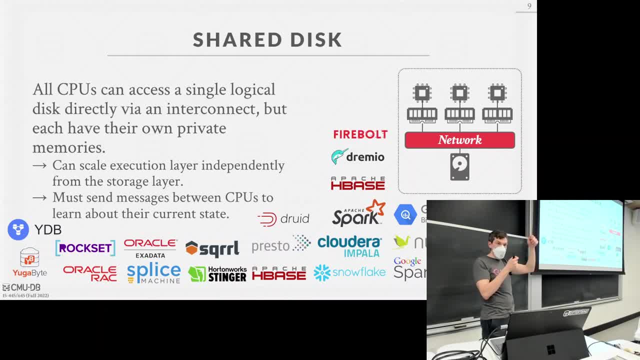 But then S3 would also replicate the write three times per node, So it would be like one write would get written nine times or something like some crazy number, Because again they're treating the disk as sort of a dumb object store that only does get and set and doesn't know anything about databases. 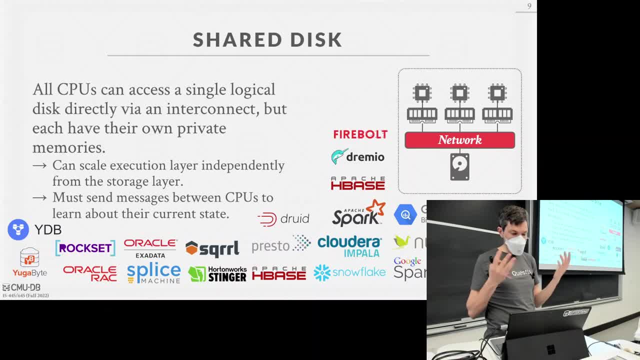 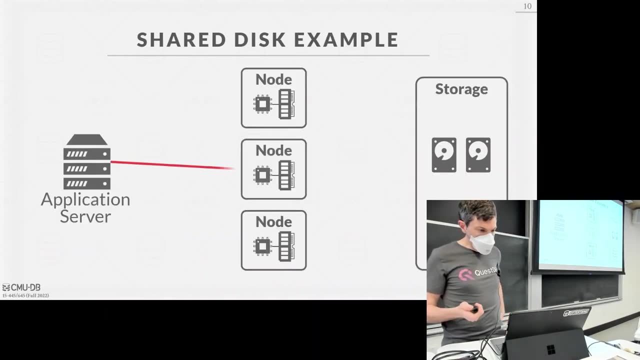 They've since solved that problem by just not replicating as much. But his point: yes, we're sacrificing quite a bit of things using shared disk, But the scalability and the cost difference is quite significant, So it's worth it Okay. 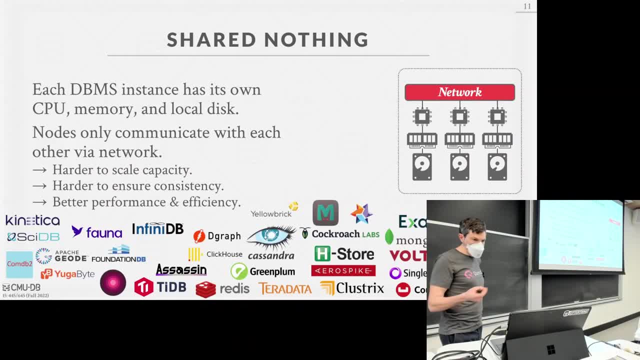 I think I've covered everything in shared nothing Right. But again here's a bunch of different systems that all do this Right Again, pretty much every distributed database written maybe before 2010 would do something like this. But then now in the cloud, everyone wants to do shared disk. 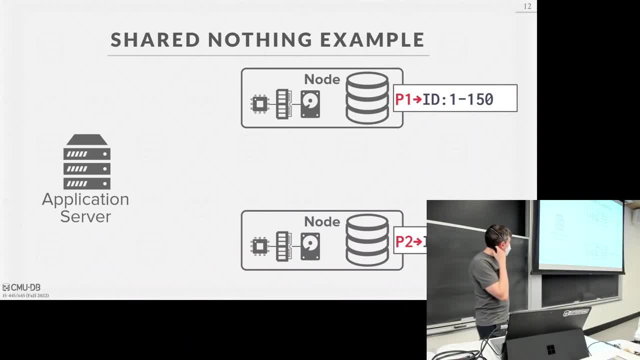 So an example would look like this: So now we don't have a shared disk, now Every node has its own disk, And then now I'm explicitly showing what data is actually storing. So we'll talk about partitioning in a second. But think of it like it's a way to take a table and we're going to split it up into separate, disjoint subsets. 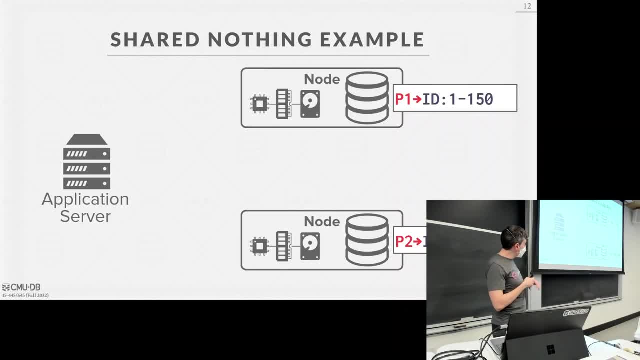 So node 1 at the top will have all the tuples for ID from 1 to 150. And the node at the bottom will have 151 to 300. So query shows up. It wants to get ID equals 200. Again, we'll cover in a second. how do we actually find where to go? 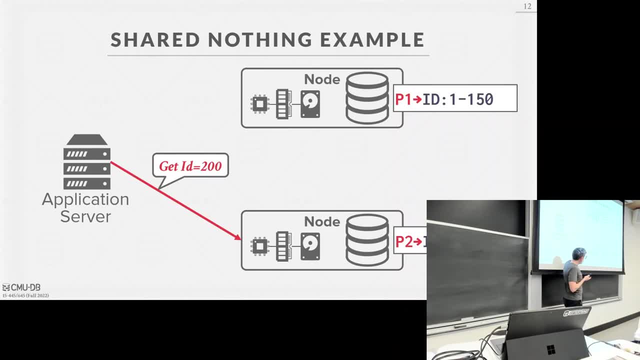 And then it knows that the data that it needs for this query is located here. So I don't need to coordinate with the other node here. I don't need to go out to a shared disk. Everything I need to run this query, Everything I need to run this query is local. 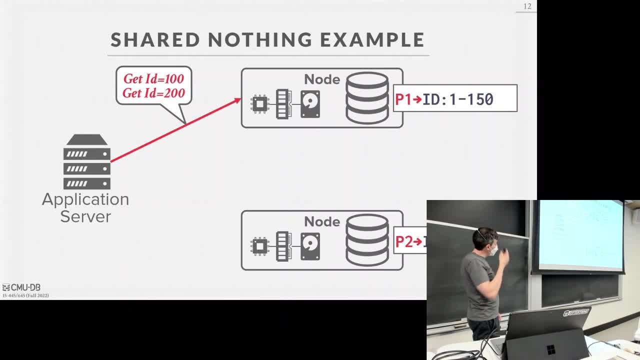 Likewise, this guy can go up here. He can say: I want 100 and 200.. Again, there's some metadata, a catalog where we're keeping track of what node has what data. So for ID 100, it could process this locally. 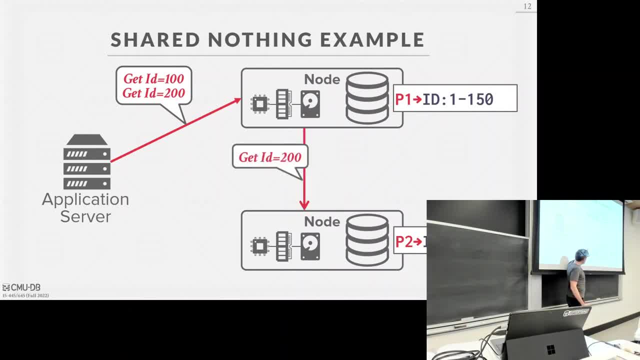 But for the ID equals 200, it could either go down here and say, hey, I know you have the record for ID equals 200. Send it up to me. Or it can say, hey, go run this query for me and then send me back the result. 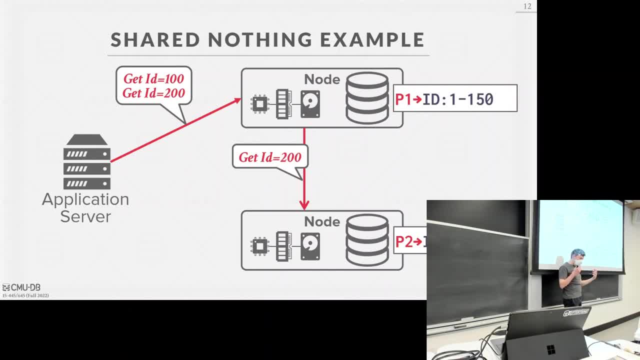 Because, again, we want to have the distribution of the data in the distributed database be transparent to the application. So ideally we don't want to have the application to know 100 is here and 200 is down here, Because it sends one SQL request to this one node. 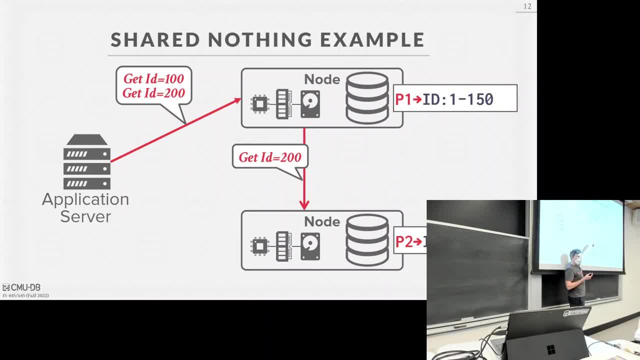 And then the nodes can figure out how to get the right result, get the result that it needs and send it back the single response. And we want to do this because every time we say a node goes down or we have to like rebalance or whatever, we don't want to have to go change anything in the application. 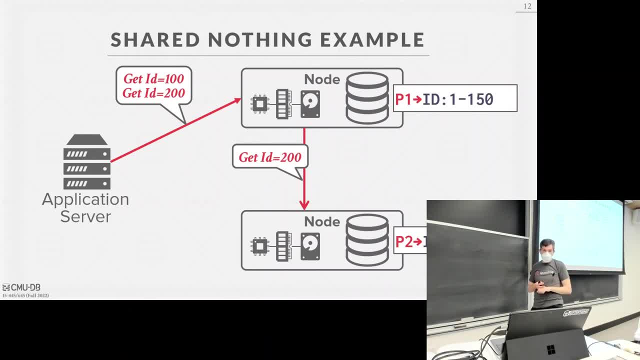 Everything should just work. It doesn't always work out that way, But ideally that's what we want, All right, So now the challenge with share nothing as opposed to share dis is when a new node shows up, or I take a node away. 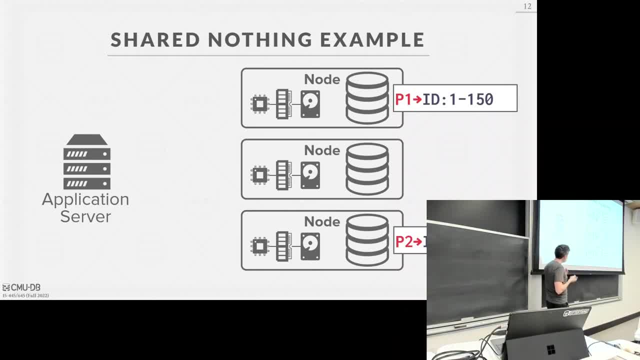 Right, Because when we initially boot it up, there's nothing inside of it, So we need to now shuffle around the data from the original two nodes that we had and put something in here. All right, So let's say we just split it up evenly. 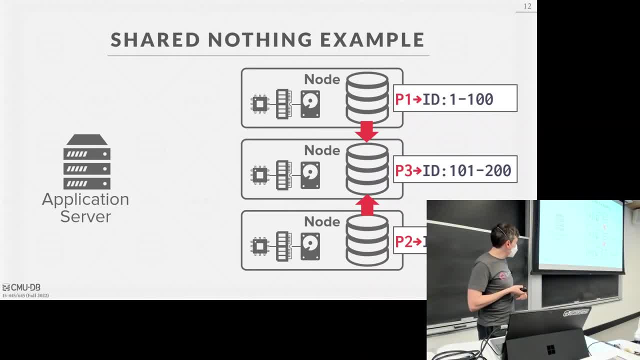 So the first guy has got 1 to 100.. He's got 1 to 1 to 200. And the last guy has got 2 to 1 to 300.. So this is hard to do because we want to do this safely. 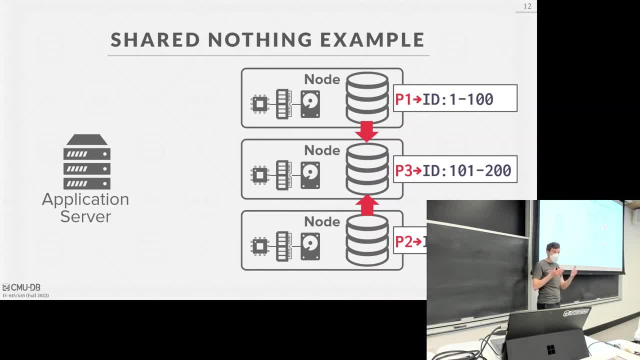 We want to do this transparently And we don't want to give. we don't want to have a small window where queries show up and you know it's looking for ID equals 150. But because we haven't probably initialized this node yet with all the data it shows up to the first. 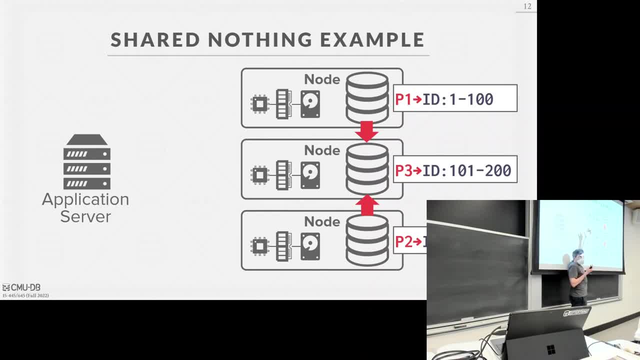 The query shows up to the first node and it says: I don't have what you need because it doesn't know about this guy yet. So you essentially need to do this migration in the context of a transaction And in shared disk. you don't have to do that. 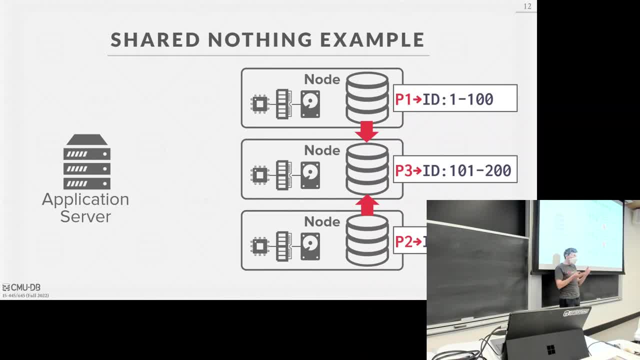 You don't have to physically move data. You just update logical information to say the data you're looking for is this compute node or that compute node. In a share nothing system it's physically moving data, which can be expensive. So I would say this is actually sometimes called autoscaling. 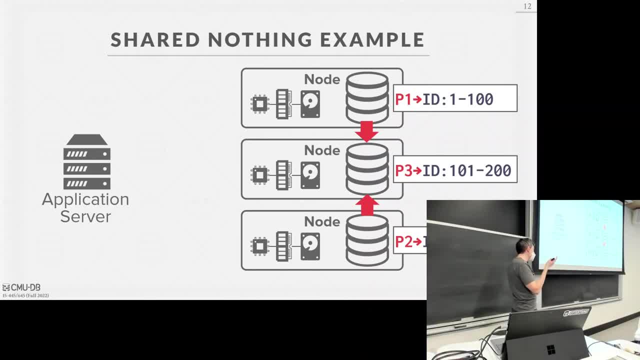 Or elasticity. This is actually one of the major selling points. This idea of repartitioning and reconfiguring your data was actually one of the major selling points of MongoDB back in the day. I think they still support it, But they wouldn't do it actually in the context of transactions, because the early versions of MongoDB didn't have transactions. 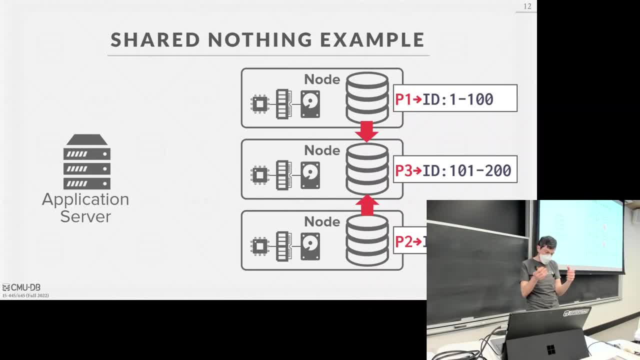 So like what would happen is, you would have these partition nodes, You would add a new node and try to rebalance, But there could be a smaller node, There could be a small window. If your query showed up, it would say: you know, give you a false, negative. 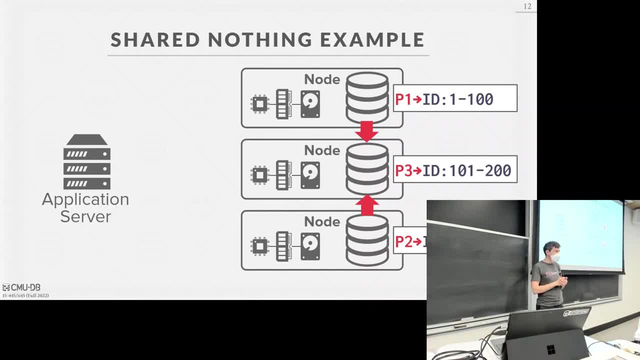 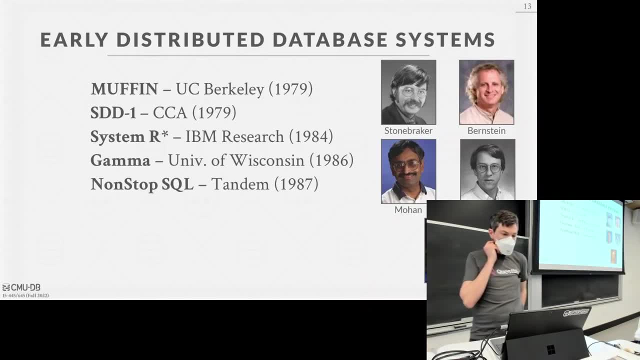 Say you didn't have data that you actually had because it was updating things and moving things around Right Again. so this is not easy to do. All right. So distributed databases are not new. They go back to the 1970s. 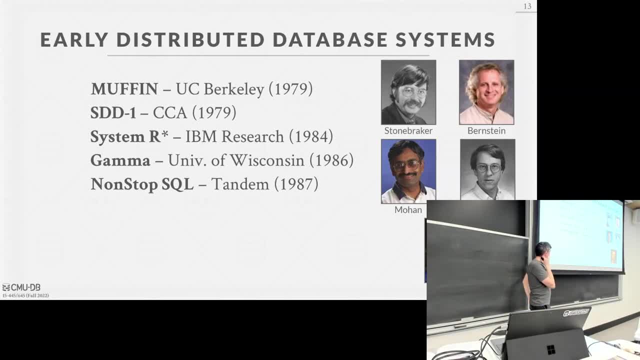 Probably the first two ones were this thing called Muffin from Stonebreaker, the guy who invented Postgres and Ingress, And this was basically Multiple instances of Ingress And then sort of a processing layer on top of it. SCD1 is oftentimes credited as the first one from Phil Bernstein. 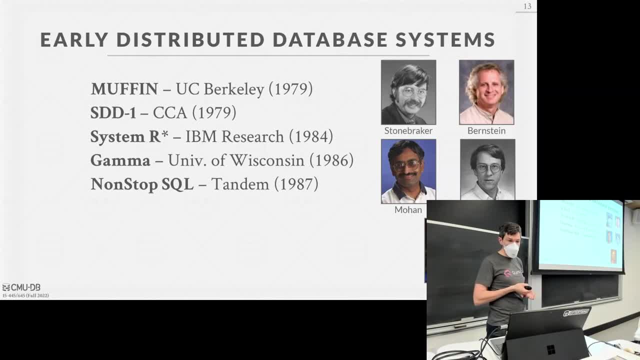 There's a bunch of papers that describe all the early architectures of distributed databases in these papers. But he gave a talk once where he said he didn't actually, They never actually built it. It was just like a bunch of scripts, It was like prototypes to get money from the government. 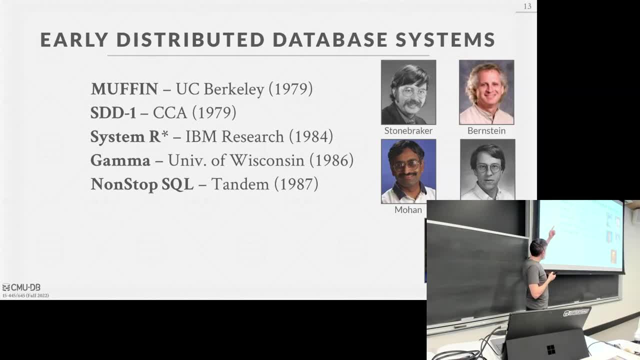 But they laid down a lot of the key theory. At IBM they built a distributed version of System R. the first relational database they built in the 70s, called RSTAR Gamma, was a very influential parallel distributed database out of University of Wisconsin. 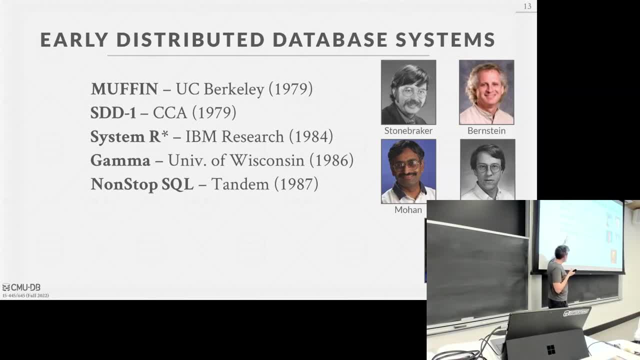 And then, of all these, the only one that's actually still running today is this thing called Nonstop SQL. Again, this was Jim Gray. the guy that invented two-phase locking, worked on System R at IBM. He went to Tandem and helped build out Nonstop SQL. 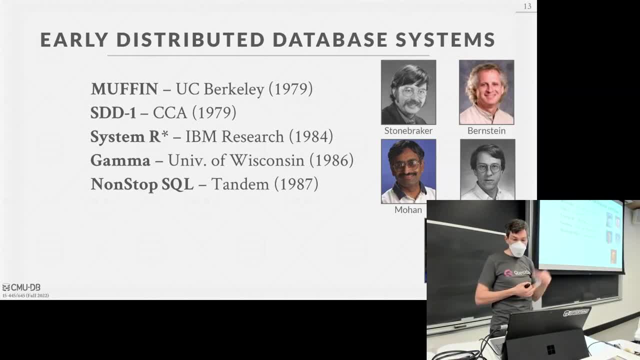 Nonstop SQL is still widely used. If you ever used the ATM, you probably used it. Tandem got bought by Compaq. Compaq got bought by DEC. No, no, Tandem got bought by DEC. DEC got bought by Compaq. 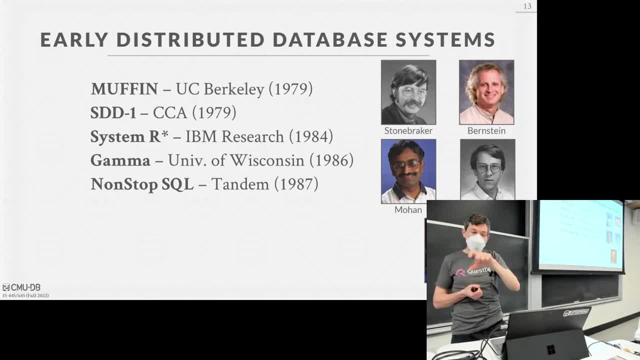 Compaq got bought by HP, So you still can get Nonstop SQL. A lot of banks still use this. But if you're a brand-new startup, you're not using this. But this is one of the first. So Tandem used to sell these devices or appliances called Nonstop. 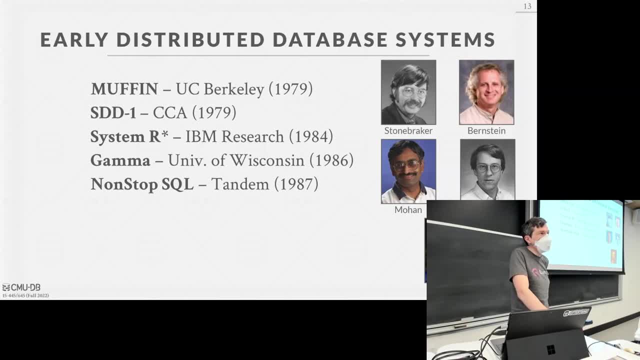 Right Machines or something. And the idea was it was like super redundant hardware, Like think of like NASA level, like where you have like three CPUs running at the same time And then you check to see whether 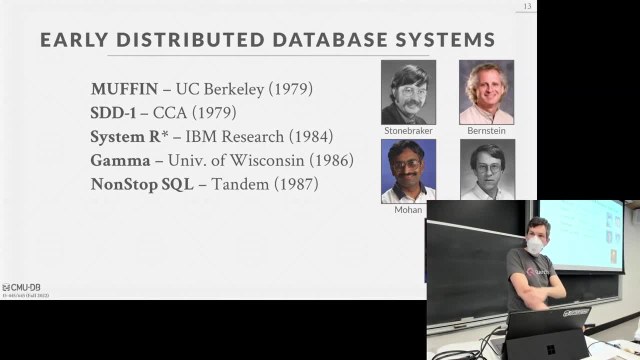 You run some computation and you check to see whether they produce the same result. So the idea was like it would never stop, And if you're a bank, you want that Right. So yeah, it's still around. I mean, they still make a lot of money off of it. 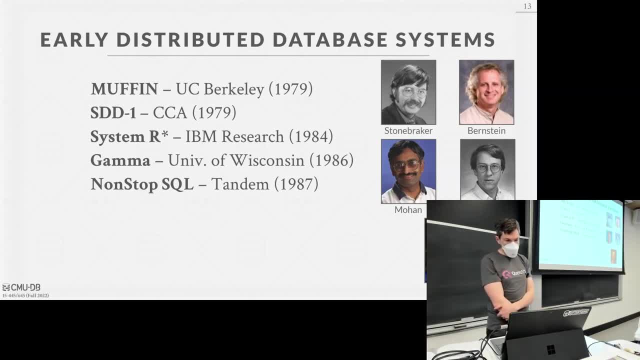 But like it's- You know it's- It's pretty much in maintenance mode at this point, But I'm sure the contracts are in the millions. I mean IMS, like the first database that IBM built in the 1960s. that's still around. 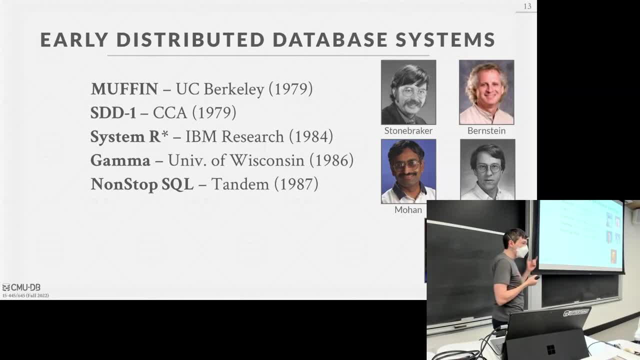 That's still widely used. I think I remember reading somewhere that's like the number one money maker still for IBM is like IMS, Because all the maintenance is, Because it's like mission-critical software that people don't want to change. 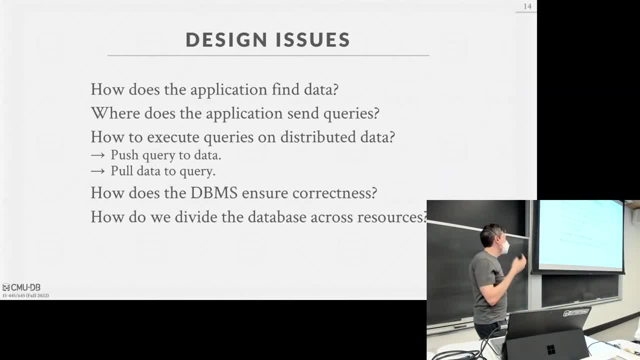 Okay, All right. So now we're at a high level. Like you know, we do share disk or share nothing. There's a bunch of these questions that came up when I was describing the different architectures that we had to figure out. 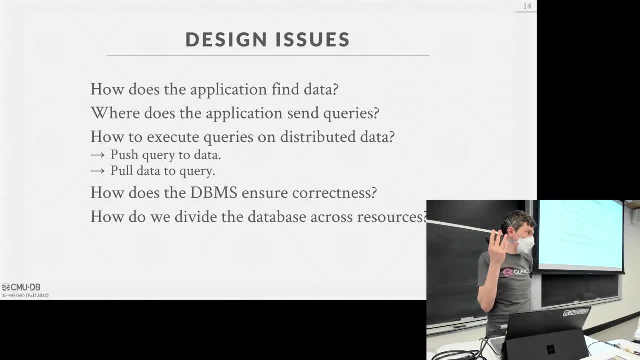 And so the first one obviously was like: how do we actually find, How does the application find data? Like I have a query, Where does it go Right? And then if the data that I need is not at that query? 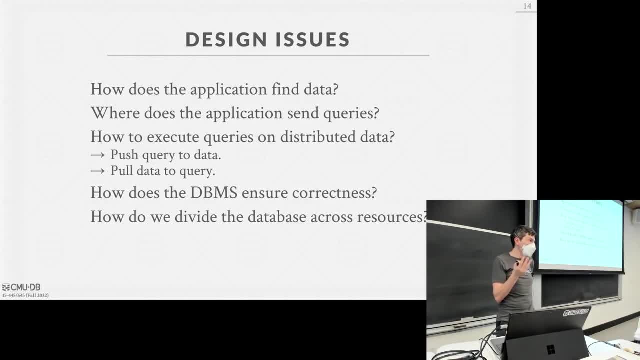 Or sorry at that node, that I sent the query to what happens, Right, And I sort of said there was two cases. There is the query rise at one node, The data it needs is at another node. Do I send the query down? 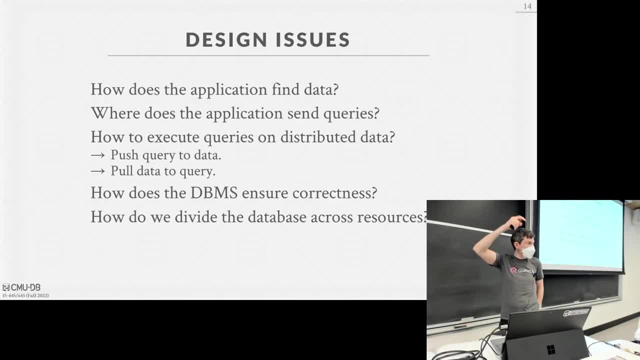 And get back to the result, Or do I send the data up and run the query locally? So it's called push or pull. So you either push the query to the data or pull the data to the query. If it's shared disk, it's always pulling the data from the shared disk layer to the compute node. 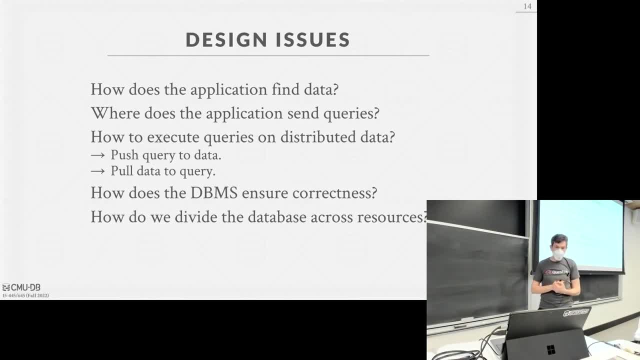 But in shared nothing you could choose one versus another, And there's this tradeoff, of course, obviously Like if the query is, like you know, the SQL string is like 10 kilobytes, But the data I want to scan with that 10 kilobyte SQL string is 1 terabyte. 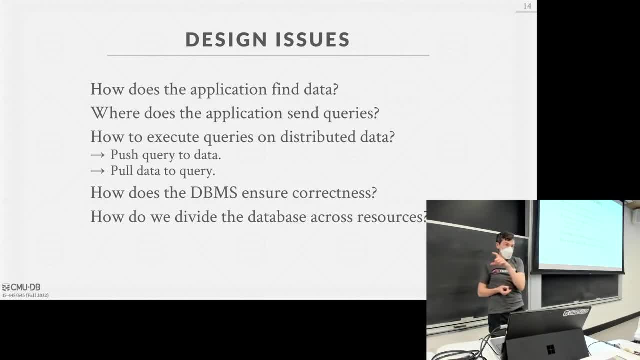 Right. It's obviously better to send the query to the data, But if I don't have any computational resources where the data is, then I can't do that. So this is mostly an issue in a shared nothing system. But even in shared disk, if you have a local disk as a cache right, you still can make that choice. 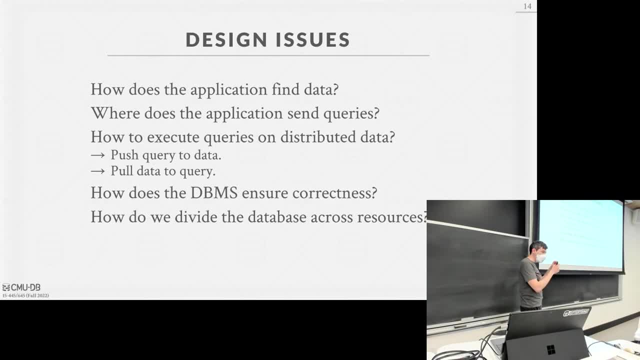 And then the question is: how do we ensure correctness If we want transactions? do we update data on multiple nodes? Do we update multiple data items? How do we make sure that everyone's in sync and says this is the correct version of the data? 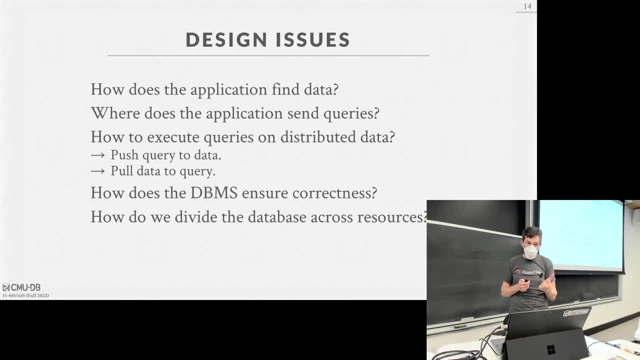 And then how we divide the data across resources. So we're going to cover all of these except for this one. We'll cover this in more detail next class. So we'll get into two-phase commit, We'll get into Paxos and RAFs and all that good stuff. 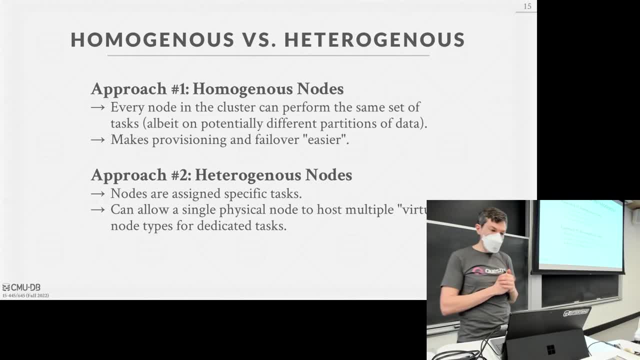 Okay, All right. So the next thing we have to make an addition is like: what do our nodes actually look like? And this is the notion of like. are the nodes homogeneous or heterogeneous? Homogeneous cluster would be: every single node in the system or in the distributed data system is like a first-class entity, meaning it can do all the tasks that any other node can do. 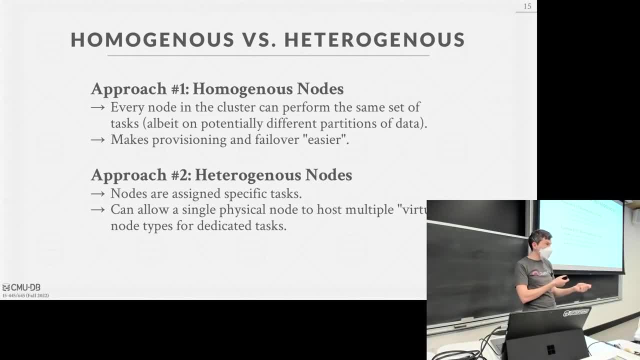 Right. It can take any query. It can take any transaction request. It can move data around- Right. This is ideal. because this arrangement is ideal because it makes it easier to do provisioning and failover, because if a node goes down, you could take it down. 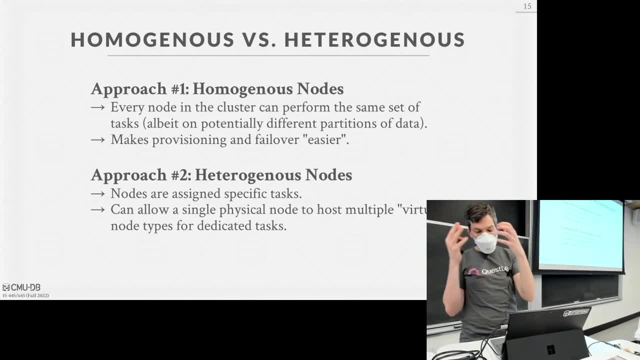 You could take another node and just fill in for it, Right? You know, if I'm designating some nodes to do some special operation, these other nodes do the other special operation. If I run out of nodes in sort of one category, I have to mainly go and say, okay, let me take resources out of another one. 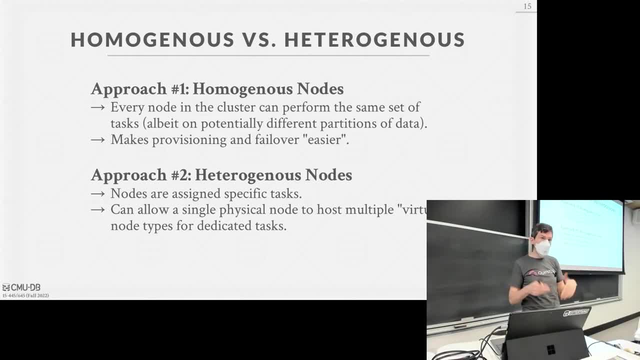 Less of an issue now with the cloud, because it's easy to spin up new instances If you're running on prem in a non-virtualized environment. this is harder to do In a heterogeneous cluster. all the nodes are assigned to specific tasks. 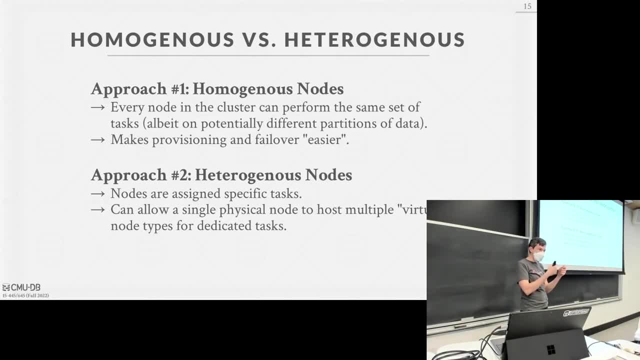 Now you may have a single physical node, have multiple demons or processes running at the same time. that can do the different responsibilities And that avoids the network message between them. But again, at a really large scale you want them to be separate because each sort of task could be very compute, heavy. 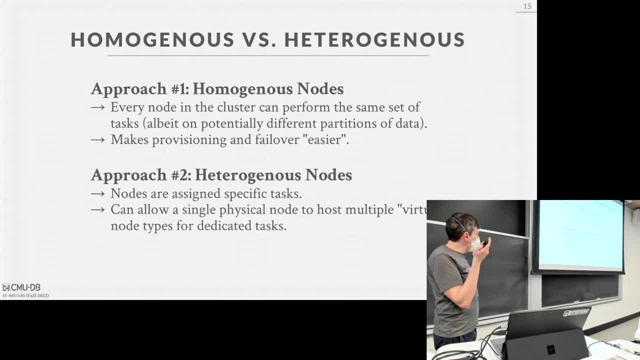 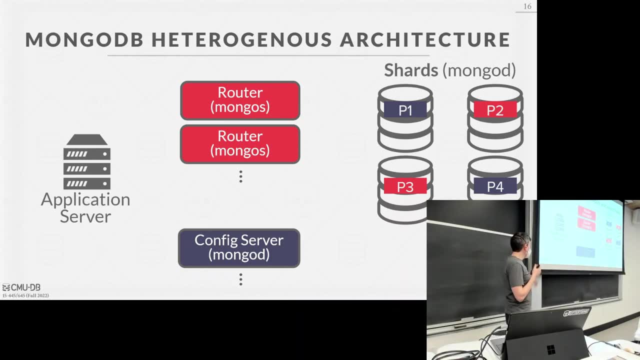 So to explain what- sorry, the homogeneous one is pretty obvious to understand, To give an example of what the heterogeneous one looks like, I want to give an example of what MongoDB's architecture looks like And I'll say that this is the MongoDB. this is like the version of MongoDB you run on prem. 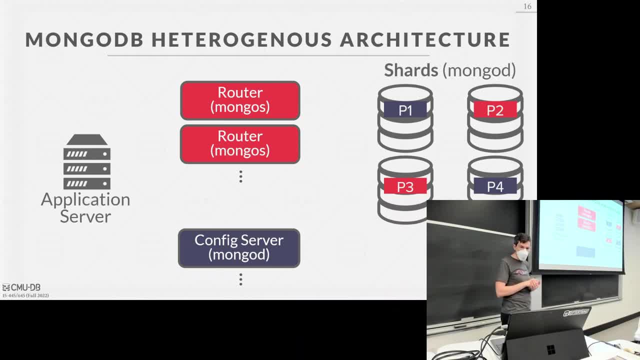 They have their own cloud version and they sort of hide all this for you. But if you download MongoDB and run it on your local machine and it just should be set up, you would get something like this: So we have an application server. 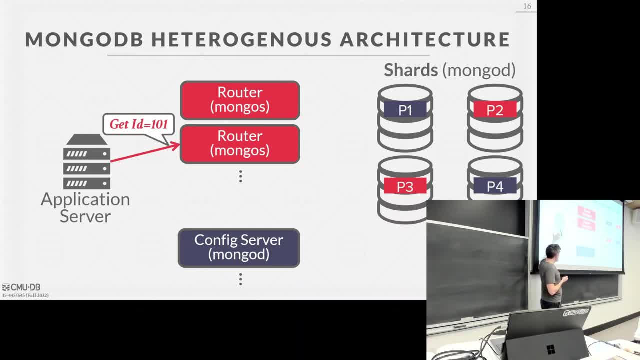 And it's going to send query requests to this special node called a router And it would examine the query request and say: I want to get you know, I want to get this, You know the record ID 101.. So then it would go down to this thing they call the config server. that's going to maintain its own internal state about where all the data is located in the database. 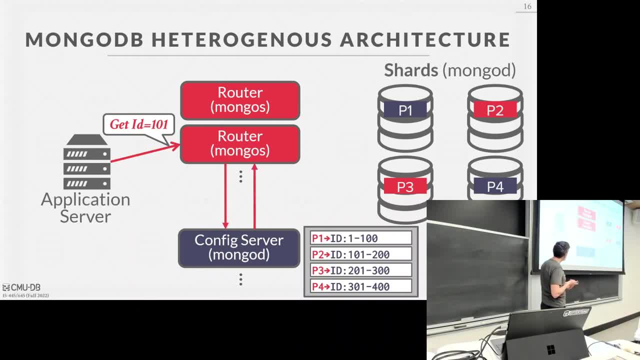 What partition has- or shard has- the data you need. It sends that information back to the router, who then now routes the query to the appropriate node that has the data that it needs, Get back the result And then you send it back to the client. 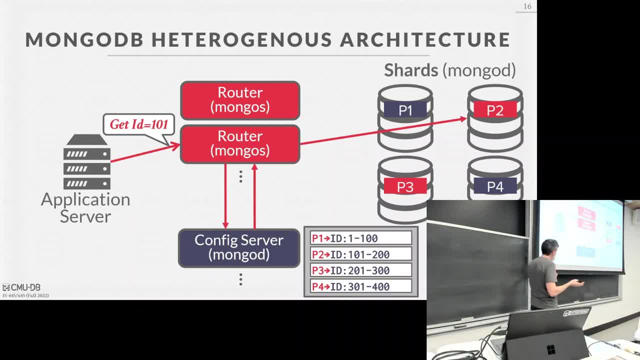 Right And sort of this Transparency between the application and the database itself, where it doesn't need to know how many partitions it has, Where the partition is located, How much disk they have and so forth. All that's hidden from you Because the router thing is responsible for sending your request to the right location. 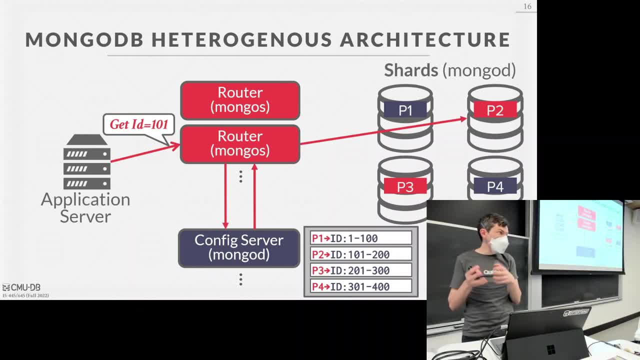 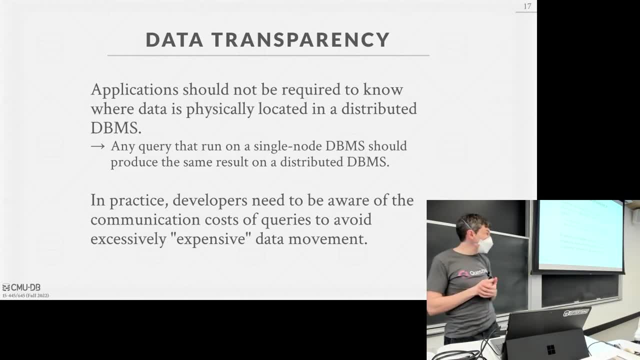 So this is sort of clear. So you have different nodes that have special tasks, And so this is just repeating what I've already said. We want this notion. We want to achieve what is called data transparency, where the application should not know anything about a distributed database. 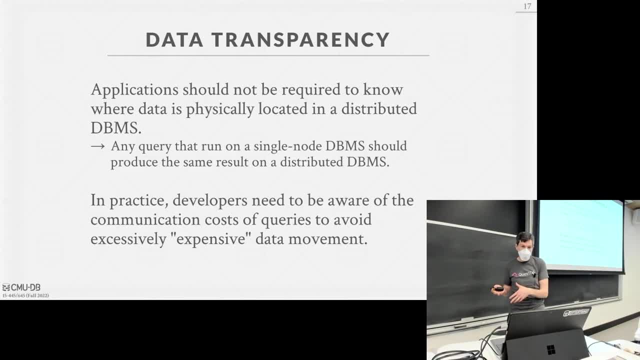 It should not know how many nodes it has. It should not know anything about where the data is actually located. Right, And any query that we run on a single node instance of our database should also run and produce the same result on a distributed database. 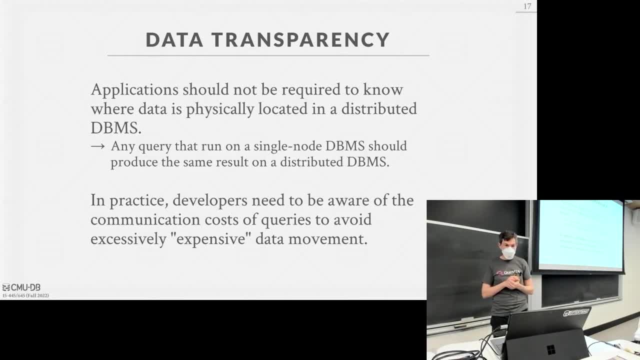 Again, regardless of how I scale things and change things Right Now, in actuality, when you're building an application, there's a lot of data, But when you're using a distributed database, you kind of do need to be aware of where your data is actually located. 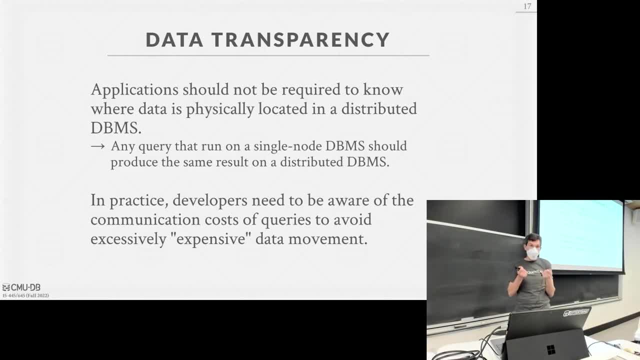 So you don't do stupid things Like if I have to update two records and those two records are on different parts of the world, If I do it in a transaction, then what's going to happen? Then I have to do multiple round trips to coordinate over the network going out into the ocean between these two data items in my database. 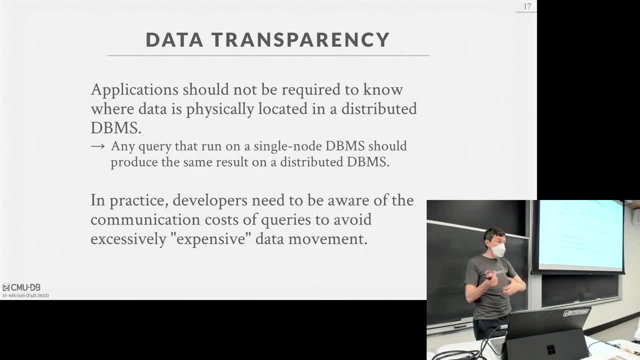 And that can be very expensive. Or if I want to run a query that wants to scan a petabyte of data, I don't want to have to pull that petabyte of data from, you know, from Europe or Asia back in the US and process it. 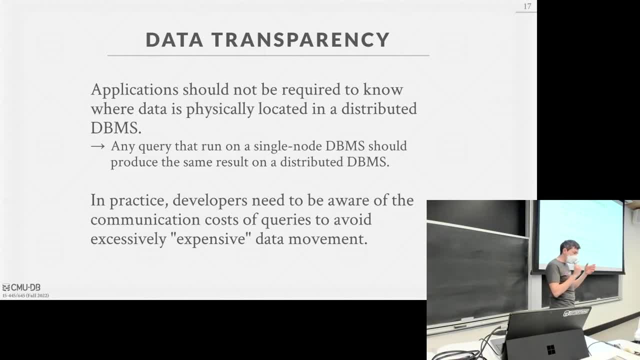 Ideally I want the. you know, maybe I could send my request to the right sort of the. not the right node, but, like the right router, The thing that knows how to get data, you know, run queries on that part of the world. 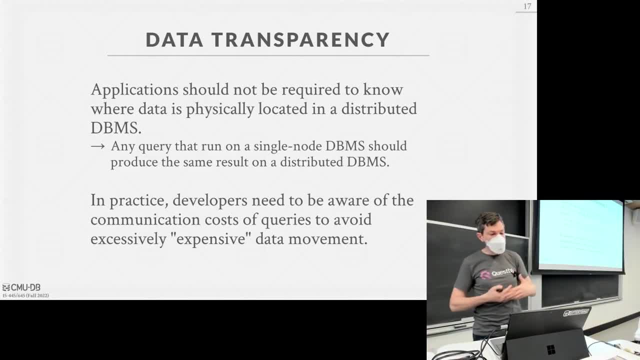 Right. So what I'm just trying to say is we don't want to have special syntax or introduce any modifications to our SQL queries to say, Okay, Hey, scan this. you know, run this query on this table located at this location. 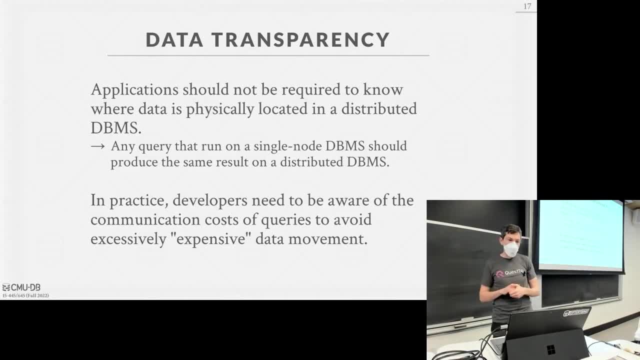 Right, We want the data system to handle all that for you, But again, you need to be sort of aware where things, where the data, is actually located, to make sure you don't- do you know, you don't run things that are more expensive than they should be. 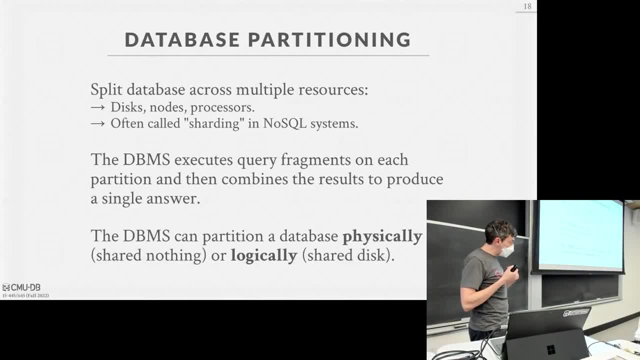 So now we need to talk about partitioning, because this is something that we've alluded to when we talked about parallel execution, And I'm showing examples now, where I have these different databases and they're being split up And queries are going to one location versus another. 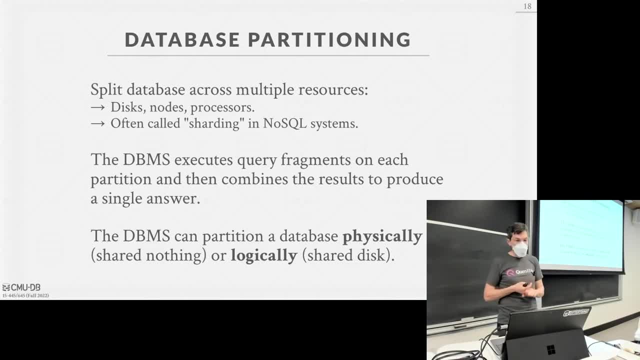 So now we need to talk about how we actually do the splitting. So the idea is that we want to split our data across the multiple resources that we have, Again depending on if it's a shared disk or shared nothing or shared everything. 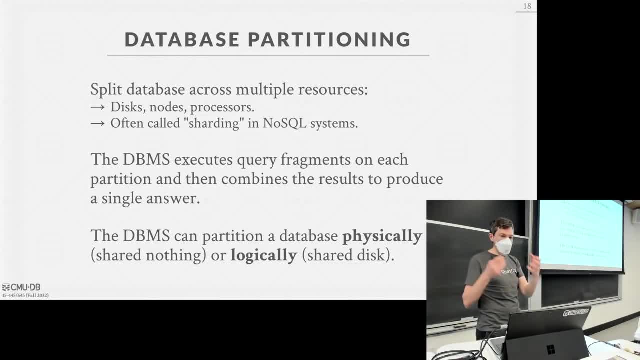 Right, It could be splitting across different hard drives, different physical nodes, different CPUs, different memory regions. I'm going to use the word partitioning because traditionally in academia and also for the relational databases, They're referred to partitions. In the NoSQL world or on the Hacker News world they're going to refer to these as shards or sharding. 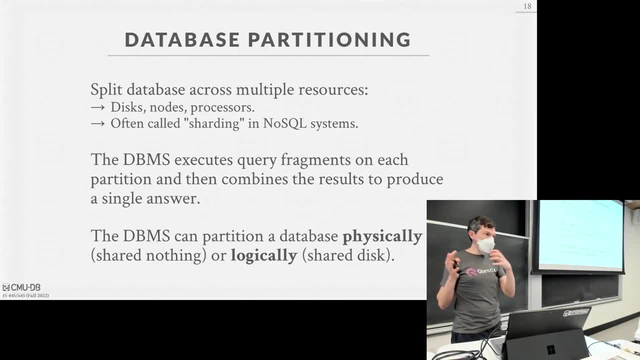 The basic idea is the same. We're going to split the database up into disjoint pieces And the idea is that, just like as we did on parallel execution, where query shows up, we generate the query plan And then we want to break this up into physical fragments that we then send to the different partitions to run in parallel. 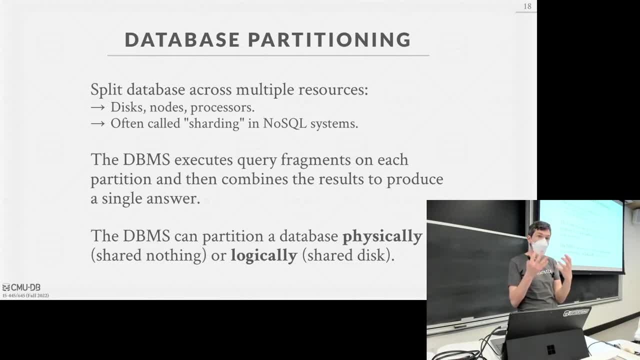 It's the same idea and it should be a database. And then we want to combine the results from the different fragments into a single answer. So the database system can be able to partition a database either physically, if it's a shared nothing system, or logically, if it's shared disk. 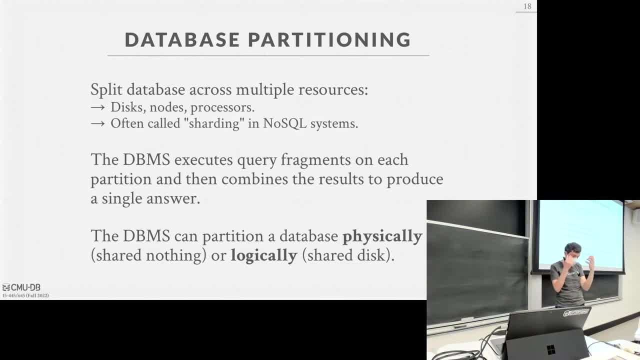 Right, And again it has to do with where the final resting place or the primary storage location of the database is actually being stored. So let's go through a bunch of different examples of different types of partitioning schemes you can have, And then we'll discuss the tradeoffs of actually trying to support these. 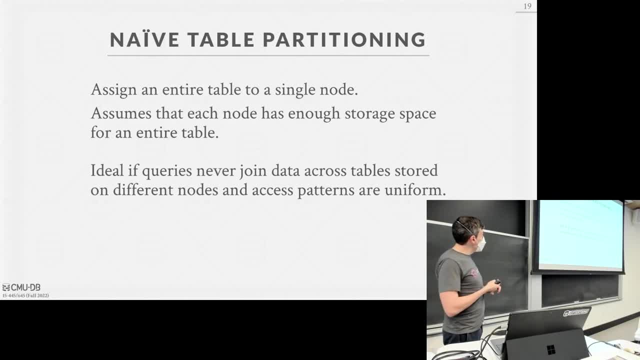 Okay, So the easiest way to do partitioning is just what is called naive table partitioning, Where you take the entire table and assign it to a single node. Like if I have two tables, one goes to one node and the other table goes to the other node. Right, This obviously assumes that you have enough storage space to store the entire table in each node. Assumes that most of your queries are going to only access one table at a time. Right? This would be terrible if they're joins. And then, of course, what happens now if you add a new table? 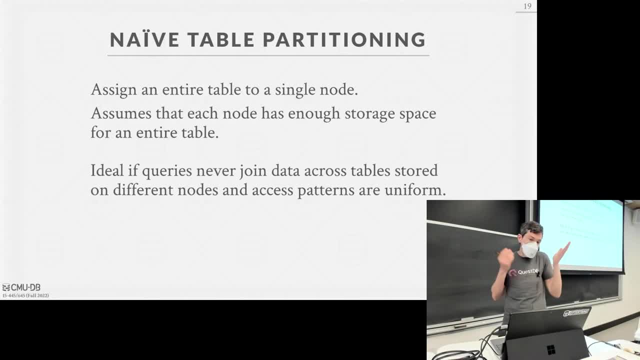 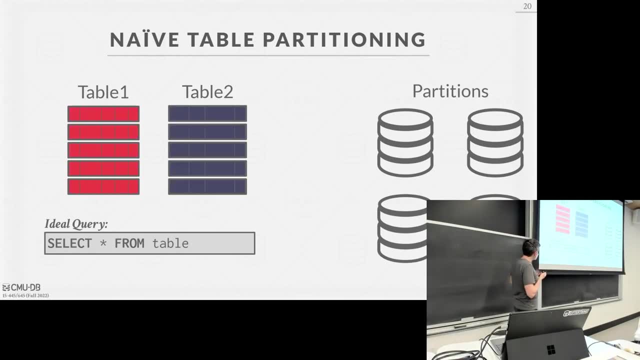 Where does that go? This complicates a bunch of things, But this is the easiest way to get to split a database up. So it looks like this: So I have two tables, one and two. I literally take all the tuples from table one, store it in that node and that's partition one. 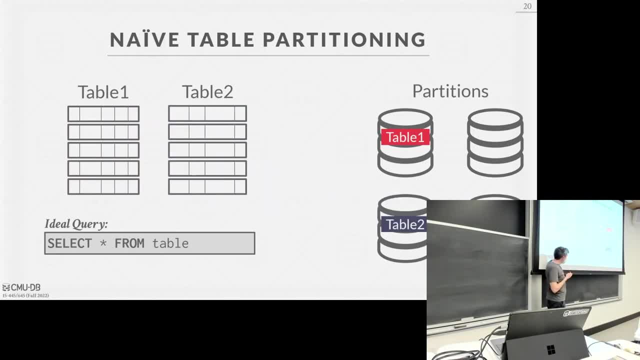 All the tuples from table two and that goes to this partition two here. Right, And the best case scenario for me for this arrangement is every query only accesses one table, So very few systems will actually let you do this. Mongo is the one that I could think of where you could say this node, this table will be. 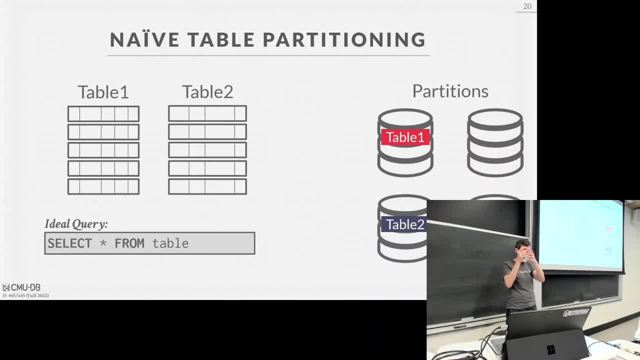 or collection, they call it. This table will be dedicated to this single node And they would do this for some cases where they have applications that want to update the actual database itself but then append, like a log record, into a table, And so you'd put that log table on a separate node. 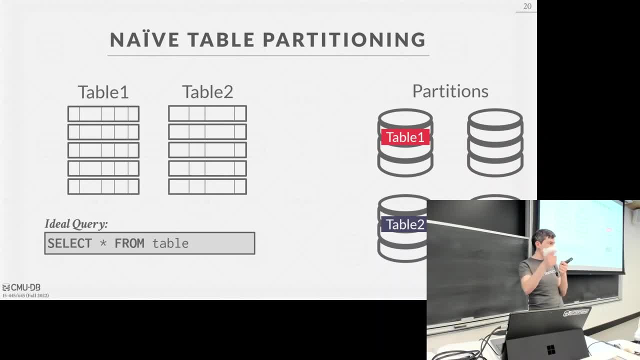 So you just blast the inserts over to that thing And it didn't interfere with updates. Right, It was just updating the actual database itself, because you never went back and read the log unless you were doing like an audit later on. Another type of partitioning is called vertical partitioning. 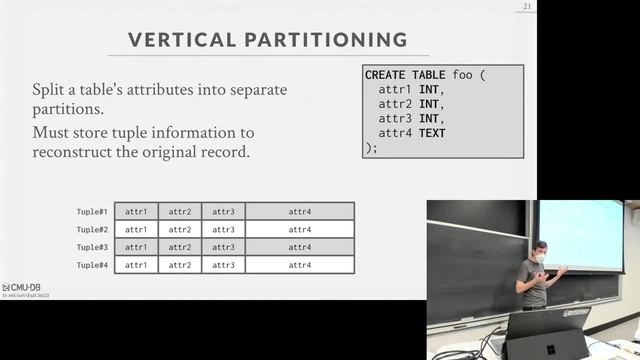 And the idea here is basically you want to sort of simulate a column store where you're going to take a table and split across its attributes. So all the tuples for all the values for some subset of attributes, for all the tuples go to one partition. 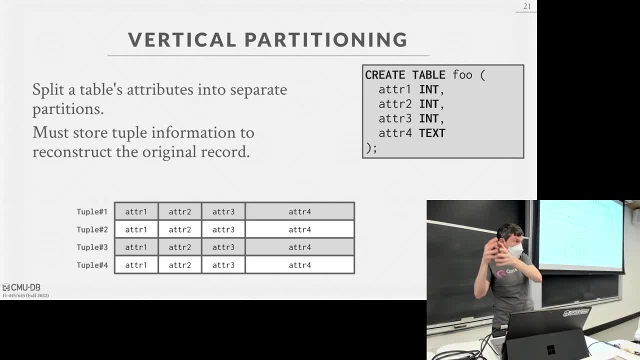 and all the values for some other subset are attributes. Go to another partition So say I have four tuples here and they have four attributes And say the last attribute, attribute four, is a large text field. So what I want to do is just break it up so that there's one partition that stores just the first three attributes. 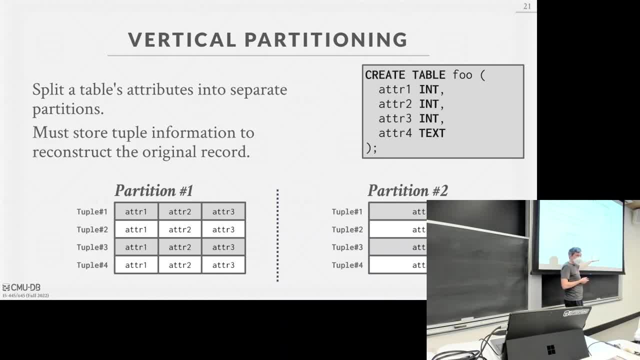 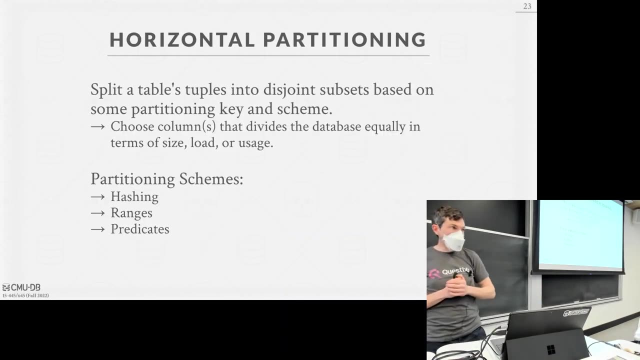 and then another partition stores the last attribute And again it's like a column store. I would have to know how to map or combine them back together to produce the original tuple. All right, What is more common in distributed databases is called horizontal partitioning. 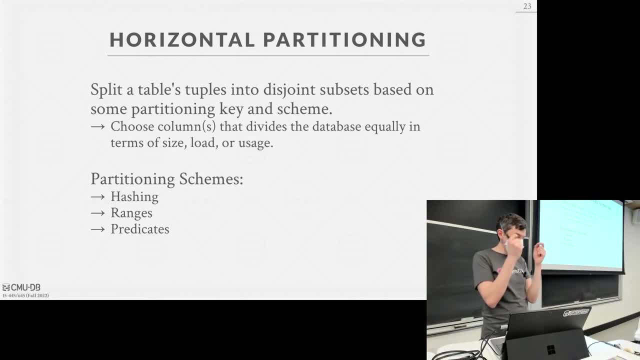 And the idea here is that we're going to split the tuples up into these subsets where all the attributes for that tuple, all the columns, will be stored together continuously on the partition. Well, it doesn't have to be continuously: If it's a column store, you can store the same thing. 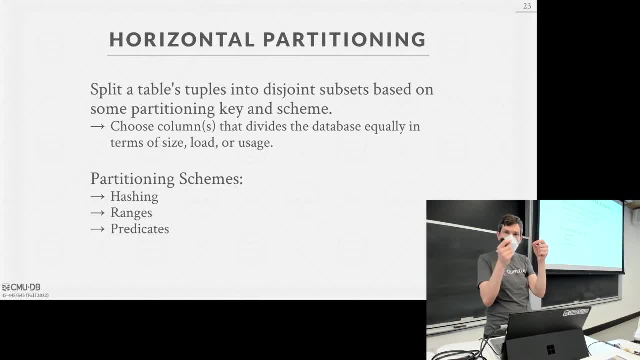 But if I want to get all the values for a single tuple, it's going to be on one partition And the challenge here is that we want to try to pick a partitioning key and a partitioning scheme, the mechanism we're going to use to divide things up. 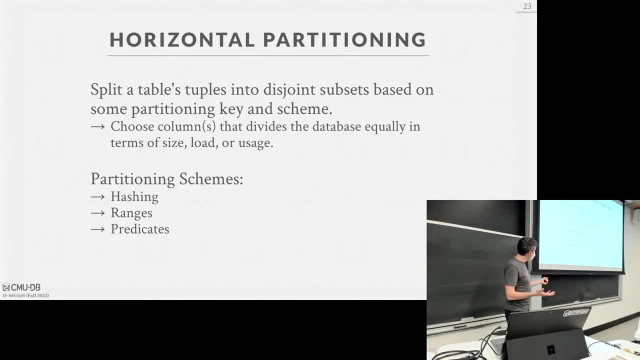 in a way that's going to divide the database equally across the different nodes by some metric: The storage size, how much queries are going to get sent to them, how often they're going to be updated, and so forth. So picking the right partitioning scheme is actually the NP-complete problem. 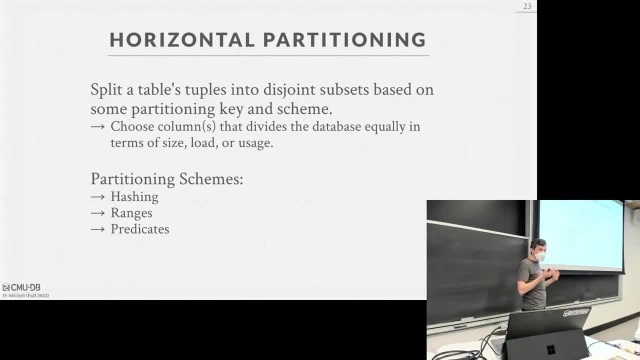 We're going to have to research on how to do this automatically. Oftentimes for OLTP, it's quite obvious. It's usually. the schema is a tree structure like customer ID. You have a customer account, customer orders, customer order items. 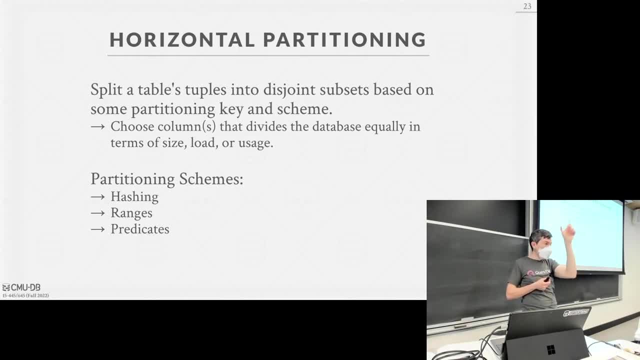 You would partition the database or those tables on the customer ID For OLAP. it's a bit harder, as we'll see next week, because I could be doing joins across any arbitrary keys and one partitioning scheme for one query may be the best. 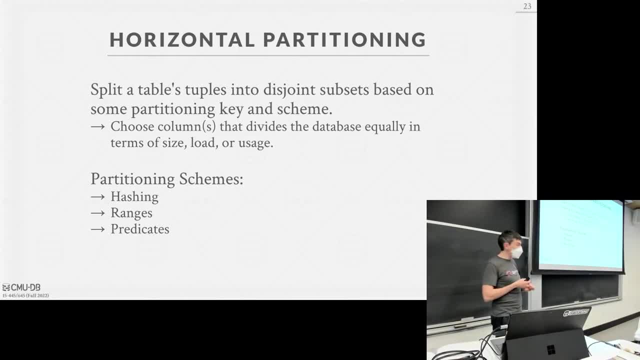 and it could be the worst for another set of queries. So trying to figure this out is non-trivial. So I've already shown sort of range partitioning. already There's some partitioning key, there's some column. I'll say from 0 to 100 goes one partition. 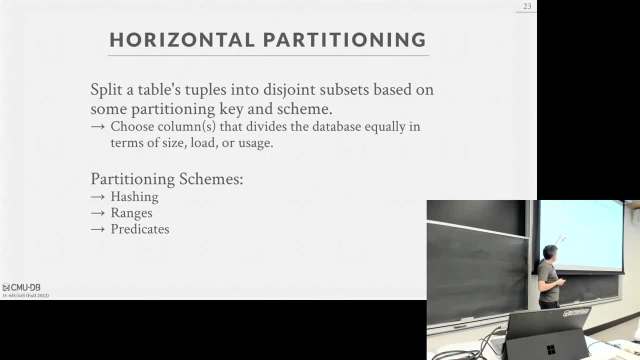 from 101 to 200 goes another partition. Oftentimes, though, hash partitioning is widely used. Predicate partitioning is not that common. Basically, think of it like a WHERE clause for any tuple that you then would use that to figure out what. 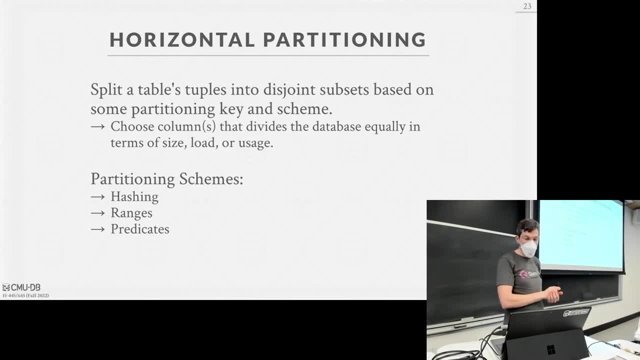 you know it's like a routing table: say where that tuple actually would go. It's usually hash partitioning or range partitioning, and then between those two, hash partitioning is usually more common, especially in OLTP workloads or the NoSQL systems. 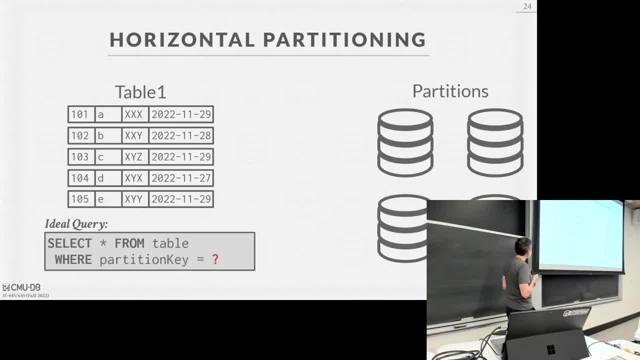 All right. so let's see how to do this hash partitioning for this table here. So the first thing we've got to do is pick a partitioning key. So say we pick the second column here and we're going to do hash partitioning. 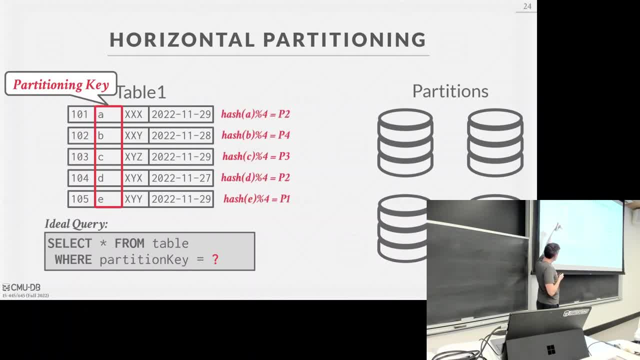 So we have four partitions. So what we're going to do is we're going to take the value for each tuple for this column here, run our hash function right: xxhash, whatever one we want. modify the number of nodes that we have. 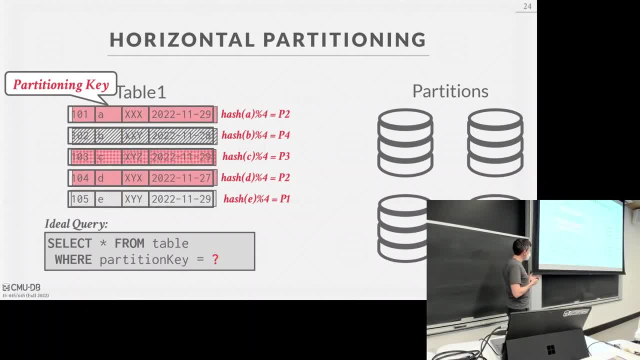 partitions we have and then that's going to determine where this data goes right, And then they'd be split up into partitions like this. So now any query that comes along, and in their WHERE clause they have an equality predicate that is doing a lookup on exactly our partitioning key column. 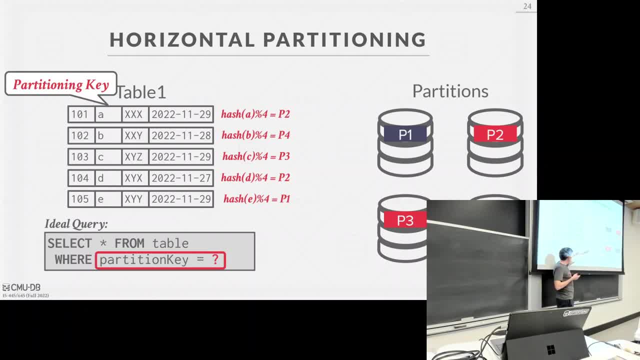 We just take this value. they're passing in hash that modify four, like we're doing an example here, and that tells what node has the data that we want. And again, this is something the database system does. You wouldn't do this in your application. 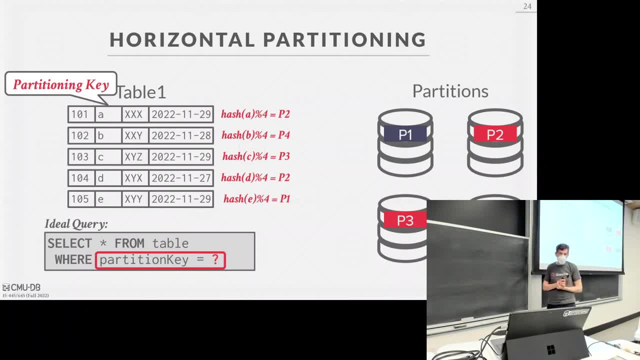 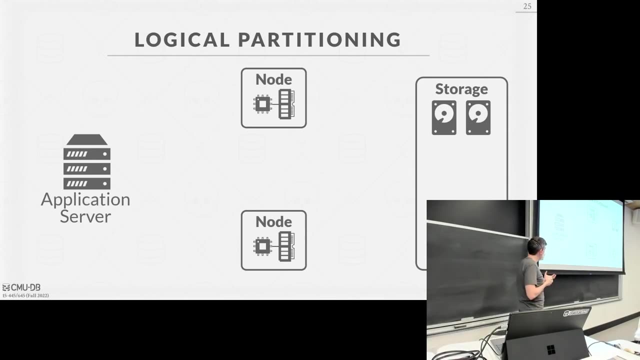 The data system would figure this out for you. So this is clear. Okay, so now let's talk about the difference between logical partitioning and physical partitioning. So in a shared disk system, logical partitioning means basically, it's a way to denote. 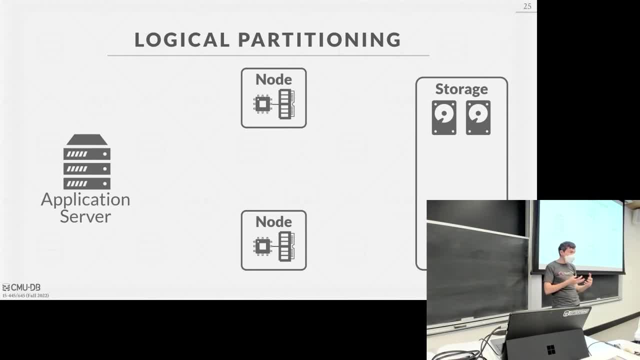 what node is responsible for processing the data or the queries that touch the data within some partition. right, So say: we have out on our storage device, we have four values and then now there'll be some metadata we keep track of at each node that says: 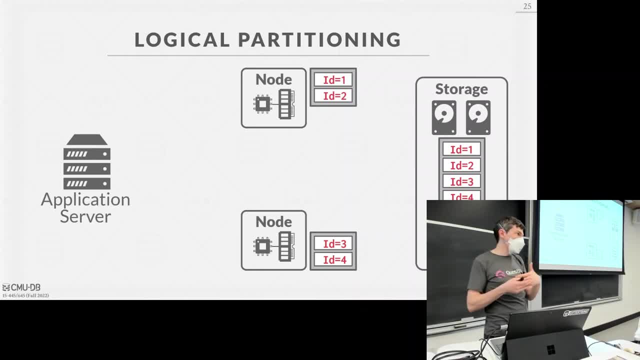 I'm responsible for IDs within this range or things that hash to me. So now, when the application server says I want to get ID one right, There could be something up in front of this. tell us how to route there. We can ignore that for now. 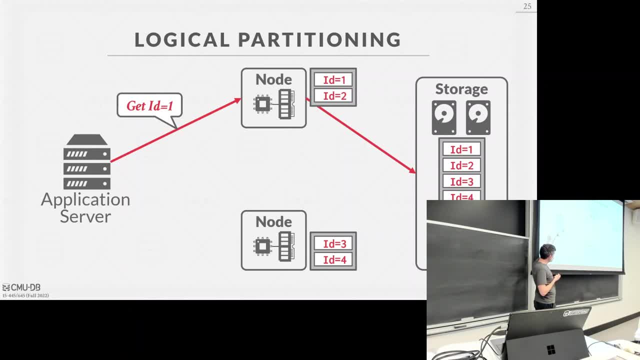 but say it goes here and this guy knows I'm responsible for this, so I can go to disk and get it right. This guy wants to get ID three. same thing, He's responsible, He can go do that. And so now, if I want to get multiple ones, 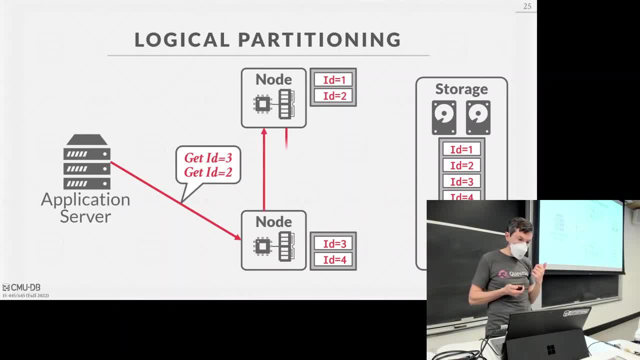 as I showed before, we have this decision where we know that this node doesn't have ID equals two, And so, rather than going just to disk, going out to disk and getting it, because then everyone knows it could potentially have a copy. 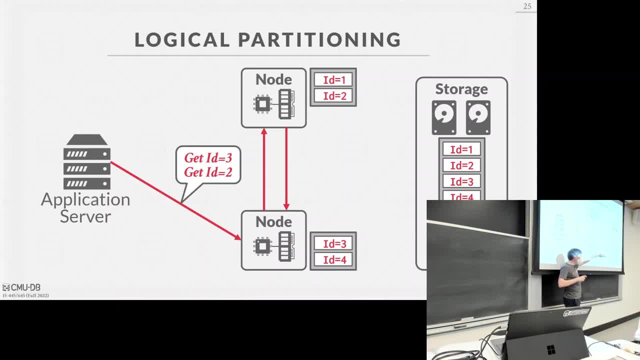 and that would be a problem. if I want to do an update, where do I go to update it? How do I tell everyone I've updated it? We could have this thing say: well, I'm not responsible for ID equals two, so let me send the query request. 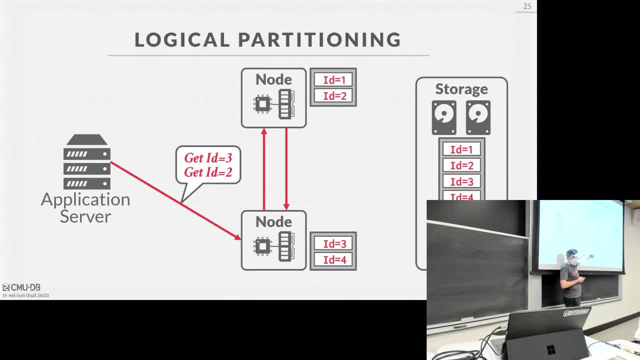 or the data request up to this node, and that node could either send me the result of the query or the actual data that I want- and I maintain an ephemeral copy- and then I send the result back there. Physical partitioning in share: nothing. 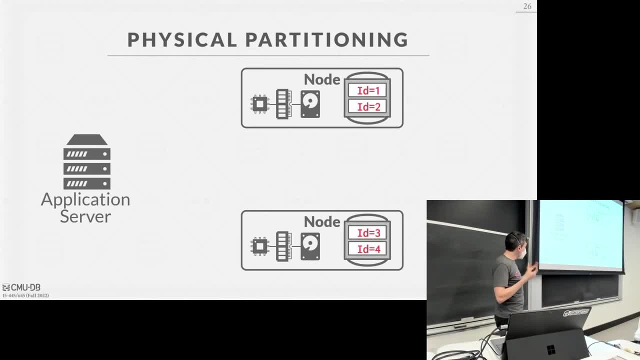 is where, again, the data is actually physically located. So, just like before I'm splitting up on ID, So when I want to get ID equal one, I know to go up here and get it. That's fine. When I want to get ID three, 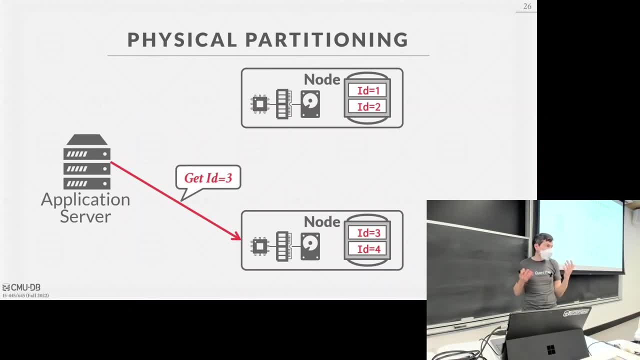 I go down here and get it and that's fine. And if I do, the same message patching as before. if the bottom guy wants to get ID equals two. then I can either send the query request or the data request and I can have a local copy. 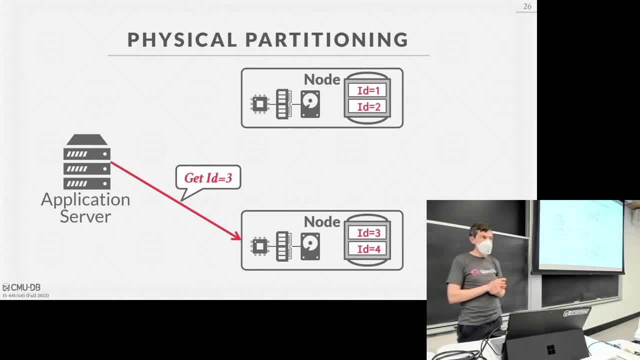 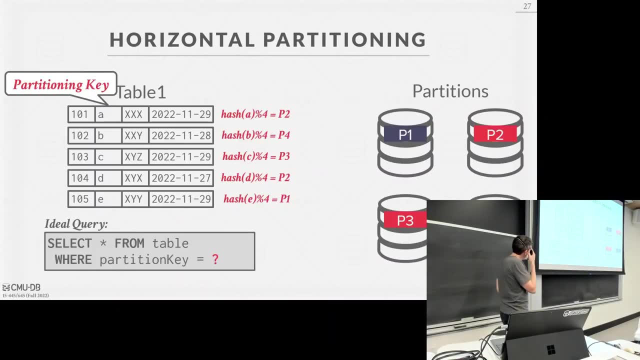 at the node on the bottom. Okay, So let's go back to this example here. So again, we were doing hash partitioning on the second column here, where I take the value for this column for each tuple hash. it mod four. 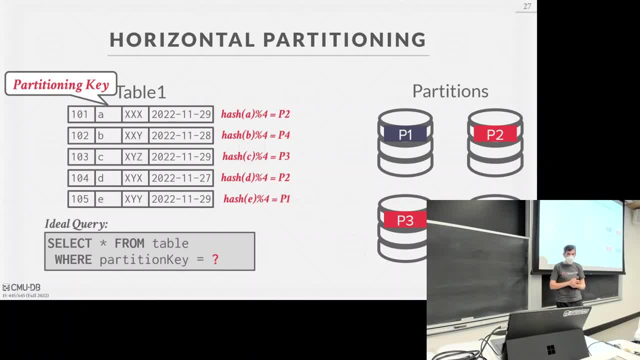 and then that tells me where the partition will actually be stored. What's the problem with this approach? Yes, As you add four nodes or you remove nodes, you have to move around. Bingo, He said: as you add new nodes, you have to move stuff around. 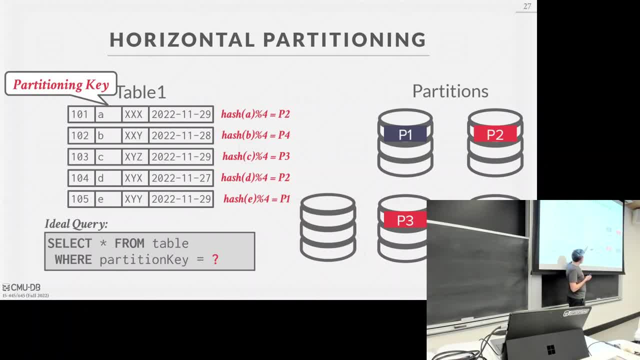 So if I add a new node here, then I can't mod four anymore, because I have five nodes or five partitions. So I've got to go ahead and rehash everything, which is going to require me to shuffle everything around. Now range partitioning. 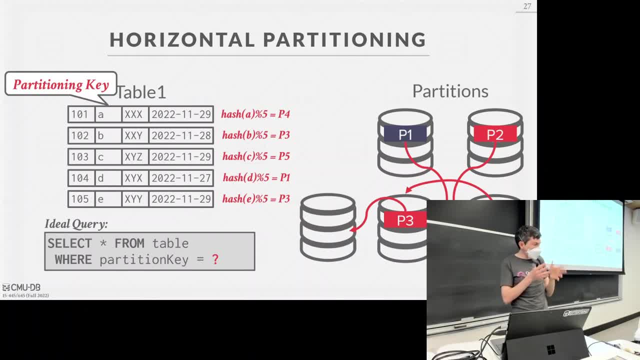 you can excise the ranges and you can play a trick there. but if you're using hash partitioning, this won't work. You have to remod everyone again. So the solution here to this problem is actually what is called consistent hashing. 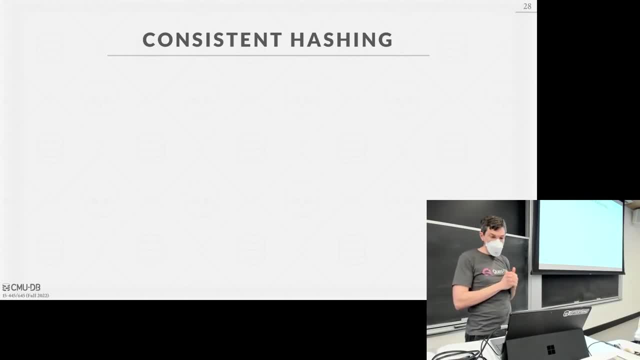 Who here has heard of consistent hashing before? Less than half, less than 25%, Okay. So consistent hashing is a really neat technique and it's widely used in both distributed databases, mostly on the operational side, operational systems, less for OLAP. 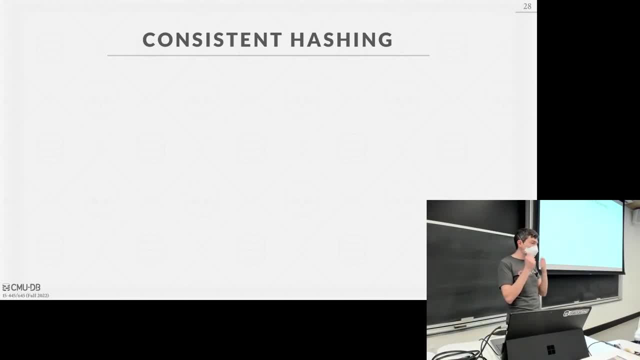 but certainly distributed systems in general. It's a technique to basically avoid this reshuffling problem. It was developed at MIT in the early 2000s, So the way to think about it is that the hash range for some partitioning key is going to be represented. 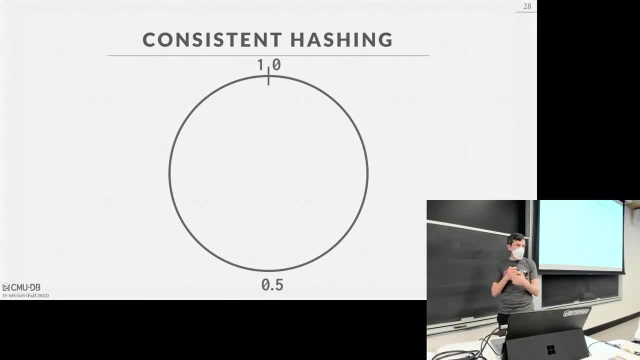 in this circle, from zero to one, And the idea is that we're going to hash the data that we have. you know, we want to start each partition. we're going to hash it and then map it to this circle here. So say, partition one. 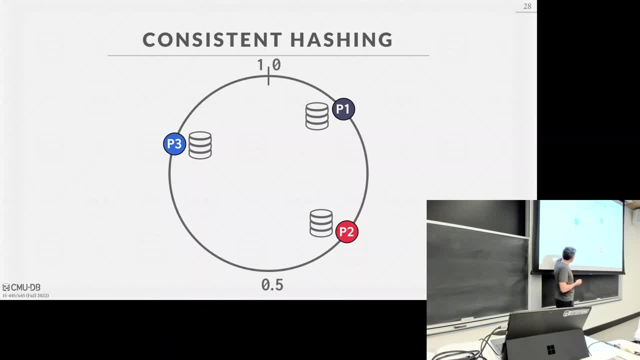 is this part in the ring. partition two is down here, partition three is over here. So now when I want to do a lookup and say, go get me ID equal 101 or whatever the key is, I'm going to hash it. 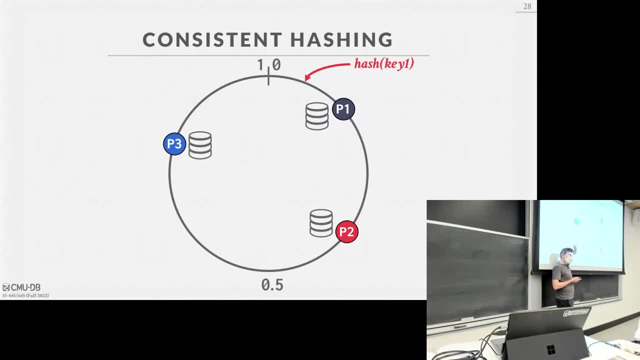 then it's going to land somewhere in the ring and then I just move forward in the ring to say what's the closest, what's the closest partition. you know, based on my location where I'm in the ring, what's the closest partition. 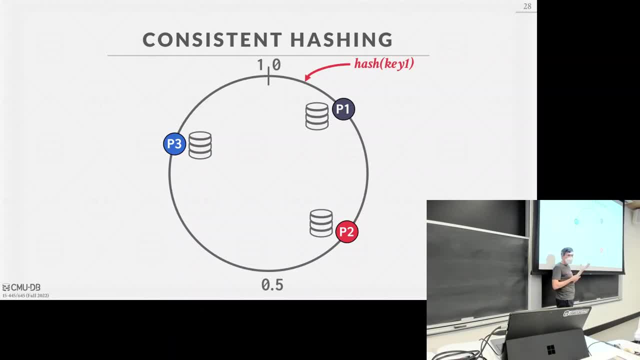 to me going in in clockwise order and that's where my data is going to be stored, Right? So I'd land here in the ring and I would scan down and say, oh, P1 is actually what I want, Right? Likewise, 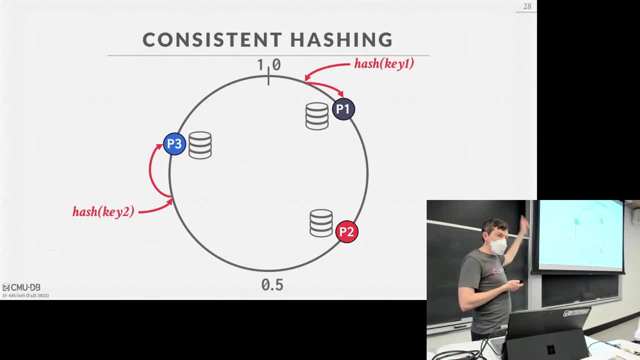 if I do another hash over here, I land in this part of the ring. slide up P3 has the data that you want, So the way to think about this is like these partitions are going to cover the key space on the hash ring. 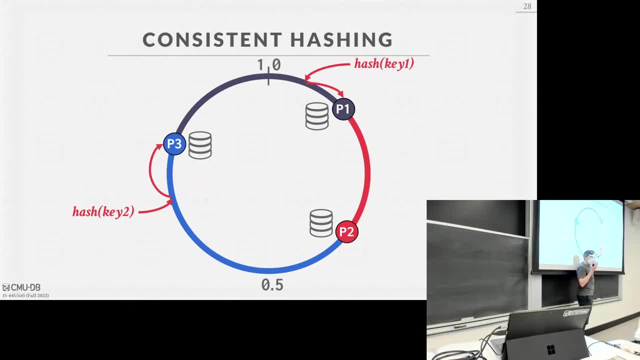 from the point where they're located around to where the next node is Right. All right, So so far this seems pretty okay. This is fine. What makes this special? Well, when I have a new partition show up here. 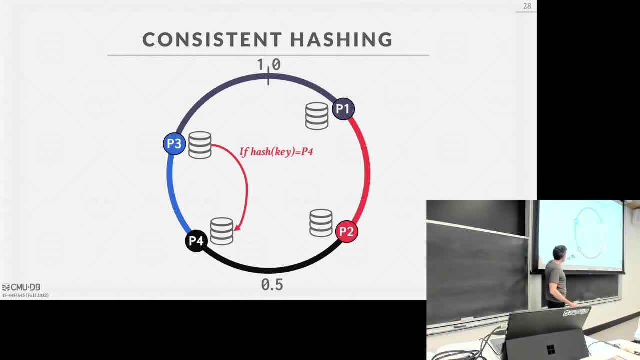 the only thing I need to do now is just move the data that used to be covered by the next partition above it in the ring I, since I'm excising or splitting in half all the data over here from P4 to P2. 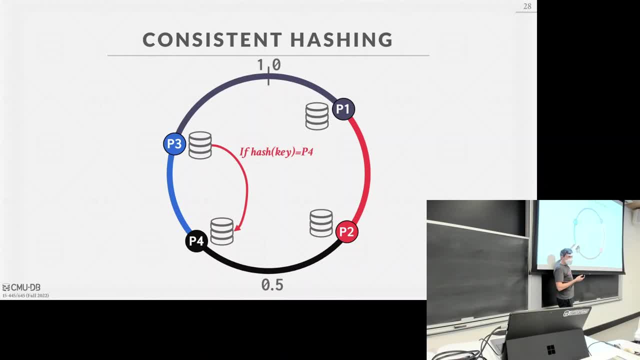 that used to be in P3, well, it only needs to move, get moved to P4.. All the data in the other partitions don't have to move at all. Right, Again, same thing I. I add another partition. 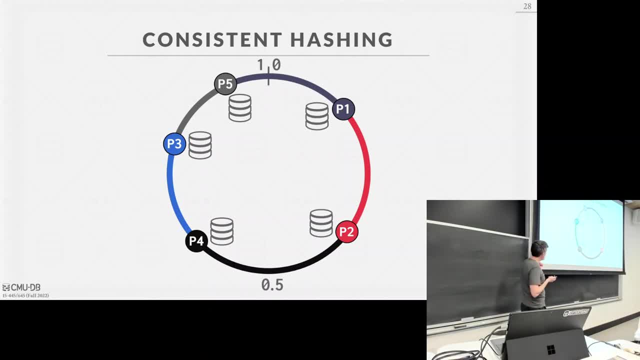 P5 here. That splits the the range from P3 to P1.. I only need to move the data from P1 that that. that falls at this point in the ring. Same thing: I add P2, I only move that data. 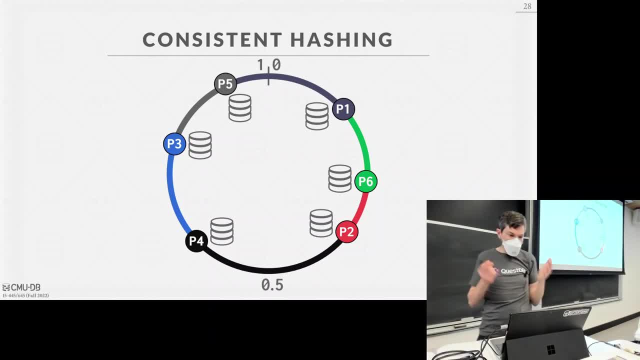 So I'm not. I don't have to reshuffle the whole whole, the whole ring, the whole partitioning scheme, The the change or modification is is localized to just that part of the ring. Okay, So how do I find data now? 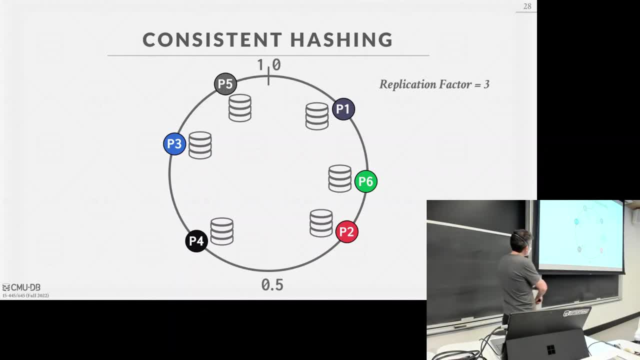 So to have better availability, which we'll cover more in the next class, I actually want to store the data across multiple nodes or multiple partitions, So so you would have this notion of a replication factor, meaning like for every single time. 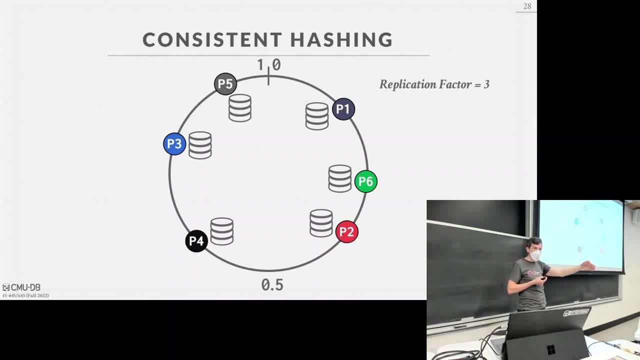 I insert a new record into the database I'm going to store on three different nodes or three, three different partitions. So let's say any data that I would store in P1 here, I'm also going to store them in the next. 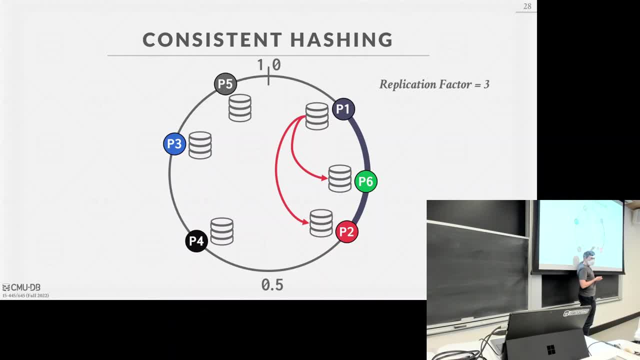 two nodes in the ring, so P6 and P2.. So now when I, when I want to do a lookup and say, go find me key, key one, I'm going to hash it. it lands here in the ring. 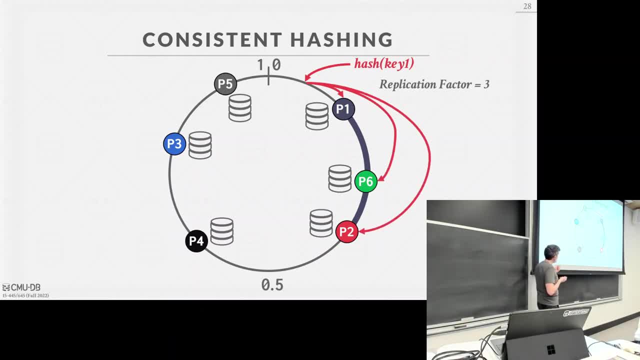 and then I know that I have, and then I know I could either go fetch it at P1, P6, or P2. And all of them would would potentially have the data that I'm that I'm looking for, Of course. 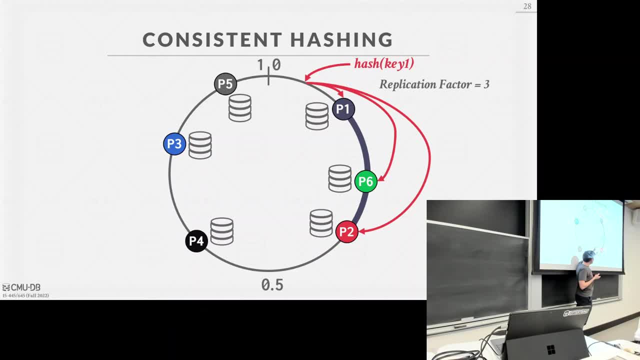 this makes writes more complicated, right? How do I make sure that if I write something to P1, it gets to P6 and P2?? Okay, we'll talk about that next class. You either wait for all of them to acknowledge it. 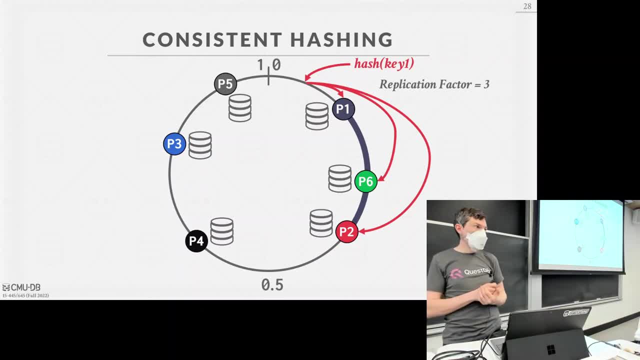 or you can wait for a majority to acknowledge, depending on your, your tolerance. So, as I said this, there's a very influential paper in the early, early 2000s for MIT, called Cord, that invented this technique, But then, most famously, 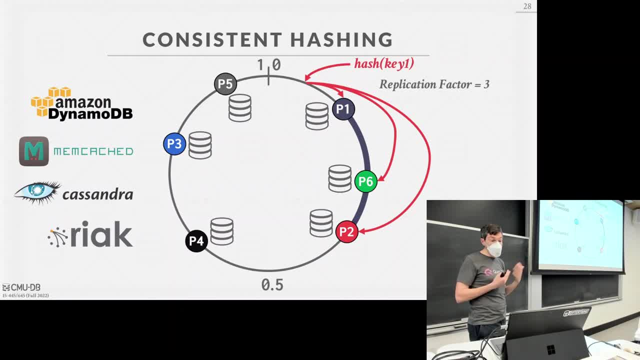 Amazon picked up this idea and they implemented it in Dynamo- DynamoDB- in the the late 2000s. There's another system called Memcached, which is a like a in-memory distributed hash table for for caching things. It's basically a database system. 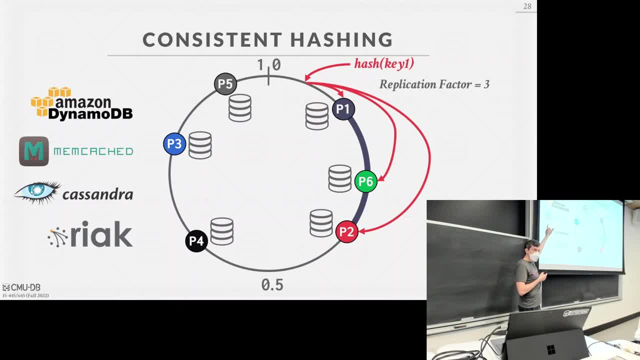 They use this. Cassandra was written by Facebook originally to power their mailbox. The guy that founded Cloudera wrote Cassandra at Facebook. in the mail, Facebook says we don't want to use this. So then they. they threw it away and made it open source. 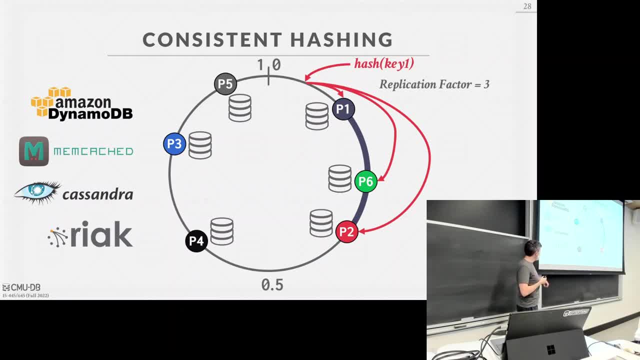 So Facebook never used Cassandra, even though they wrote it. Then a bunch of other people picked it up And then React is a, is or was a distributed key value store. I think it's still around The. the company backing it went under. 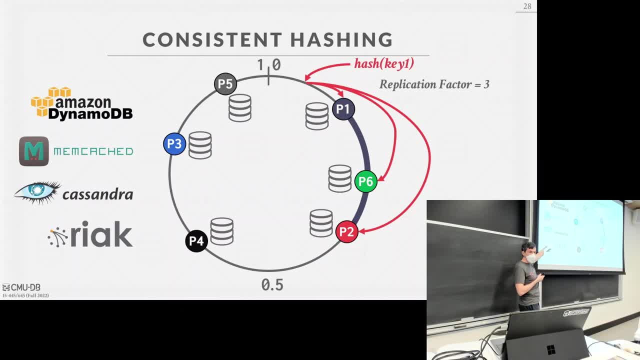 But you can see in their logo they have this, the ring, and they're doing that sort of three, three replication thing I showed before. right, Because it's a, it's a, it's a key value store that's using a consistent. 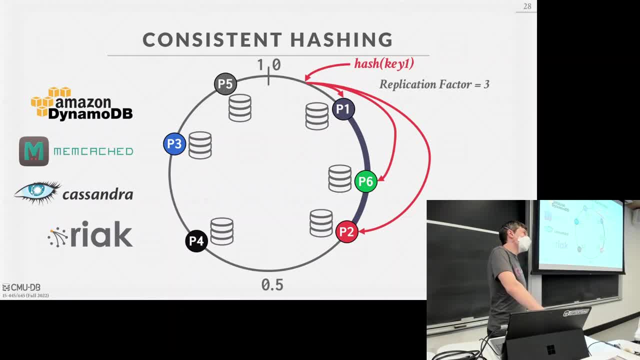 fashion word. So this question: do I mean Dynamo versus DynamoDB? DynamoDB is the public commercial version of Dynamo. They say it's totally different from Dynamo, Right from scratch, or the design From the design. That I'll double check. 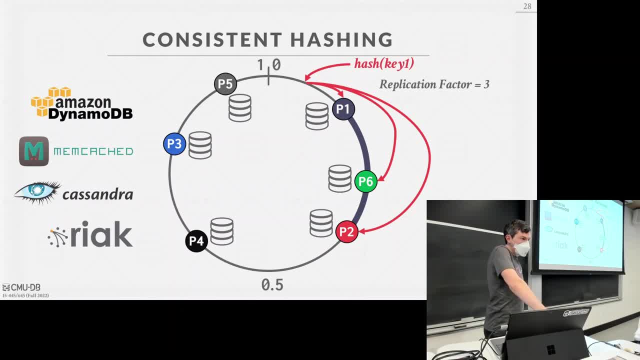 They never have. they just wrote a paper this year about the DynamoDB design, but they didn't talk about consistent fashion word. Okay, I'll double check that. Okay. So yeah, the original Dynamo paper from 2009 does, or 2007 does, this. 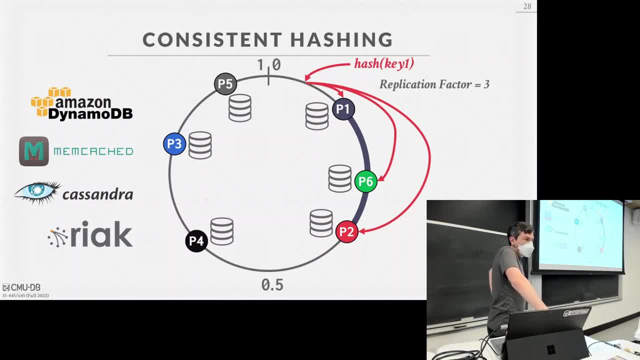 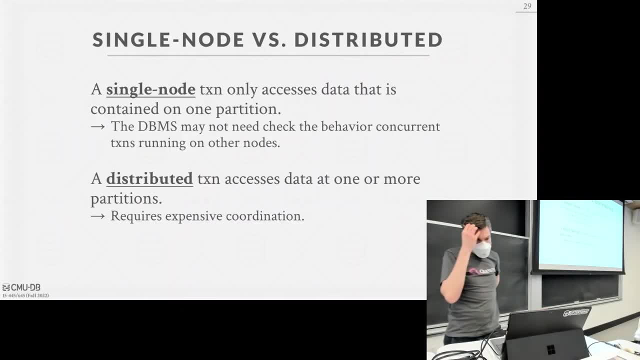 I'll double check that We should cover that in the advanced class. Good, Okay, All right. So so now in this example here, when I said, okay, I do a write, I want to write the data to three locations. 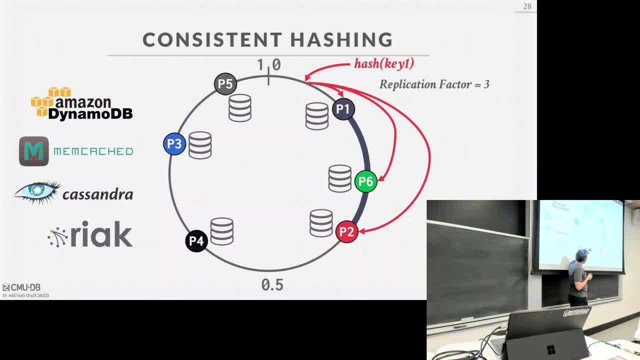 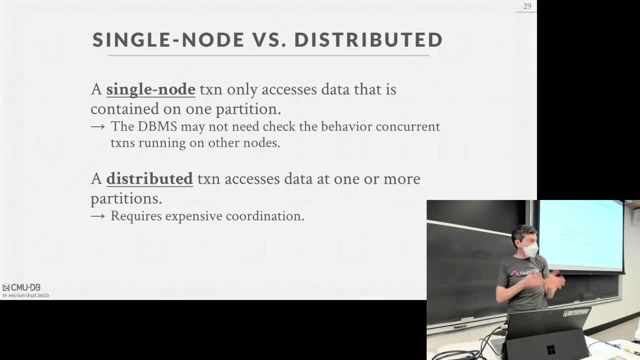 right. This now gets us into the world of how do we make sure that when we do updates, those, those updates get applied to multiple nodes and everything is, it's like, safe and durable, And so so, so, so and so. 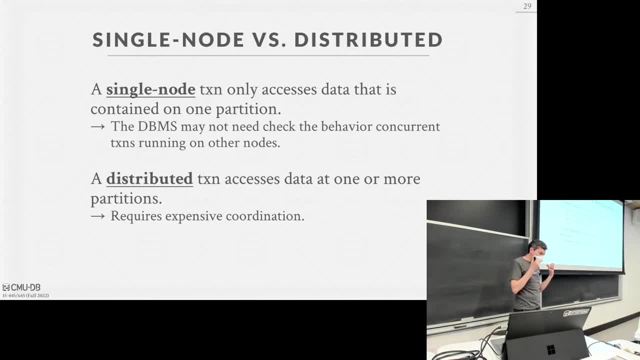 so now we have this notion of a, of a you know what's the sort of the scope of the transaction, meaning how much data or how many nodes we're actually going to have to touch. And again, this doesn't matter. 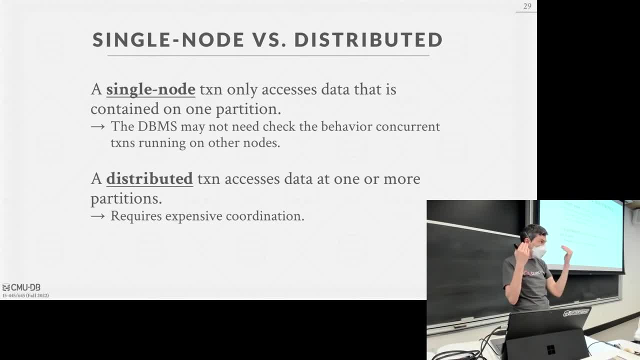 where it's a- whether it's shared disk or shared, nothing if the data is being located or either logically or physically partitioned at different nodes. right, I got to coordinate across them when I do an update, so it happens atomically. So 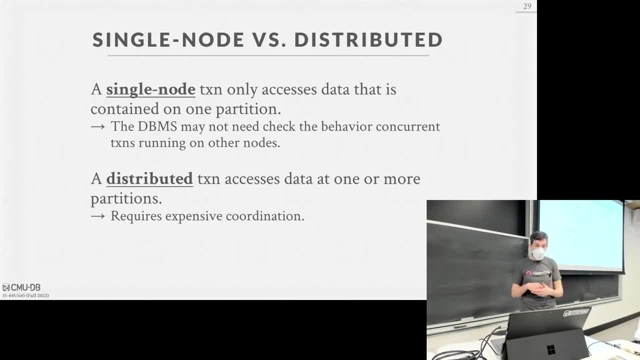 it's obviously, like you know, single partition transaction or single node transaction, and this is the best case scenario because potentially I don't need to coordinate the the commit process of that transaction with other nodes in the system, right, because the data it touches. 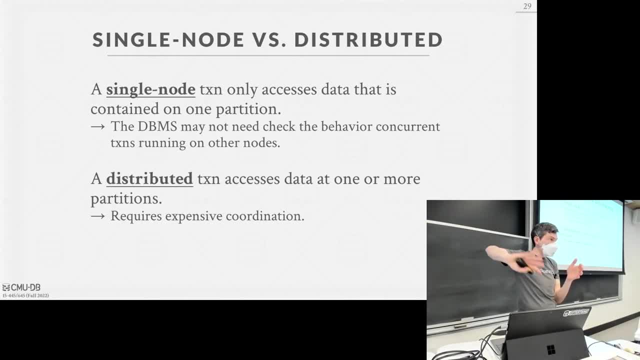 only at that single partition. I don't care what other, what other data, other nodes or what data other transactions running other nodes modify, because they only care about what's local to me. Right, that's the best case scenario and you want to, ideally. 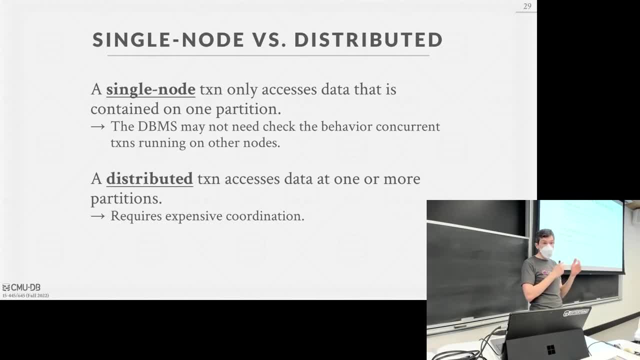 pick a partitioning key if it's an OTP system that maximizes. maximizes the number of single partition or single node transactions and oftentimes you actually can do this right if you think about, like my example of using the customer ID as the partitioning key. 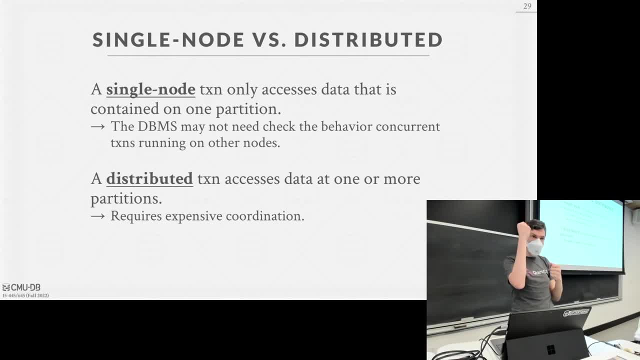 for a table. when you go log into Amazon you can only update things to to to your table or you know your customer record, your your account, right? you're not updating all the people's accounts, so if your data's partitioned, 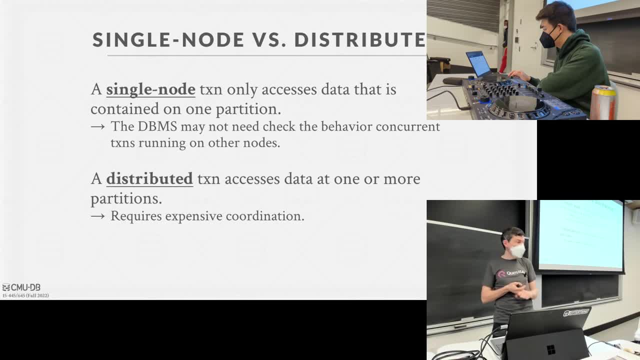 such that all your information is on a single node. you would get a single node transaction. a distributed transaction would be when where the transaction. DJ Mushu, Uh, do I know you? You've been served. Holy, Yeah, I thought. 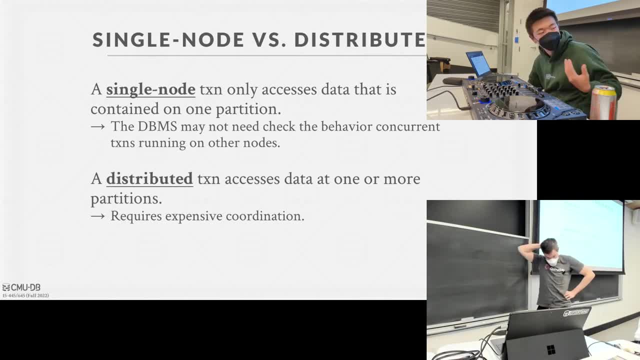 I thought I was in the clear man. Okay, You sure they didn't like reach out to you, They? how did they know I was here? Did you narc on me? I didn't say anything. No, Are you sure? 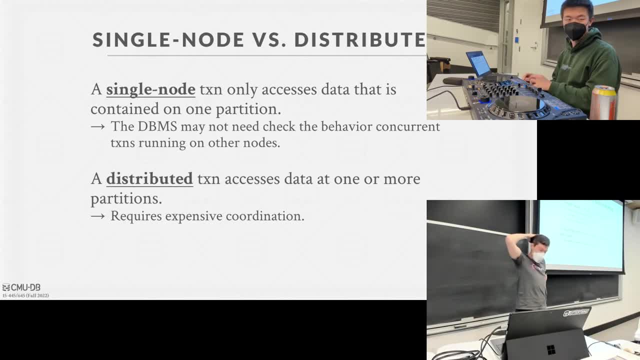 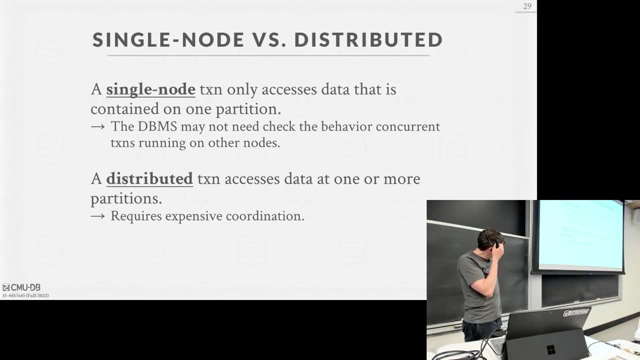 You're not gonna read it. I mean, I'm sure it's just they. they're suing me for child support, but like Okay, All right, uh, yeah, okay, uh, um, all right. Transactions. 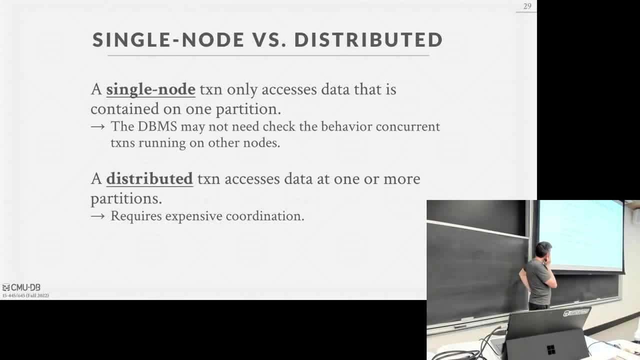 Right, so, uh, again, if, if a transaction has to touch multiple, multiple things, that's multiple things, that's a distributed transaction and that gets very expensive. right, Uh, and we'll, we'll focus on this in the next class. 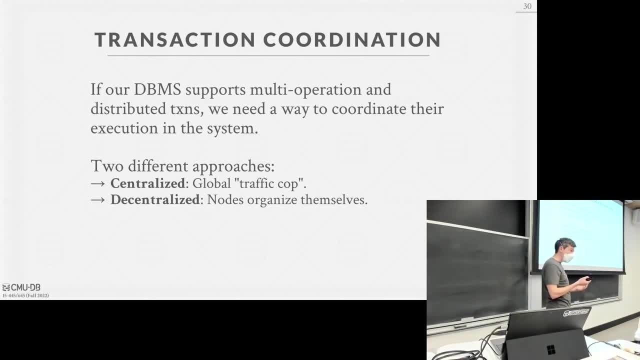 but the the question is now how. who's actually gonna coordinate these transactions Right? Whether it's two-phase commit or sorry, two-phase locking or OCC, it doesn't matter. We still need somebody to say, okay, this transaction is committing. 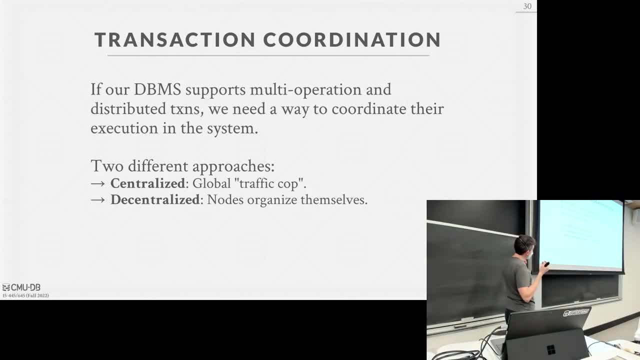 like: let's, let's go ahead and do it. Um and the, the two approaches to have a sort of centralized uh between the nodes themselves. Um, the, the centralized one. it probably is historically more common. Um. 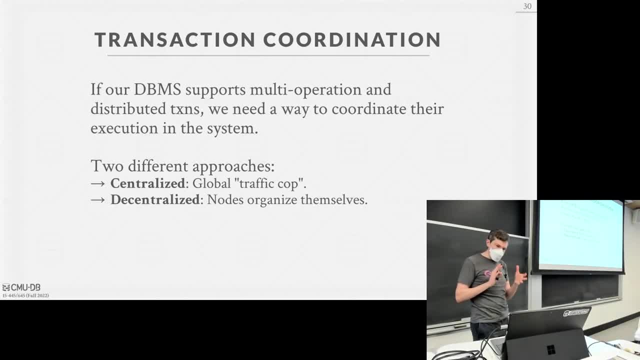 it's again. things get blurry because, uh, the way, the way these, these systems sort of work now is it's a decentralized coordination, but they run a leader election, like Paxos or RAF, to say who is actually the coordinator. 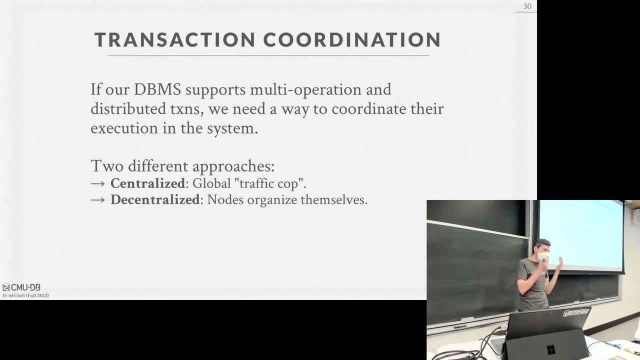 So it is become, essentially becomes centralized, but in theory, if that leader crashes and goes down, you elect a new leader. So it's not a clean dichotomy, but but it's a clean dichotomy, but it's. 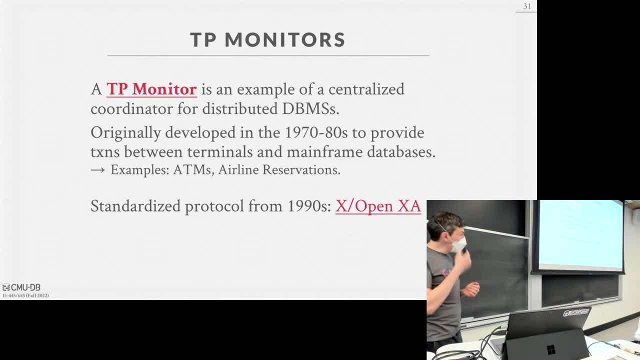 I want to cover both ideas, All right. So, so a centralized uh coordinator, uh, the. the first version of this was was, or typically called TP monitors. Um, TP would some. now it stands for transaction processing. 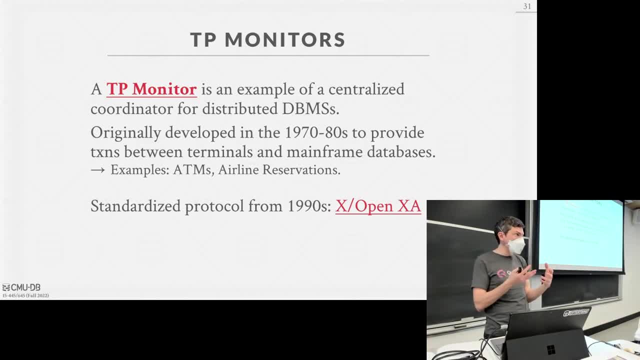 In the old days I think it sounds it stands for the telecom processing, because they they would build these, these sort of centralized transaction coordinators for distributed databases to manage things like people calling on the phone, uh, keeping track of call records. 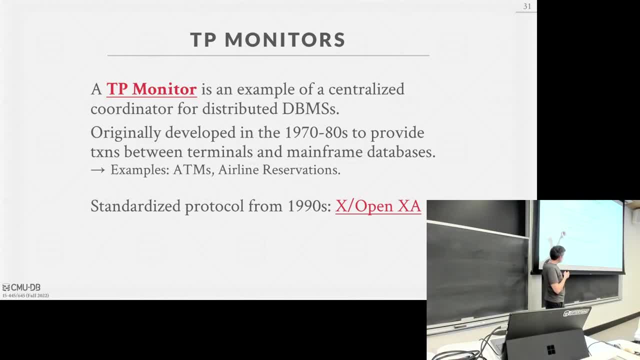 or like ATM machines or whatever right. So they built these early TP monitors back in the 1970s and and like the idea was, you had these single node databases that could do transactions locally on the data that it had right, Similar to what you're building. 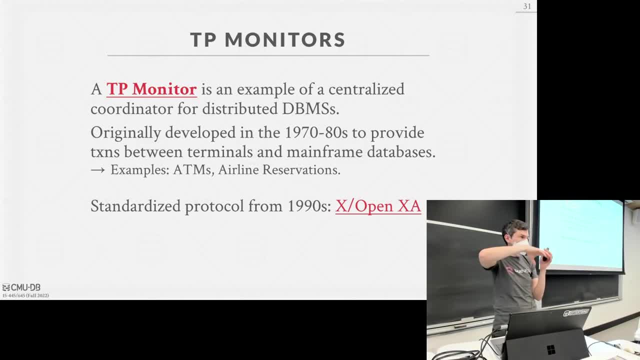 in bus tub. But now, if I want to touch multiple, multiple database systems and run transactions across all of them at the same time, I need this like centralized coordinator. I just sort of sort of you know, be a god above them. 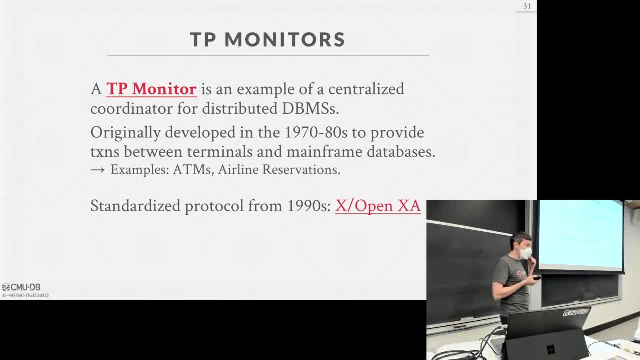 and decide who can do what, And so they built these in the 1970s. A lot of these things are still around today. I think American Airlines- they built a system called Sabre that uses uh TP monitor. that they're. 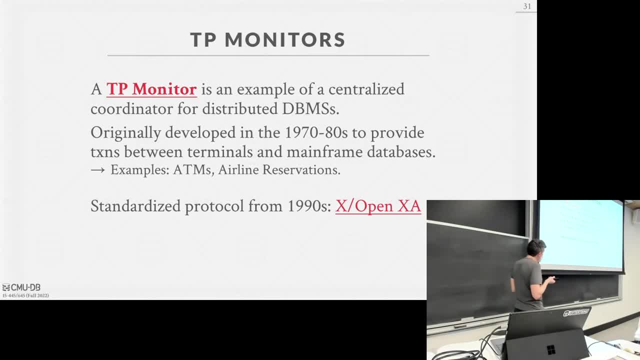 they still use today, uh to to coordinate airline reservations. right In the 1990s there was an attempt to standardize the, the sort of the protocol for committing transactions between uh, these different nodes, um, and called XA. 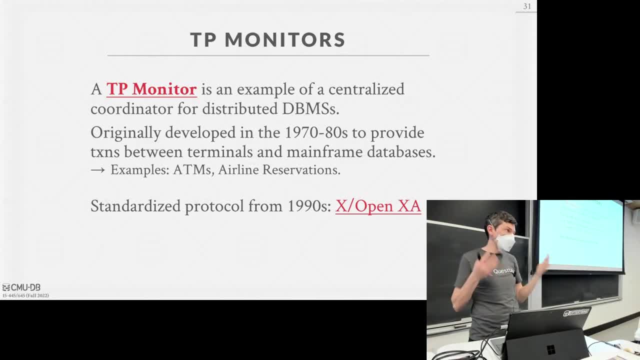 or XOpen- Uh, you few newer systems don't support this. but like the enterprise systems, you can take a single node Oracle database, have multiple ones running at the same time, use a TP monitor and they can. they can coordinate with each other. 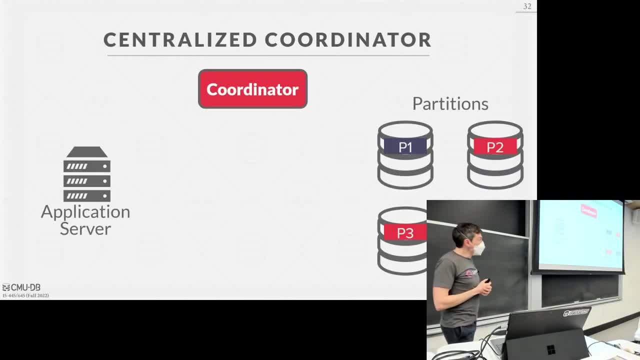 using this, this TP monitor over the XA protocol. So the idea looks like this: right, So we have an application server. So before it's allowed to go touch data on any partition, uh and say it wants to touch, touch partitions one and three. 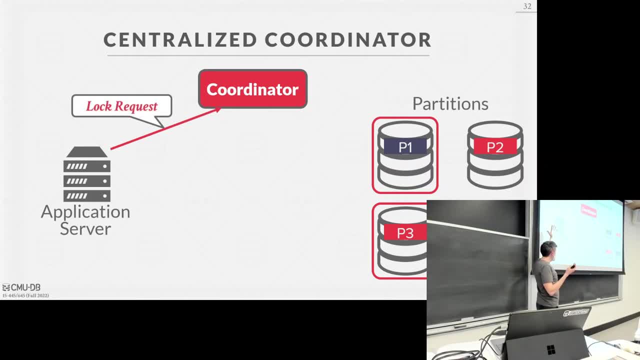 uh, it has to go to this coordinator and say: I'm gonna need this data at these partitions, Let me go ahead and lock them right. And then the coordinator has the: the guys are building project four that- and keep track of. 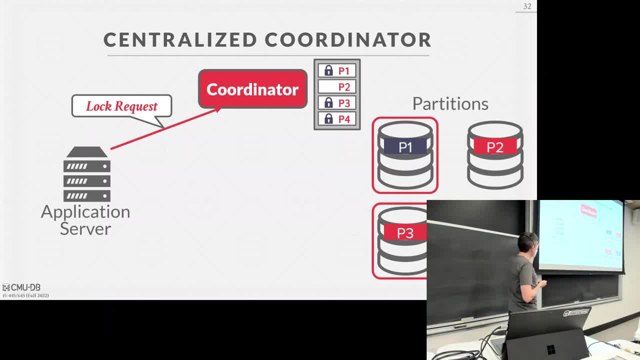 who holds the lock for for what data? Um, so it gets you know, makes the lock request, and once it granted the lock, then it gets acknowledgement, Then it goes. the application server can then go out to, uh, the different nodes. 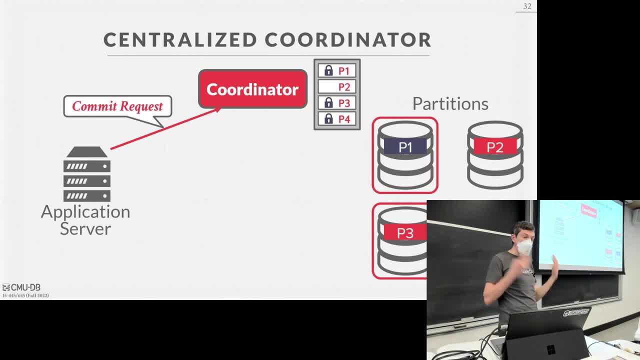 and do whatever it needs to do to to run the queries, do the updates, But now, when it wants to commit, it goes back to the coordinator and says, hey, I wanna, I wanna commit. The coordinator knows how to talk to the different nodes. 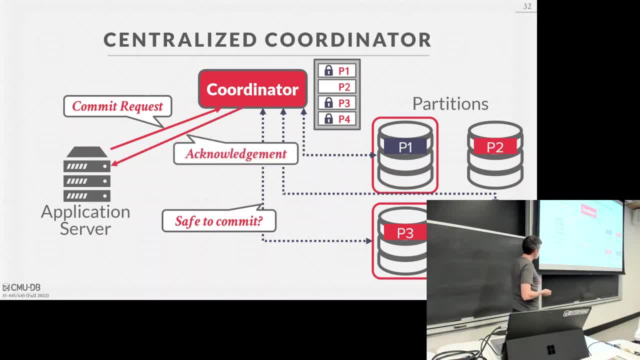 and uh, and if yes, then it'll do the commit and and get the acknowledgement back. Now, what this wire protocol, this part here like how do we say it's safe to commit, get everyone to agree and then commit? 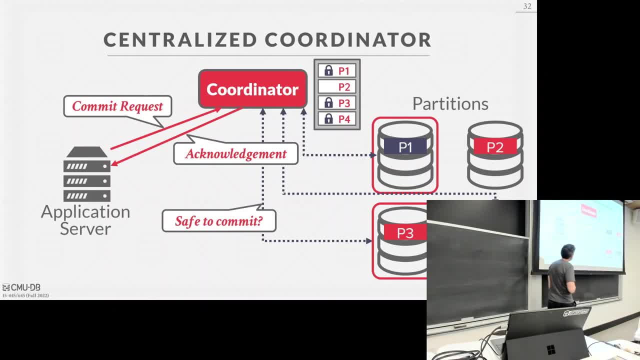 that's Paxos Raft or TPA's commit, which we'll cover next class, All right, So this TP monitor there's, there's, there's a bunch of older systems out there. that, uh, that that. 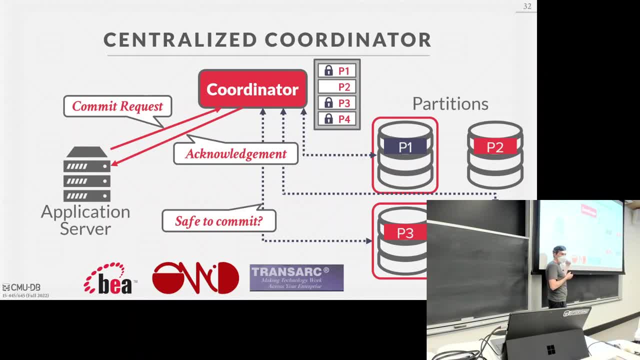 that that do this. BA had this thing called Tuxedo that they bought from AT&T because they built one of these first ones in the 1980s, and then Oracle bought them and it's you can still get Tuxedo today. 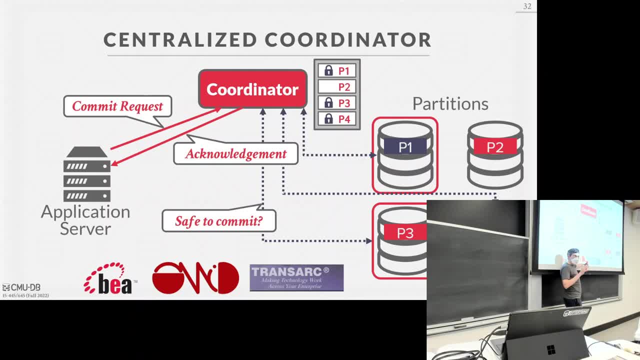 Um, Transarc actually came out of CMU, uh came out with the AFS project. It was like a TP monitor for doing transactions and then IBM bought them. uh, late 90s, early 2000s, Uh. 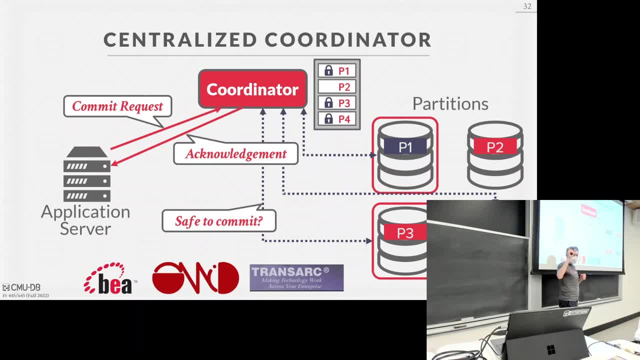 if you, if you, if you're an ISR, whatever the, the software engineering department is called. now there's a guy, Jeff Eppinger. he was the, he was the, he was the CEO of Tuxedo a couple of years ago. 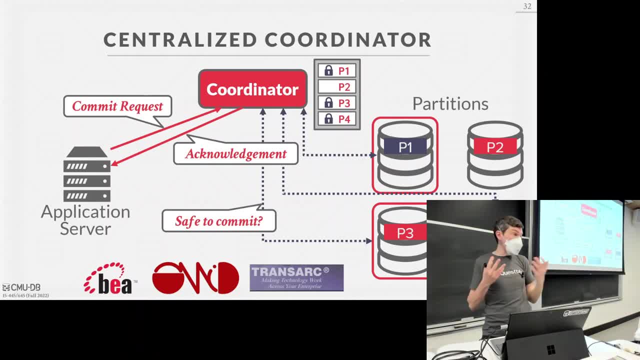 but this is OMID. Uh, this is a TP monitor or a transaction coordinator for uh for HBase. um, that came out of Yahoo Labs and it's an open source project- Apache project that I think is still available today. 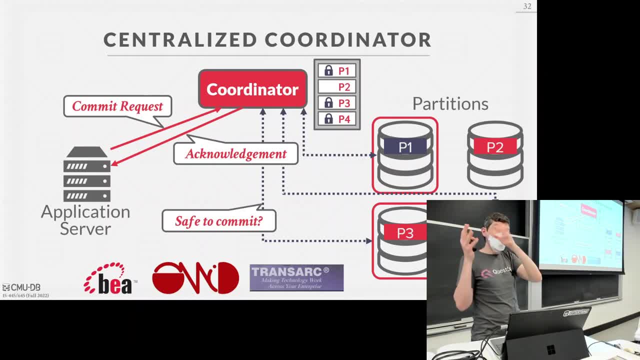 Right. So again, the idea here is that the there's this coordinator on the side. the application has to know that there's a coordinator. it has to go to the coordinator and say, hey, can I do something? The coordinator says yes or no. 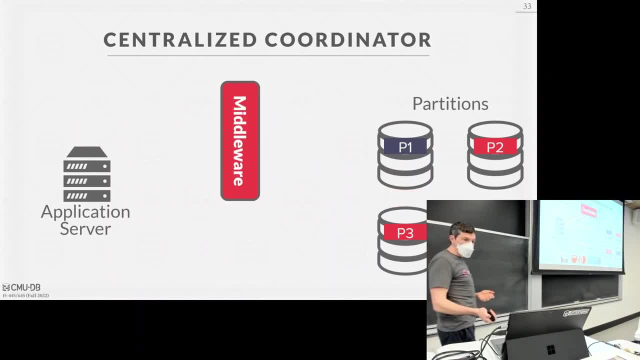 and then you then send your request directly to, directly to the partitions, and what is more common is to have a middleware as a centralized coordinator, where the application doesn't know about the partitions, doesn't know about these nodes. it always sends a request. 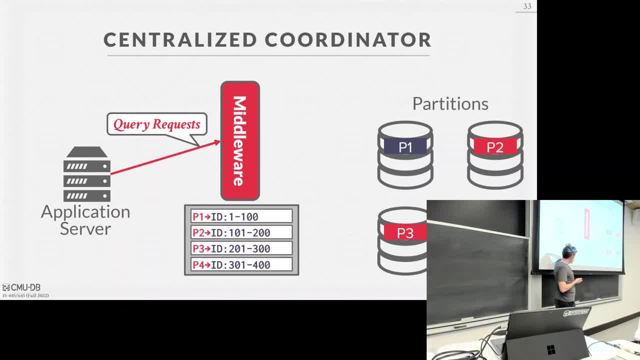 to the middleware and the, the. it has its own block tables and management and everything, and then it can just send the request to uh, the different nodes as as needed Right, And then once, once it wants to go to commit. 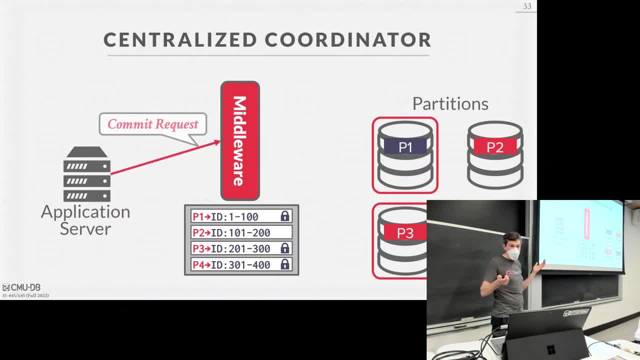 you go to, you ask the coordinator or the middleware: can I commit and then, like before, it goes and asks the different nodes? am I allowed to do this? So right And again, the the. the advantage of this one is that the 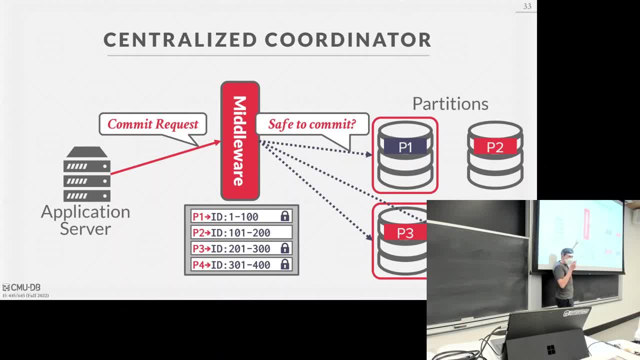 this handles the query routing. this handles the transactions right. The application doesn't need to know what's what's behind it. So there's a bunch of open source systems that do this. The test came out of YouTube, uh. 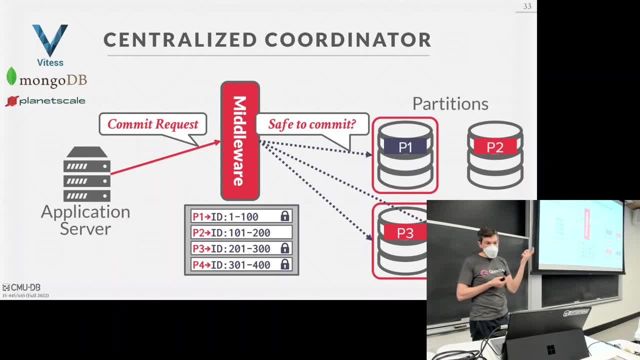 to to basically a middleware in front of uh MySQL, and they do this now uh planet scale, then then commercialize this. I should have showed the example of MongoDB. They work sort of this way. They started MySQL. This is what Facebook does now. 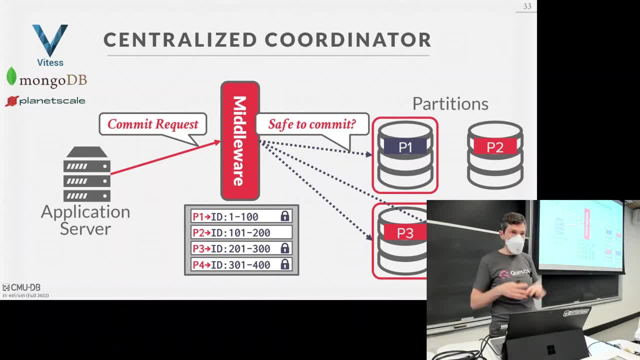 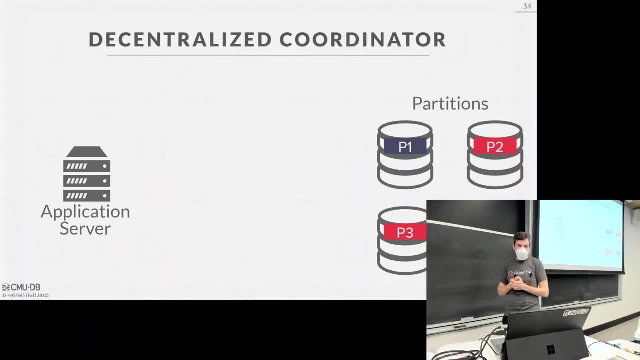 with MySQL. eBay did this with Oracle- right, There's a. there's a bunch of people that that that do this, right. Okay, The one that's sort of again more common, or again it blurs the line. 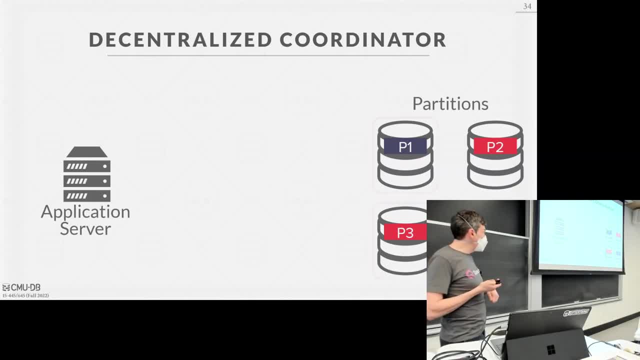 between a middleware and and or a centralized coordinator and decentralized coordinator. uh, for decentralized coordination, the idea is that the, the application server, will right some node in our cluster. This guy then gets anointed as the leader and it's responsible. 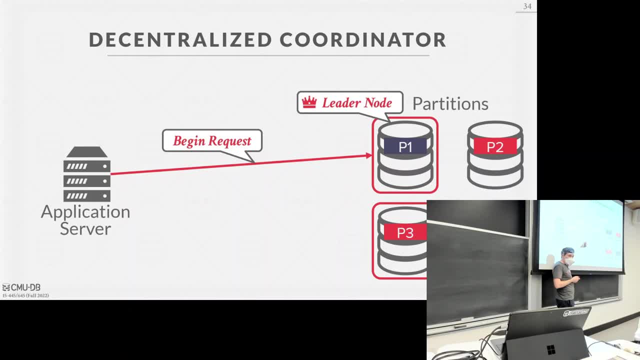 for determining whether this transaction is allowed to commit or not. and if it doesn't, it's not allowed to commit, to tell everyone that they have to roll back and make sure everyone is in agreement that this thing has to commit or not. So now the application. 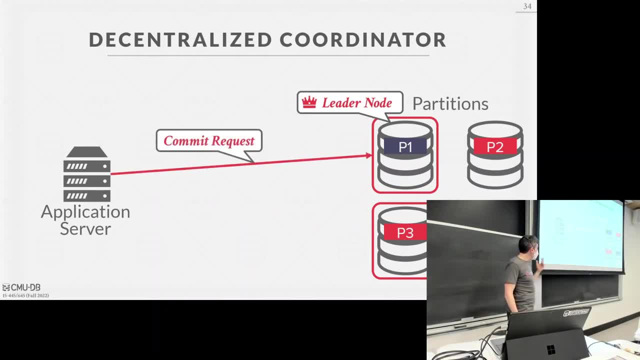 could send query requests into individual partitions, or it could go through the leader, It doesn't matter. But then again, when it goes to commit, it asks the leader: can I do this? They all have to agree. and then then you send back the deposit. 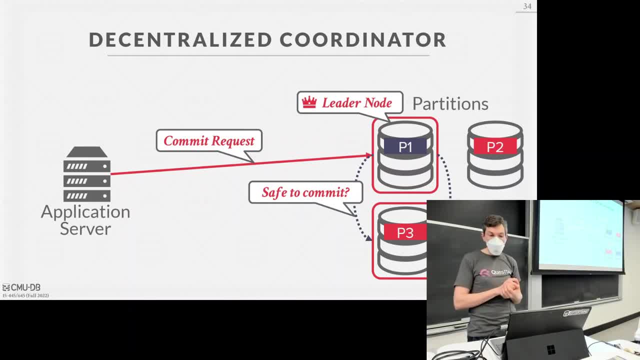 Again, we'll. we'll discuss next class what that, uh, what that protocol actually is. Yes, So the leader can be any of the nodes, or is that? This question is: can the leader be any any node? Uh, in theory. 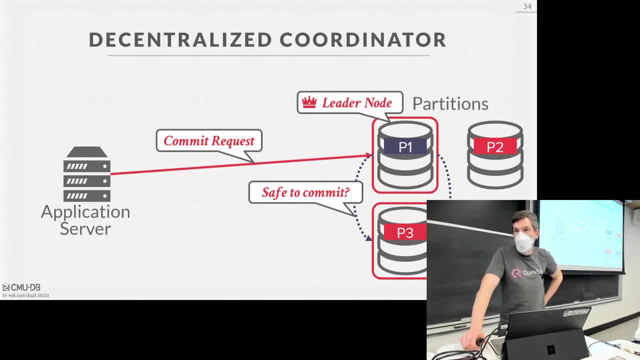 it could be anyone. Yes, But when I'm, when you're, I feel like when I'm using like something like you know, Redshift or so you didn't have one. Yes, There's only one. Is that considered? 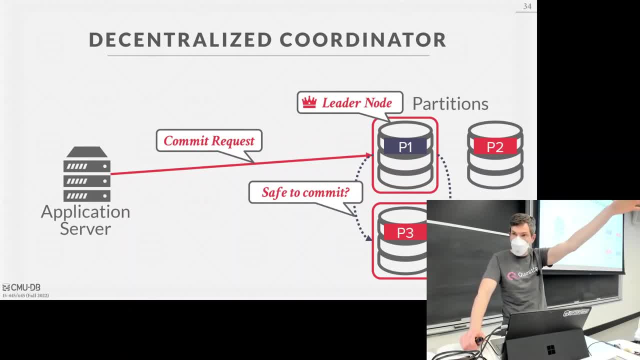 right, And then it for for for dispatching them to the different things. Right, That's the middleware approach. Oh, okay, Yeah, But then? but isn't this what you're saying? how like I'm confused. 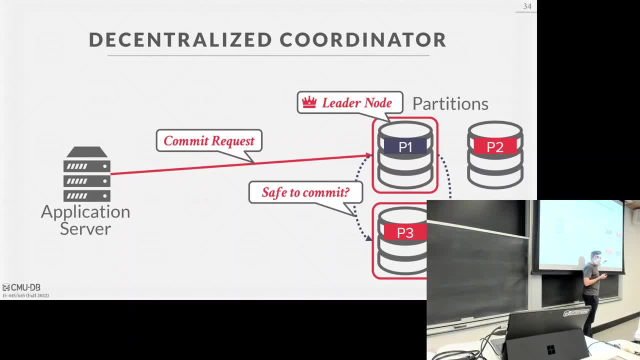 how is this decentralized? I guess How is this decentralized? Because another transaction could be sending, could start a transaction at P3. The P3 is the leader for that transaction. Oh, okay, okay, But now you gotta deal with like. 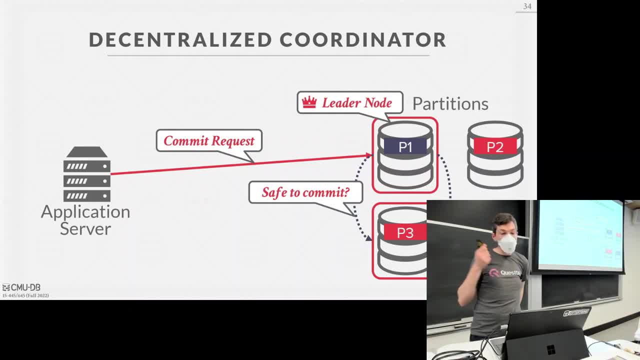 leader election per transaction. See his question is: do you run leader election per transaction? No, you would run like you would have leases, Because otherwise if you're running Paxos leader election, then committing your transaction it's kind of redundant. 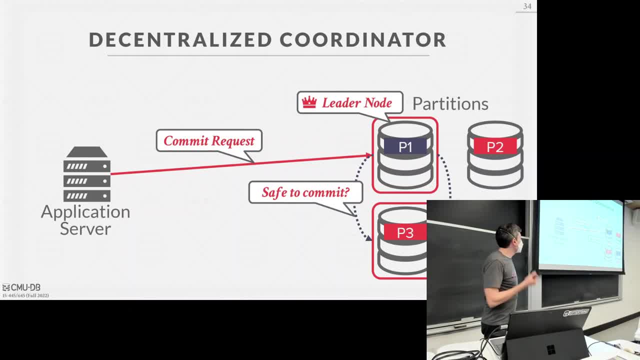 It's wasteful. Yes, Does each partition do their own concurrency control or the leader, the coordinator? Yes. So his statement is: does each transaction do its own concurrency control or does the leader do it for you? So I could have two transactions. 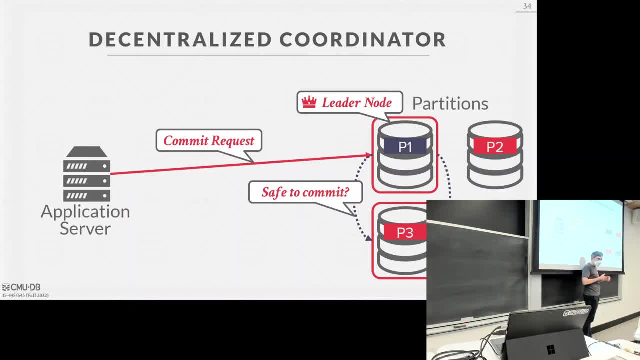 hit up P3 and whatever you want locally as well. right, It's just you need to be aware of, okay? well, like somebody else is also updating data to this thing at this node here And their leader's up above. 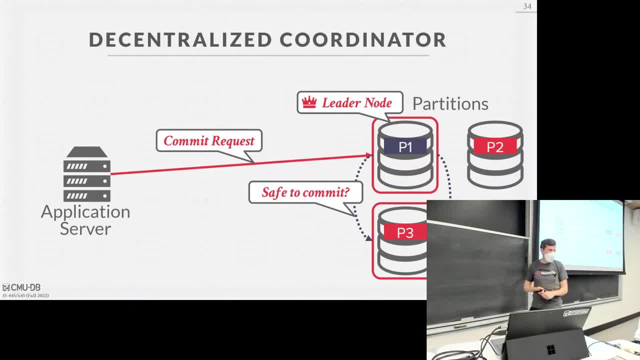 So I need to make sure I'm aware of that. But if you're using centralized coordinator, you can let the centralized coordinator do the concurrency. Yeah, same If I'm doing centralized coordinator, since everything goes through the, at least the middleware. 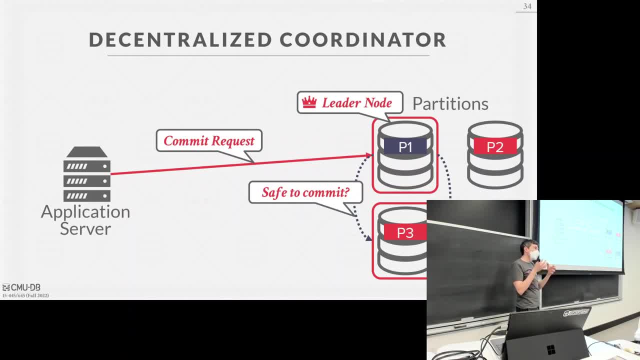 if everything goes through the middleware, the middleware it depends. It could be like I have locks on a portion of the partition and then for individual like tuple level locks, you still do that locally right. So again, this is like. 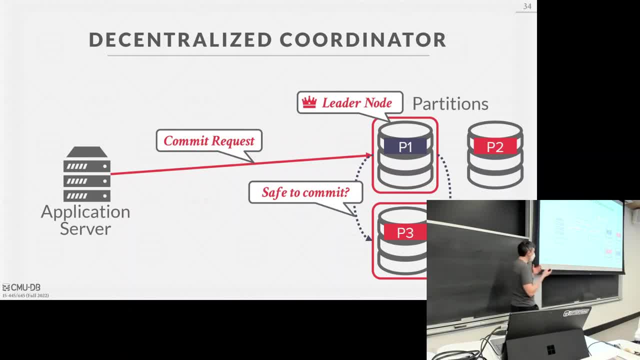 it's two-phase locking distributed, but then also on the local node you do two-phase locking as well, And the reason why you have to ask whether it's safe to commit because you could be sending query. you're sending SQL requests over. 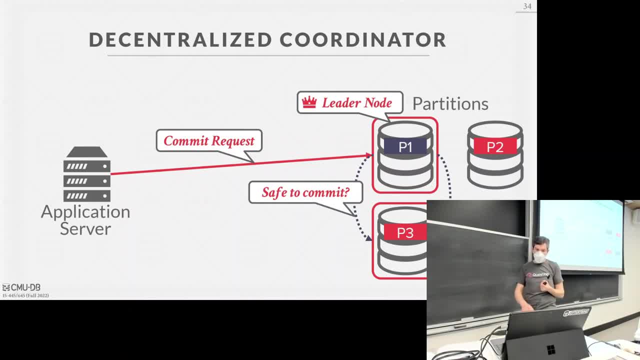 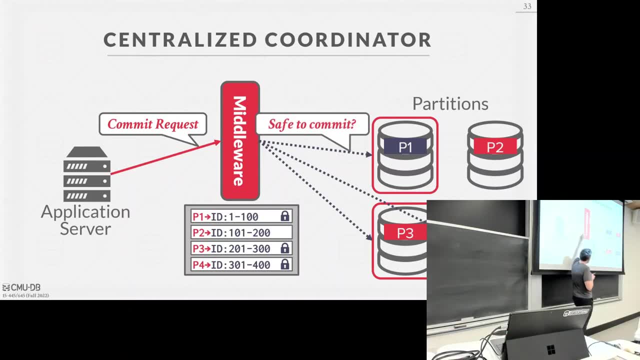 just go back. let me go back to the centralized one because I think it's a little bit harder. Like the application could have sent SQL requests over The middleware says, well, I know how to route it to the location that has the data. 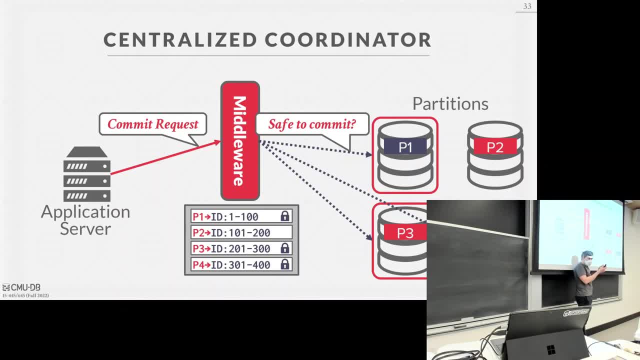 you want. but I don't actually know what you did right, Because it's like you look at the where clause but in like the set clause. if it's an update, it might do something like set somebody's. 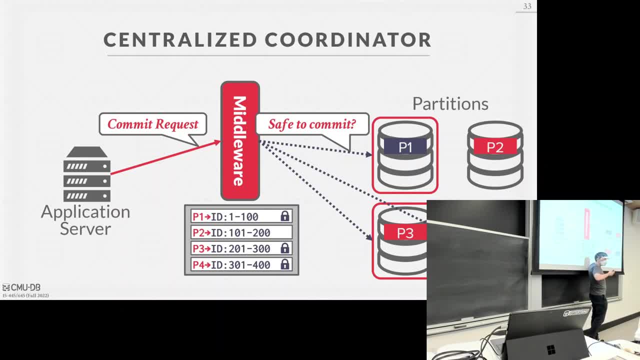 you know age to a negative value, and then there's an integrity constraint that says that's not true, And if it failed, you have to tell everyone else that you failed, And the middleware would handle that for you. Okay, All right. 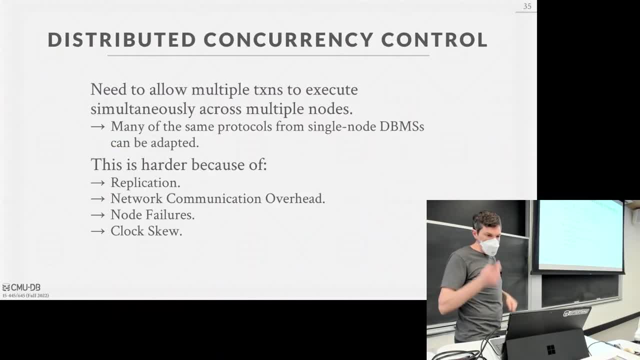 So the last thing I said I wanted to cover is distributed currency control, and I've been alluding to all this, and this will be what we'll talk about next week. Ideally, we want to have multiple transactions be able to execute simultaneously across different nodes. 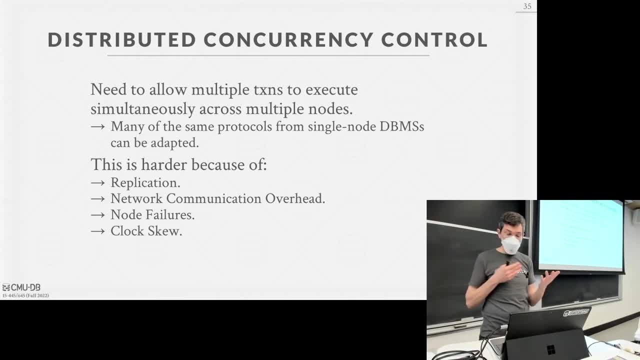 at the same time. It doesn't matter whether it's shared or shared, nothing right. We want to be able to handle this, And so we need to make sure now we want to have all the same asset guarantees that we spent the last three weeks. 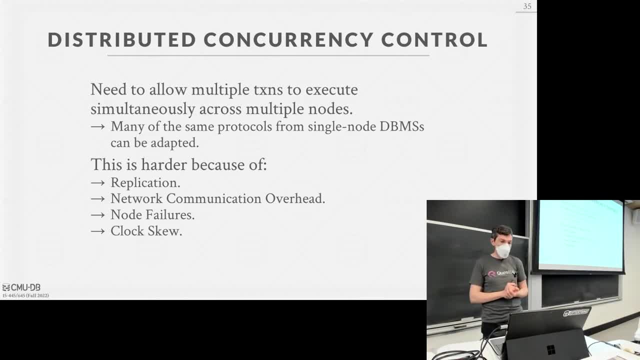 talking about for our single node database, We want them to carry over to our distributed database, right? Of course, this is going to be a lot harder, as I said before, because now we've got to worry about the network, the cost of sending, 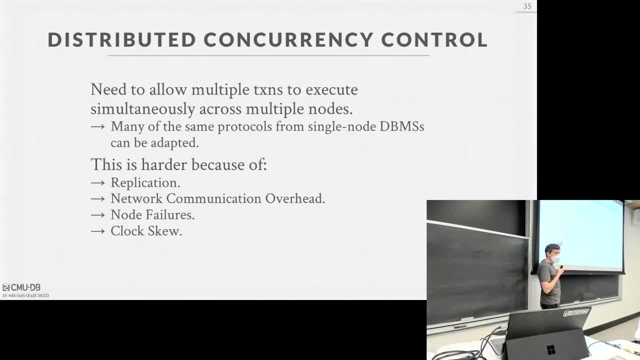 messages, messages not arriving at all. We have to deal with machines going down and crashing If we're using like clocks for the timestamps, if we're doing timestamp ordering or even multiversioning or using the timestamp to keep track of who started first. 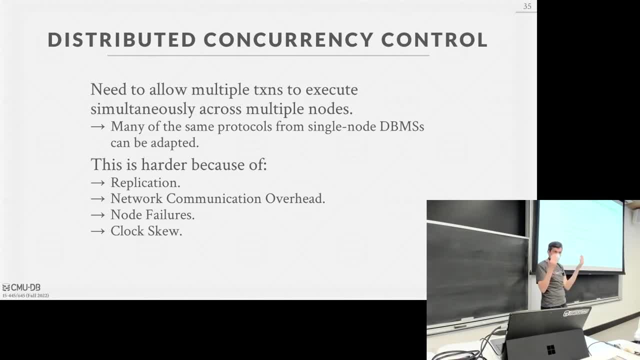 versus another. how do I actually keep the clock in sync with different nodes running at the same time? That's super hard, right? And then we'll talk about also now, since I want to have high availability. I don't want it to be. 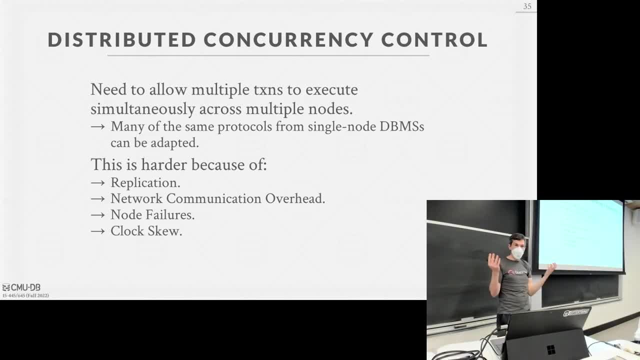 the case where if one node goes down, my whole database goes down because now I'm missing data. I want to be able to do replication, where I update data. I write data to one node and it gets propagated to other nodes. Shared disk solves. 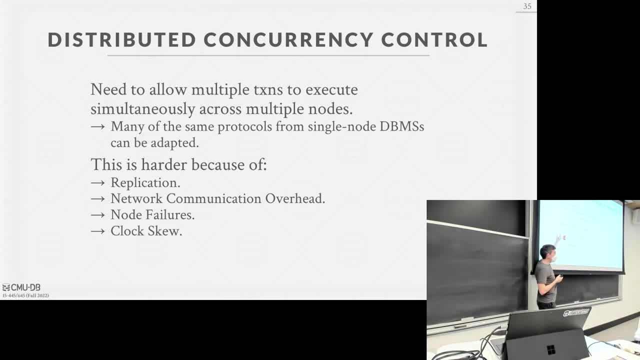 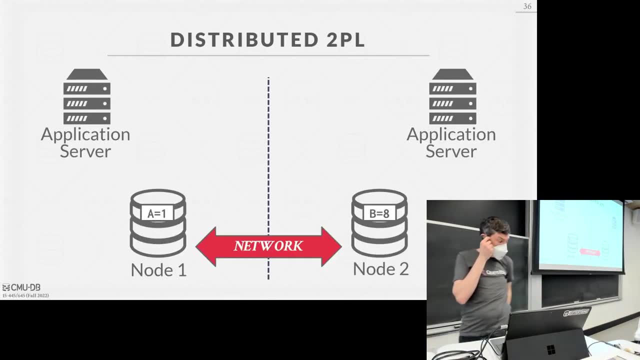 that problem in some ways. but if you don't share nothing, you have to worry about those right. So let's see why this is hard. So say we want to do distributed TPL. We have two nodes that are separated by some network. 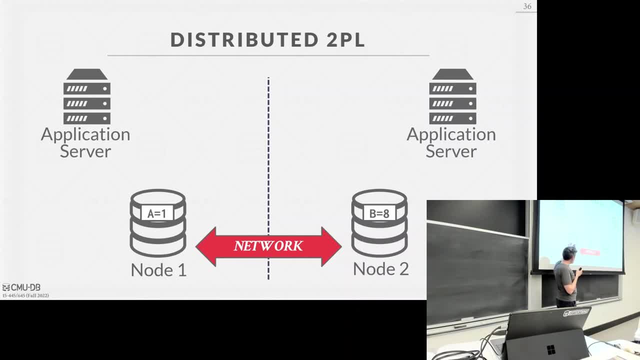 and the node one has a single key A, node two has a single key B. So at exactly the same time these two transactions start running. They don't know about each other at this point. The first guy wants to update A, the second guy wants: 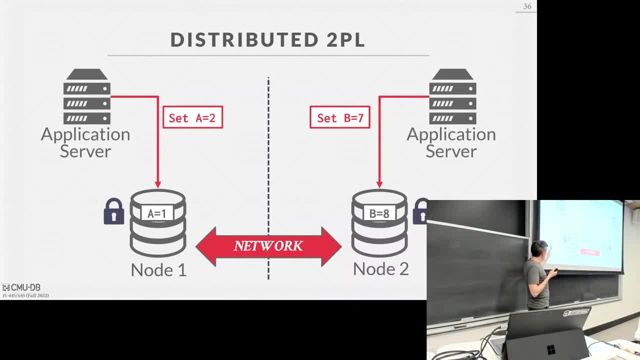 to update B. So we just run a local two-phase locking. no big deal. They both get the exclusive lock on these two objects, right, That's fine. But now they want to. the first guy wants to update B, the other guy. 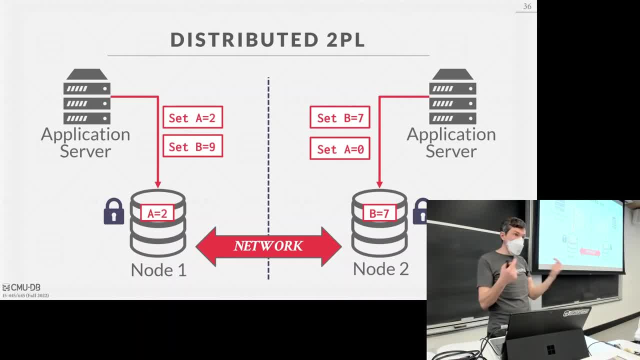 wants to update A, but the system knows that this data is not local, it's on the other node. so it's got to send a lock request over the network back and forth And we have the classic deadlock that we had to deal with from before. 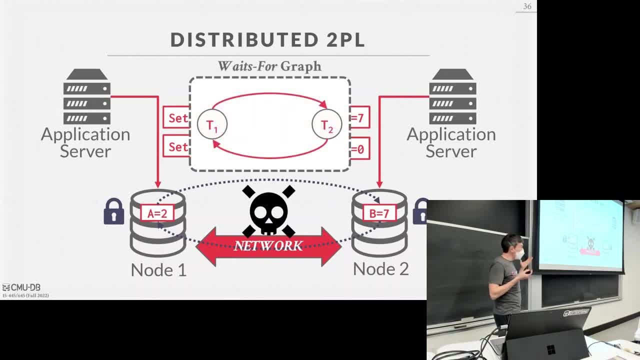 All right, we know how to do deadlock detection, right. This is just a wait for graph right to figure out who's waiting for who and are they, you know, is it never going to get released? But now the problem is I got to send. 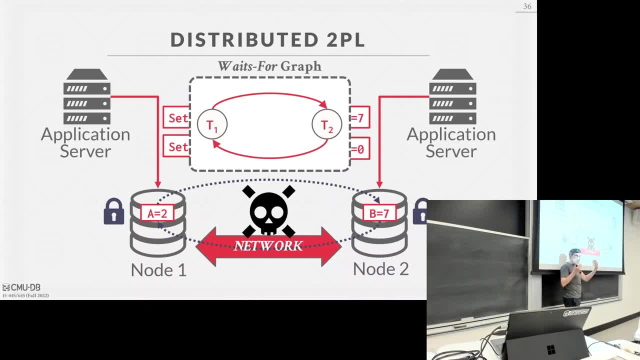 I got to coordinate between these different nodes because they have their own notion of who's waiting for what. Someone's got to run deadlock detection, someone's got to tell somebody who's going to die, But like if say the message gets lost. or say like 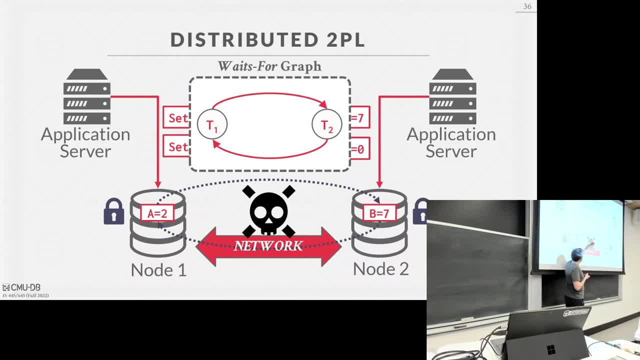 they both try and nothing ever gets done right. it's the same hour that everything's just harder because now the network's unreliable, the network is slow and the state of the system is split across two different, you know- geographical regions, Now the centralized. 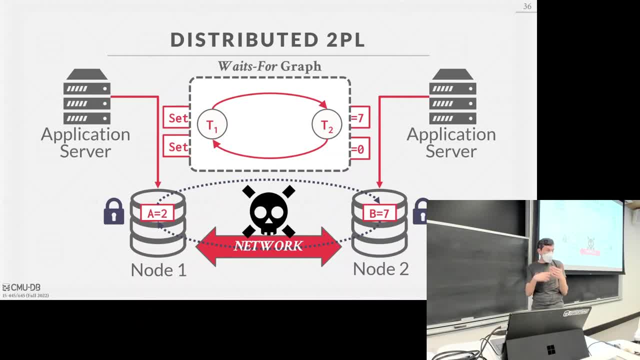 coordinator solves this in some ways, but you still have the problems of, you know, communicating between different nodes and say, hey, are we allowed to do this, yes or no? So, just because you have a centralized coordinator, okay, All right. 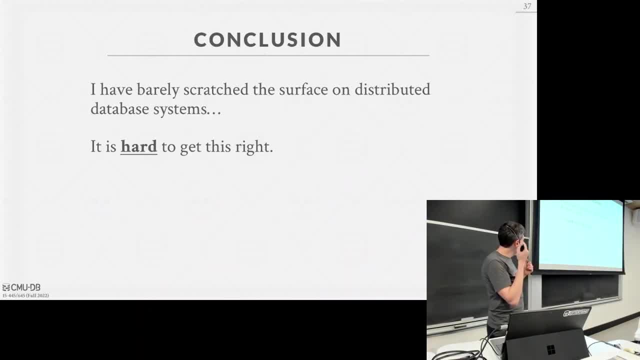 so just to sort of finish up, and then we'll talk about project four. So I barely scratched the surface on distributed database systems. Again, next week will be all about first doing it for OLTP and doing it for OLAP, and as often as I say in this, 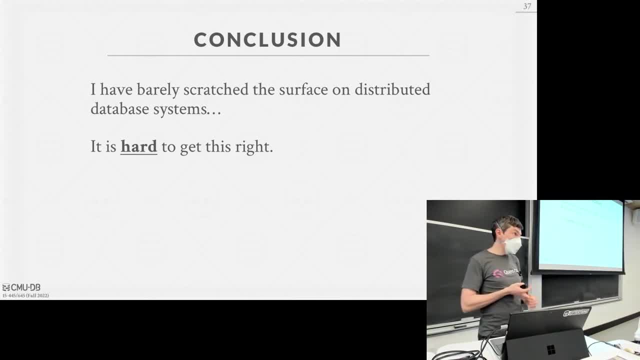 class. it's hard to get this right. This is why you don't want random JavaScript programmers writing their own distributed database, which they often do right. That centralized coordinator thing. people actually build that thing a lot inside their application, Like in their application code. 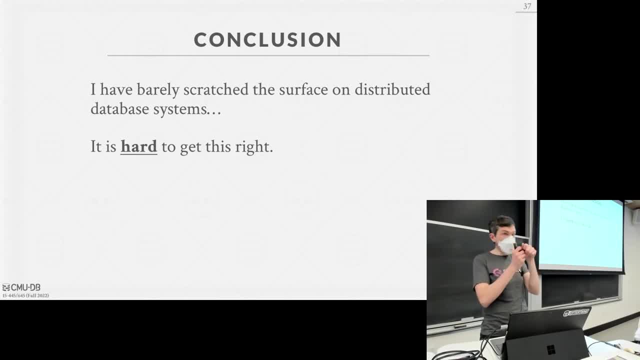 they'll say: okay, well, I hash the thing I'm looking up on and that'll tell me which database connection I go to right. They're basically doing sharding internally in their application. In my opinion, that's a bad idea. 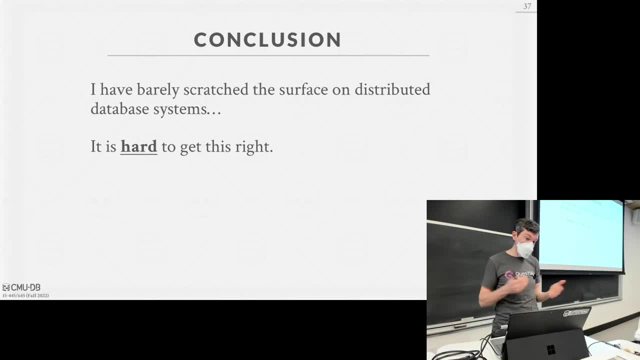 You don't want to do that. You want to use a database system. Most cases, most people, don't need a distributed database at all. Like 99% of the applications out there don't need distributed database. They don't need a sort of 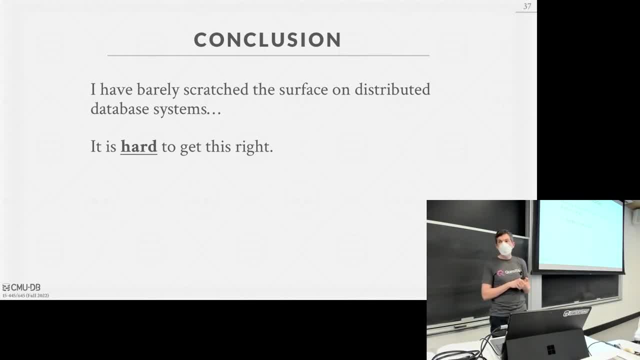 horizontally scale-out distributed database. So this question is: when should you be considering a distributed database? My answer would be: if you're doing a startup and you cannot scale vertically Postgres anymore because you have a lot of data. you have a lot of. 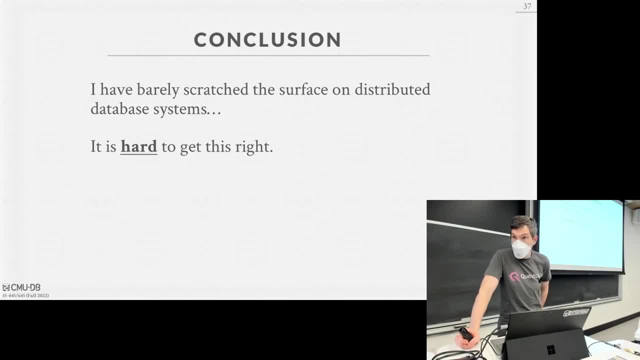 operations, a lot of transactions. at that point you have money and then you pay for that architecture because it's going to be either for me or for him or somebody- Probably him- Somebody come and tell you what to do, But most startups- 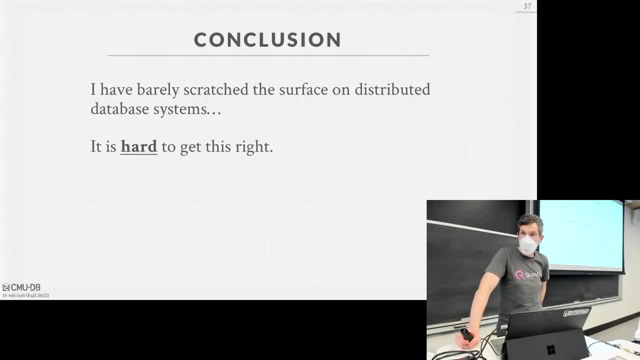 when they start off, can get by with a well-tuned Postgres running on a single box with replication for availability. Most people like the no-SQL stuff. a lot of that came out because people started building these things, because this what Google did. 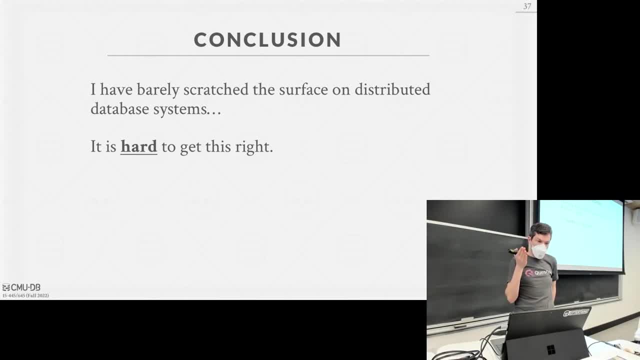 Google was super, is and was. now like a lot of people try to say: oh, google, they're making a lot of money. they have a bunch of scale buddy problems- i'm gonna be the next google. i have the same kind of problems- and they sort of try to make their own versions. 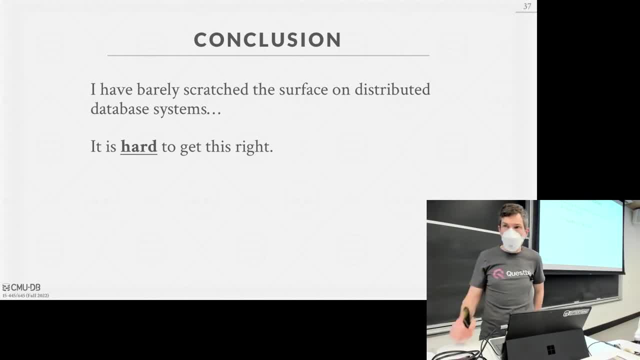 of big table and other things that google was building internally. but a lot of the design stations that google made were right for google but not right for a lot of people. so people were sort of unnecessarily building complex systems that they probably didn't need to- sort of reinventing the wheel for a lot of things. 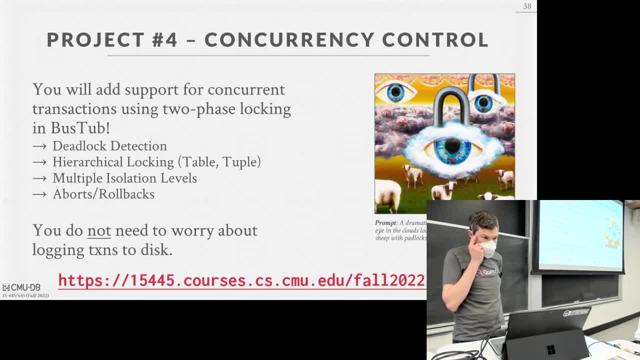 okay, all right, project four, project four, is out, uh, and what you guys will be doing is adding support for transactions, doing two-phase locking in bus top, and so you're going to do deadlock detection, uh, hierarchical locking, just with tables and tuples, no page locks. um, you have to support multiple. 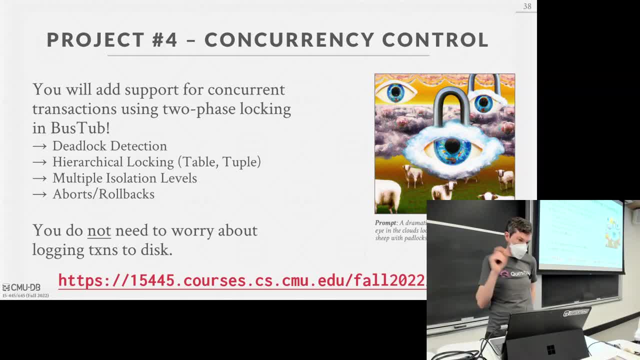 isolation levels. i don't think we require serializability because that requires extra steps. we're not going to do that. um, and you have support transaction rollbacks and aborts or rolling back data because of aborts? okay, so you do not need to worry about doing right ahead logging in. 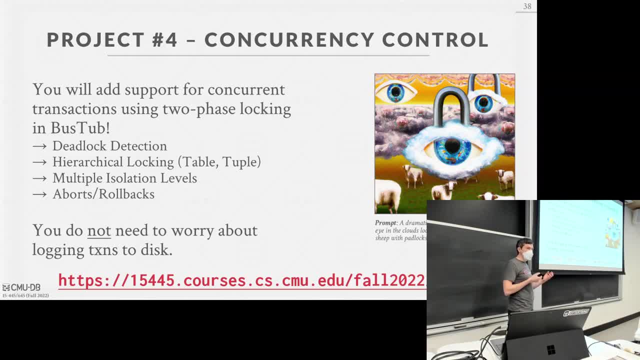 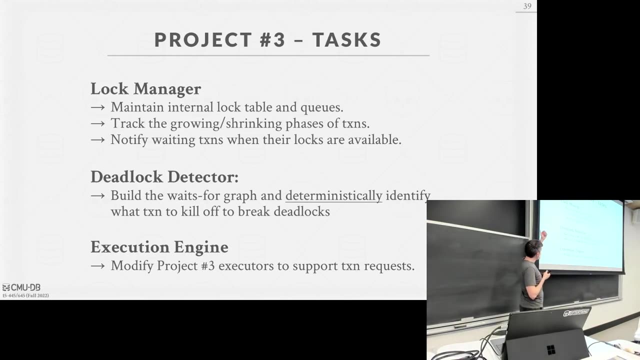 in your, in the system. so we essentially are doing a a and i: atomicity and isolation for your transactions. we're not doing durability, consistency. we don't worry about that as well. okay, so there's three tasks actually project four, not three. the first one, the lock manager. again you're going to maintain the internal. 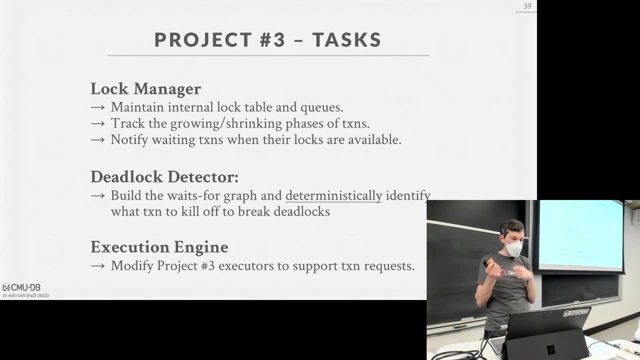 lock table and then and the queues of what transactions are waiting for what locks. uh, you need to keep track of what phase they are in in two-phase locking. and then, when a transactions, the transaction, is waiting for a lock, you need a way to notify the transaction to wake up. 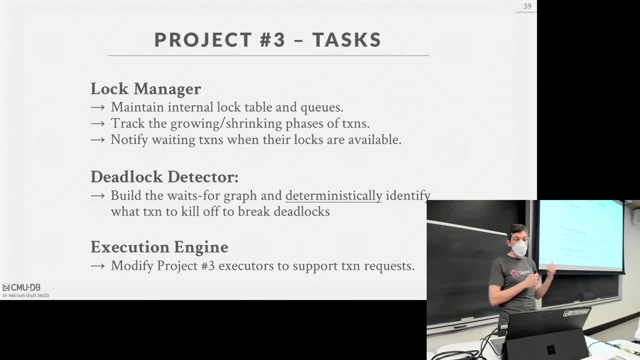 and unblock them and then let them acquire acquire the lock. you also need to support a lock upgrades as well, which i'm missing from this. you have to build a deadlock detector. it's going to maintain its own weights for a graph and then have a deterministic protocol for. 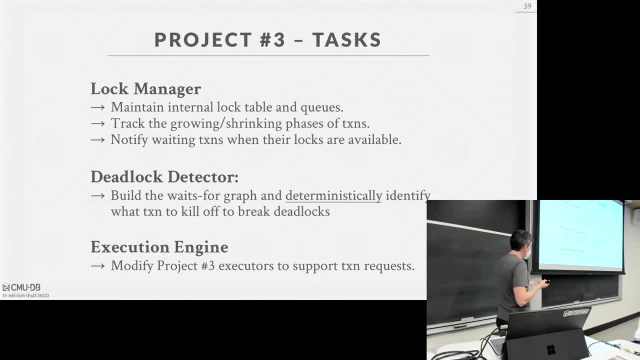 identifying what transactions you want to kill. and i'm underlying the term, the term or the word deterministically, because you want to be the case that for every single, for every sort of arrangement of transactions- who's waiting for who? you want to make sure you kill the the same transaction over and over again. 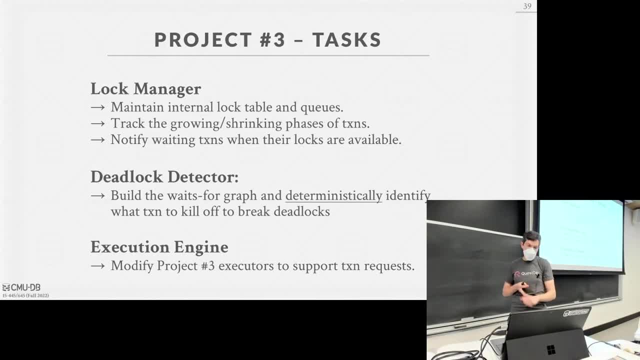 because that's how the test cases will check for things. right, if you're flipping a coin, then it'll unlock something that the test doesn't expect, and then you need to modify your execution engine for project three to uh update like the sequential scan and the index scan. i think the insert uh executor is to now support transactions. 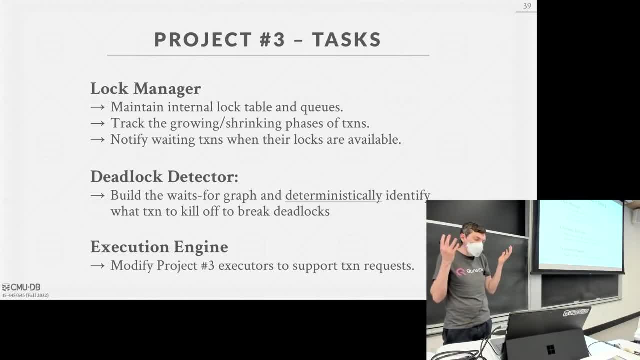 okay, you don't need. you don't need a lock tape, you don't need to lock tuples in your hash. your, your, your nest loop join operator, because you've already scanned the data. at that point, i assume that that the access method below that already already acquired the locks to read the data.